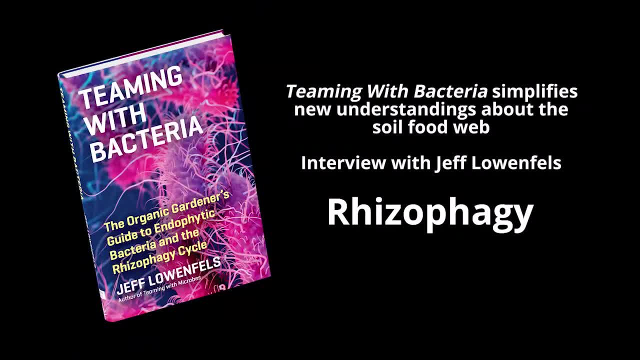 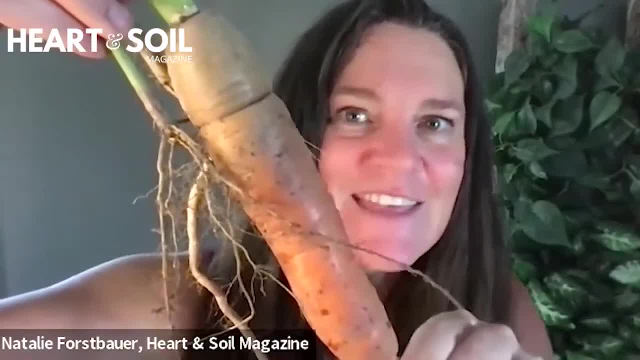 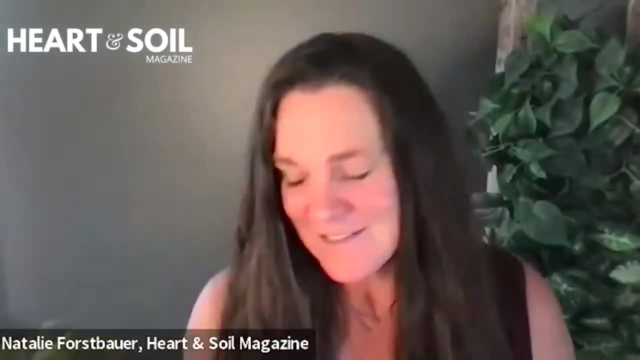 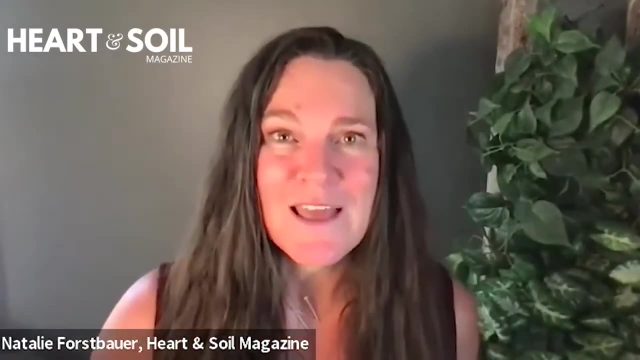 See little hairs on this carrot and on these roots. See all those little hairs. They weren't grown by the plant. In fact, they were grown by bacteria. And Jeff Lowenfels, the author of the book Teeming with Micros and the books Teeming with Nutrients and Teeming with Fungi. 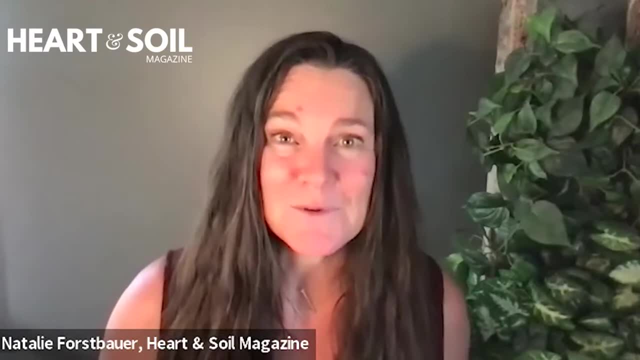 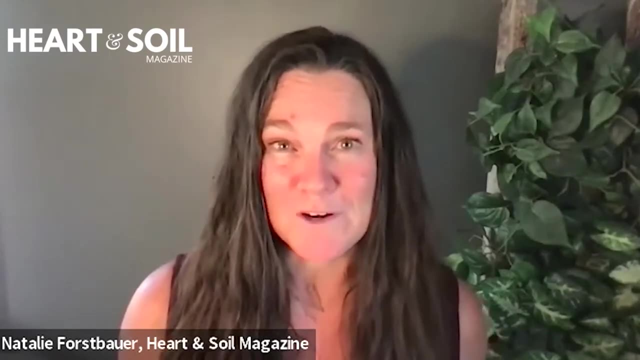 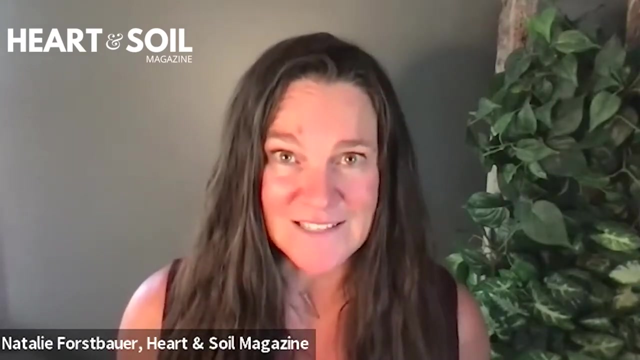 has just released a brand new book called Teeming with Bacteria, And in it he dives into how we've misunderstood how the soil food web works and what we are learning about the important role bacteria plays in growing food and growing plants. It's fascinating. It's exciting And with 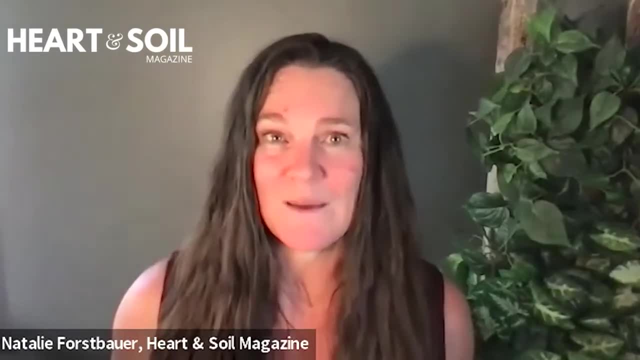 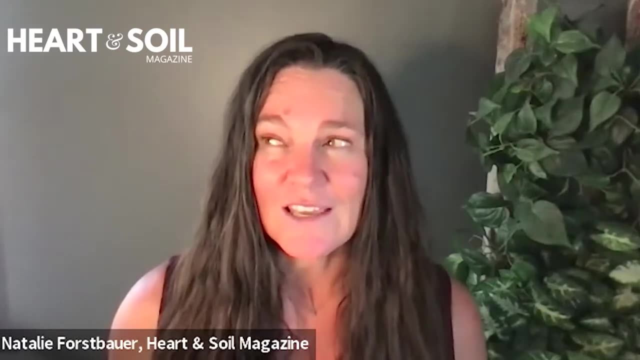 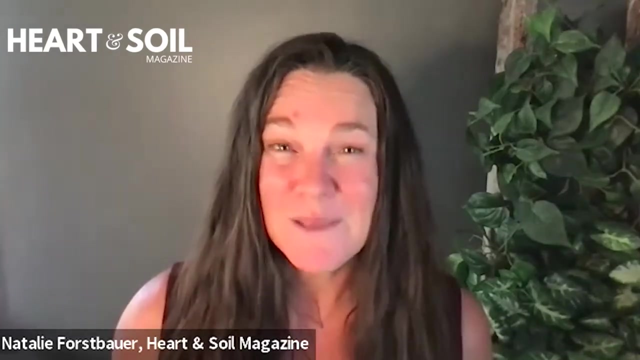 this new knowledge, we can actually move away from using chemicals on our fields and on our crops to make a better world, And so I'm going to share with you a little bit about how we've moved towards looking at how we can use bacteria to feed our plants and how we can use bacteria to 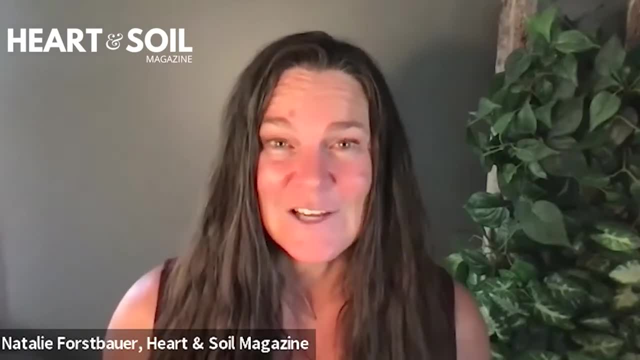 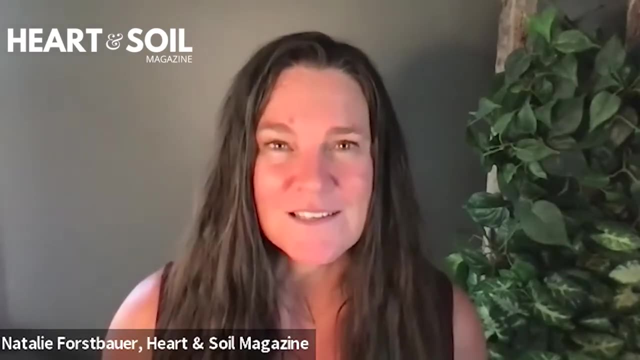 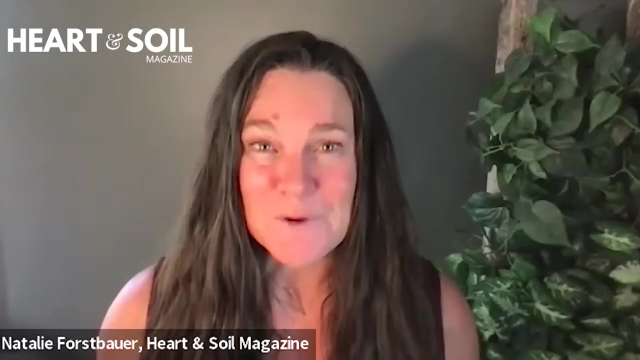 maybe even control weeds. Jeff Lowenfels is a gardener and a writer and a superhuman who amplifies the incredible science that is being discovered around the world about the soil food web and how we can grow food without chemicals and through our plants, So I'm going to share with 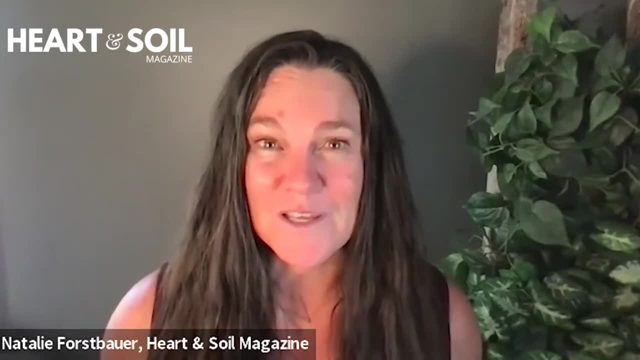 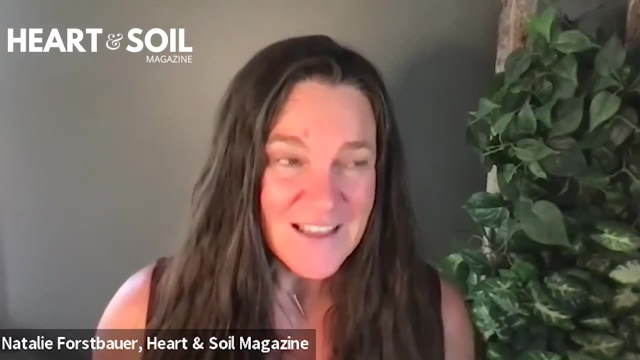 you a little bit about how we've moved towards building soil health and building the soil food web and working with nature instead of against nature, And I'm really excited to share this conversation with you. I'm Natalie Forsbauer, founder and editor-in-chief of Heart and Soil. 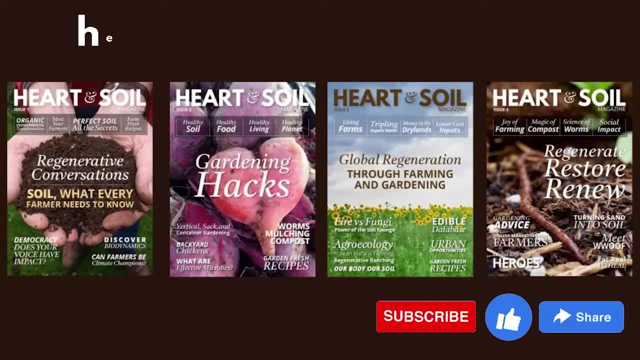 Magazine. If you want a free magazine, head on over to heartandsoilmagazinecom and you can grab a free issue there where you can check it out and see if it's a fit for you. And if you want to subscribe and become part of our community, it's just $39.99 a year. 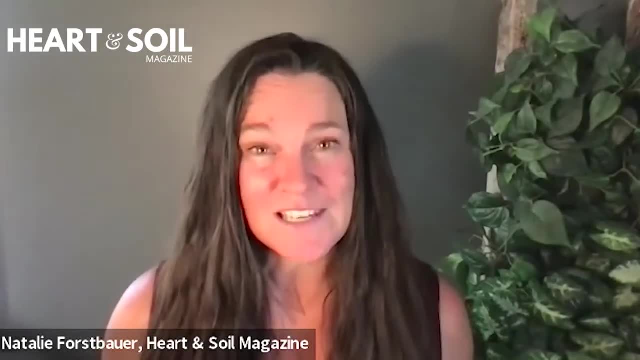 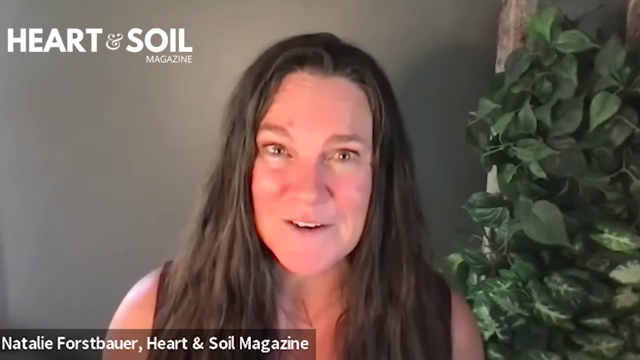 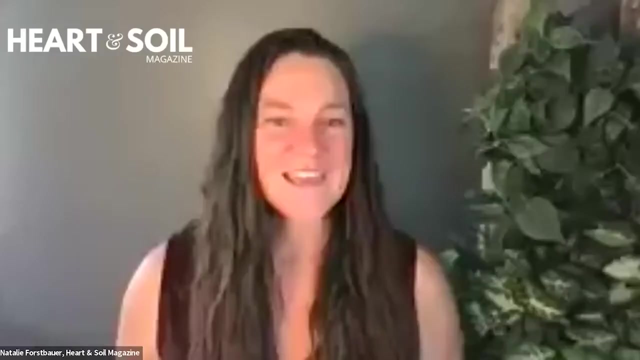 And if you want to subscribe and become part of our community, you get access to all the back issues, plus a bunch of new goodies that we're dropping into the membership area. Enjoy the conversation with Jeff Lowenfels and you make yourself an amazing day. Okay, awesome. 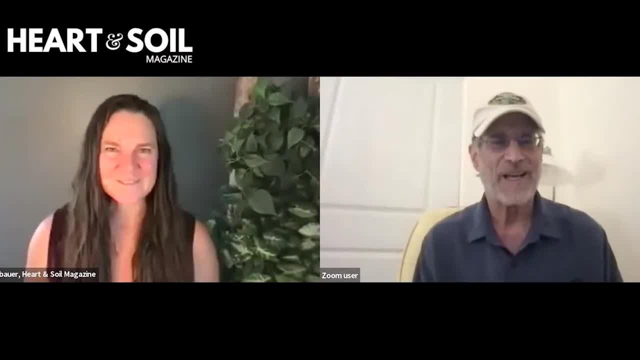 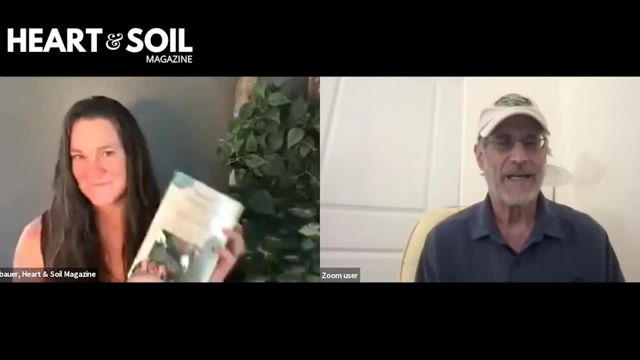 Yeah, nice to meet you. Nice to meet you too, Jeff, I'm deeply honored to spend some time with you. Sure, Yeah, Look what I have here: Teaming with microbes, not bacteria, because we're here to talk bacteria today, right? 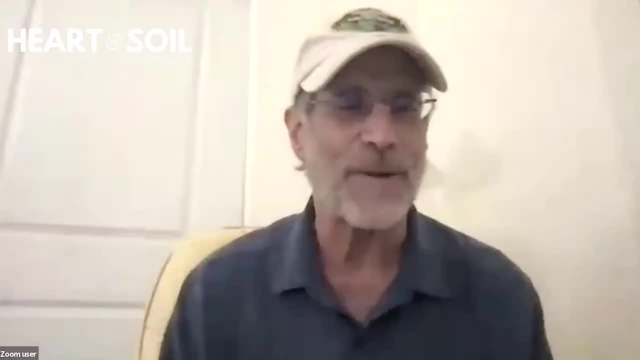 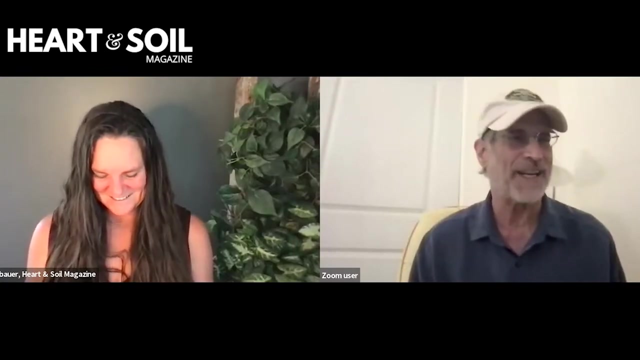 Right, But that's it. Well, we can talk anything you want, but that's a very, very early one. I hope the mistake on page 47 with regard to the pH has been corrected. The first edition that came out, the pH definition was reversed so that if you added hydrogen ions, 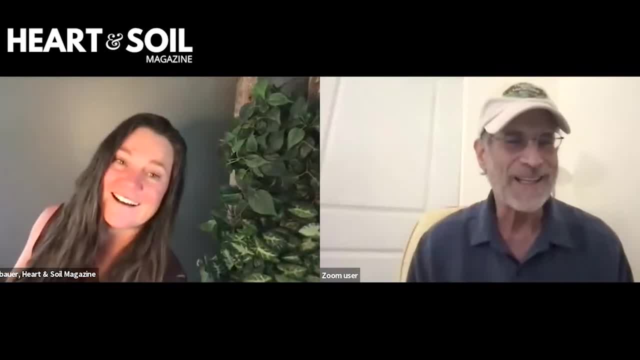 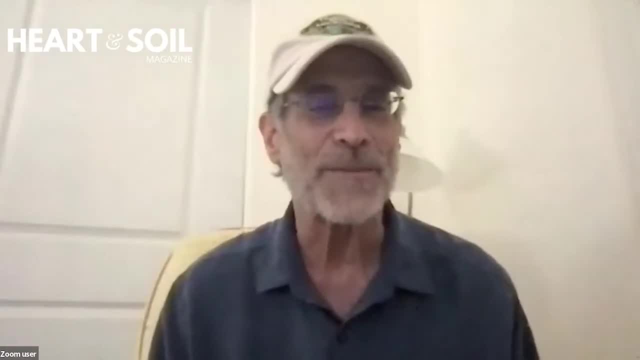 it didn't lower the pH, it raised the pH, and that's wrong. So then, every time they come out with an audible or a different edition, it picks up the original mistake, even though we fixed it a couple of times. but you should be okay if it's not the first print. Oh snap, You know what This? 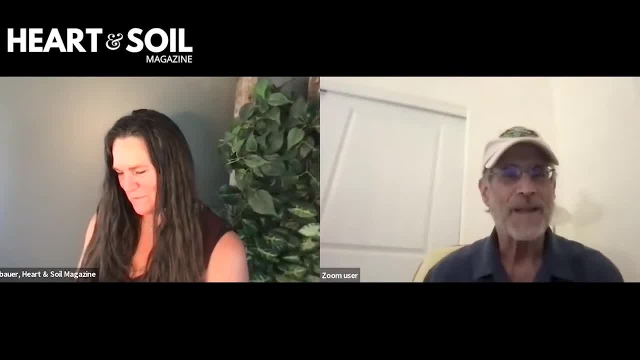 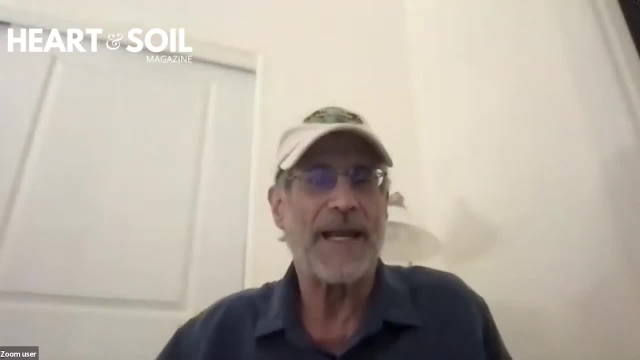 actually might be an earlier. When did you publish this? What year? Oh, that's the 2006,, but it was revised and republished in 2011,, I think, or 10.. Yeah, And I'm pretty sure. 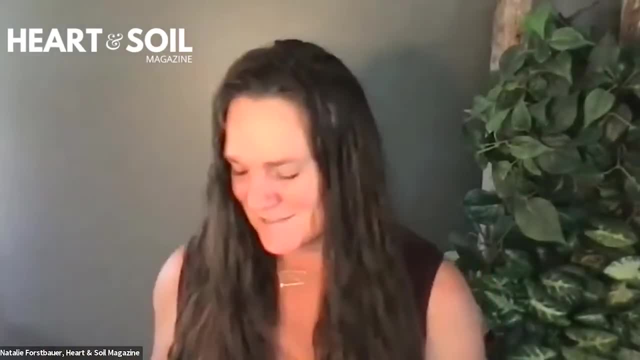 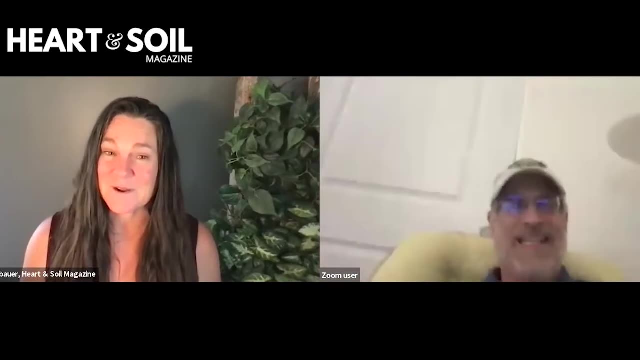 I got this early days, early early days. Wow, I did Elaine Ingham's training in, I think, 2007.. I think that's around when I picked it up. Sure, sure, That could be an early one with. 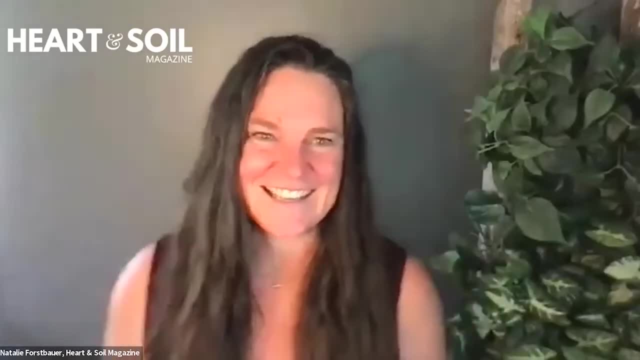 a mistake, but that's okay. If you haven't found it, we're okay. Yeah, we're all good. We're all good. I've wanted to. I've followed your work for a long time and I've wanted to have a conversation. 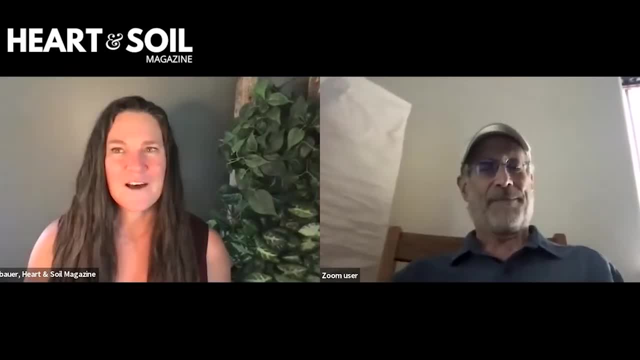 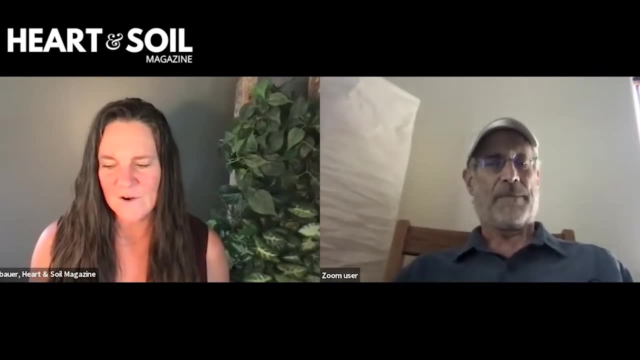 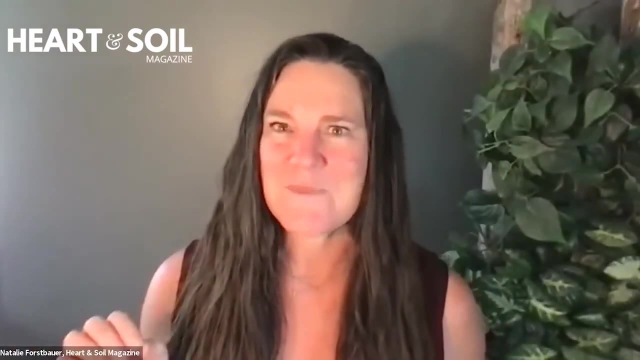 with you or many conversations with you about the work you're doing, for a lot of different reasons. One is because I think it's so curious how you are not necessarily the scientist or the expert behind the words or the findings And at the same time, there's this deep passion for what you're. 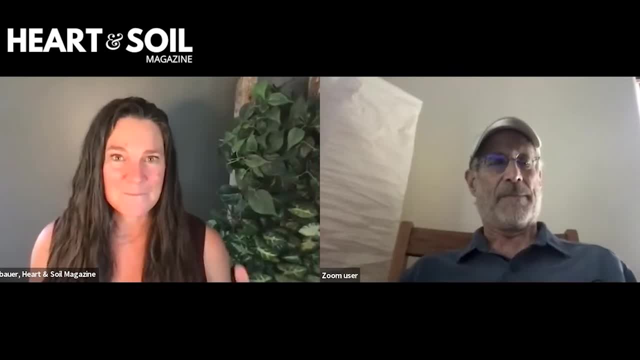 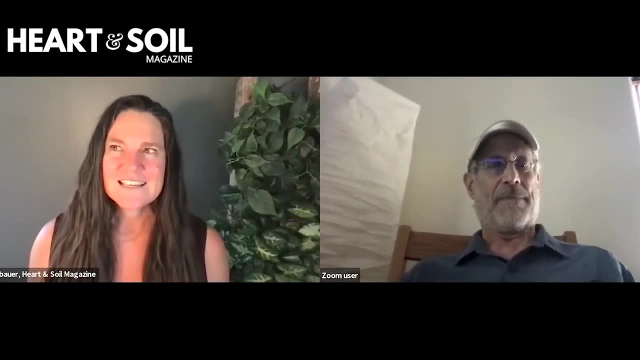 doing and this deep desire to share what we are learning and discovering beneath our feet, And so that is really curious to me And I'm wondering what drives you? what drives that want and desire to talk about microbes and bacteria? and well, I mean, it's the system that works and most people don't. 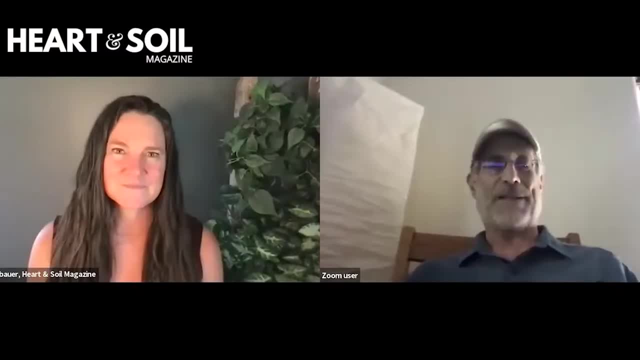 know about it, and so they don't really know what they're doing, and that's that's unfortunate, because once you know the system, you can do what you do better, and we really, we really do need to do something about our soil, and all of this ultimately leads to better soil, which ultimately, 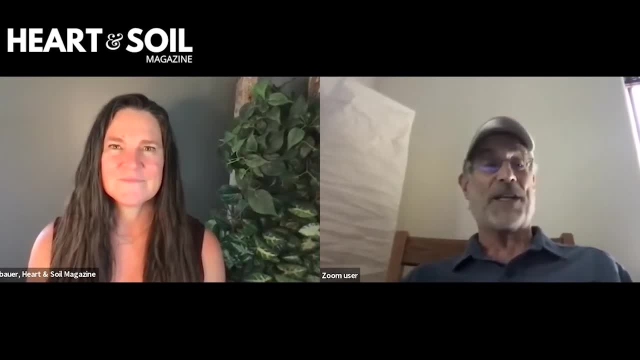 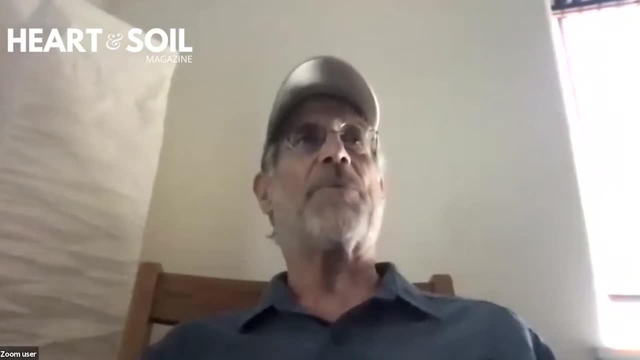 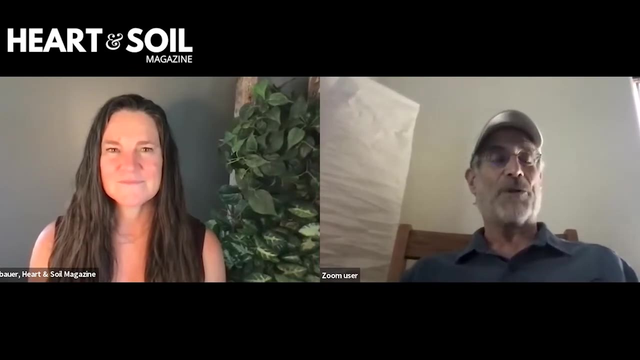 leads to another season of the 60 that we have left. maybe, if we do it right, we'll have 61. you know, it's a very, very important subject, so to see people mess it up really is upsetting, and so I guess that's what drives me is is wanting people to do things the right way. And why is soil so? 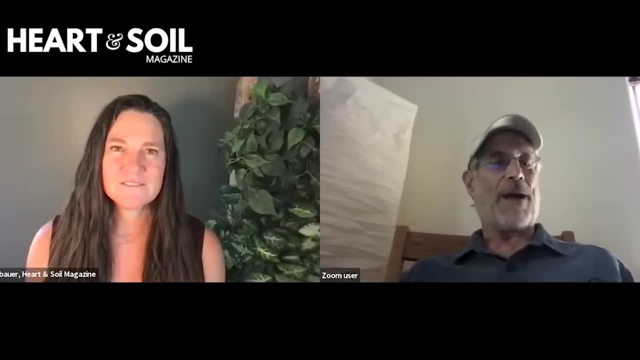 important, though. what's the importance of that in the equation? Well, no soil, no food. I mean, soil is the basis of everything, and so so, yeah, sure, you could do it hydroponically, but not the same, you know. and so if you don't have good soil, the things we love don't exist, and 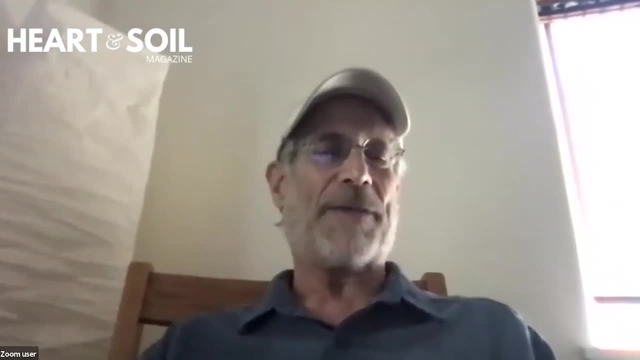 that's just the bottom line and we're not treating it very well and we have a serious, serious problem that we need to take care of. Tell me more about that. when you say we're not treating it very well, what do you mean by that? Well, when you use chemicals there, there are not only impacts to the plants, which are negative. there are impacts to the soil because you change the soil food web, you reduce the numbers of bacteria, things like that that are attracted to the plant, and those are the things that create soil structure. the bacteria have a slime which causes individual particles of soil to stick together. fungi come. 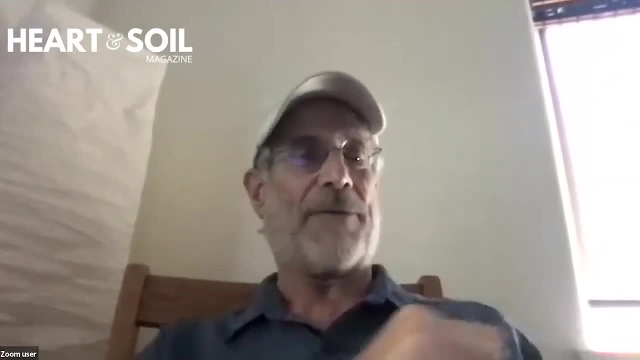 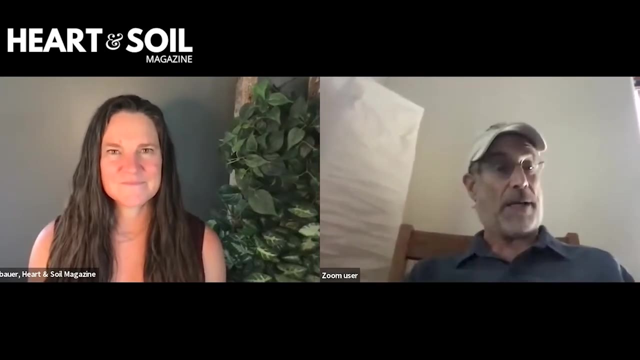 in and weave those little slimy things together and you end up with these aggregates. they're not bricks, they're not flat, so they have poor spaces. air can go in, be held there, water can be held there, microbial space for you know, protection from from the bigger. guys. they're trying to eat the littler guys and basically soil structure. that's where it comes from. it doesn't come from the plant. it comes from the microbes that are in the soil. and when you destroy those microbes or you displace those microbes by rototilling and and doing things, 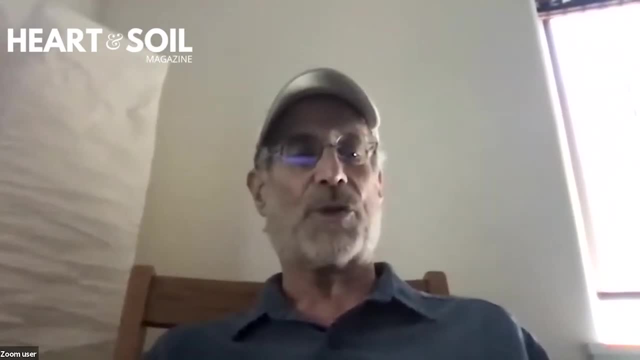 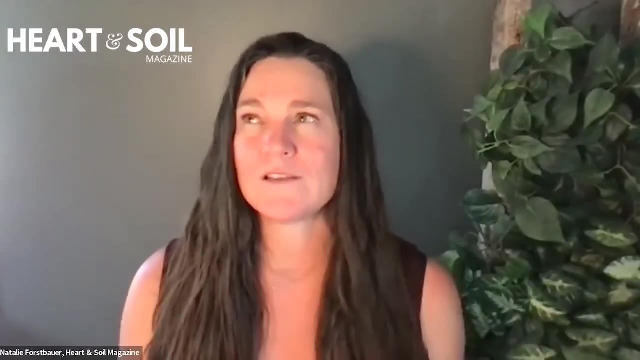 like sterilizing the soil. you end up creating a situation where soil structure is being destroyed, not created. And so what happens when we focus on creating soil structure rather than destroying soil structure? The buzzword these days is: soil structure is being destroyed, not created. 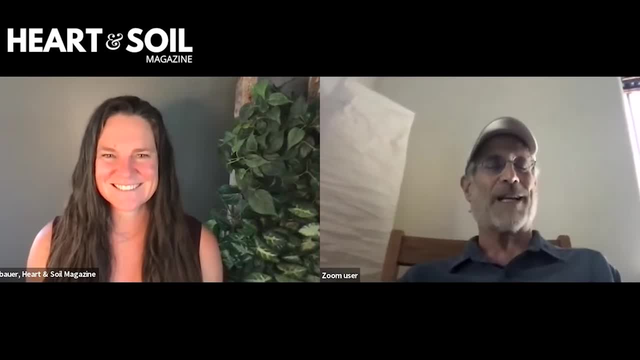 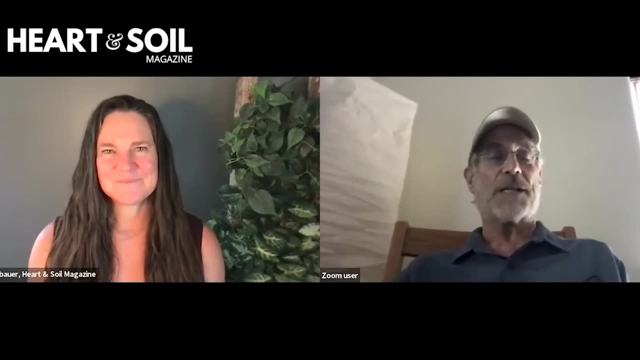 The buzzword these days is regenerative. when you, when you focus on on soil structure, you you're focusing on putting back into the soil things that have been taken away and making sure that it's maintained in a way that it regenerates itself and the goodies that are in it and that 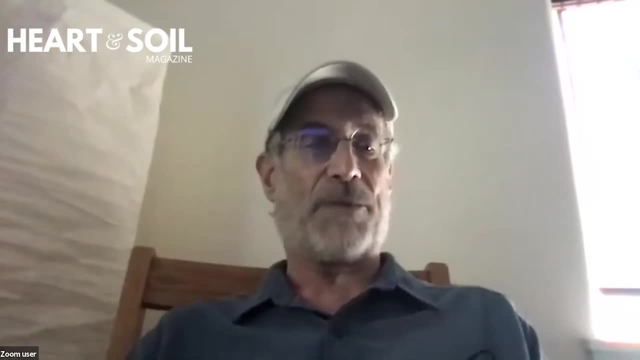 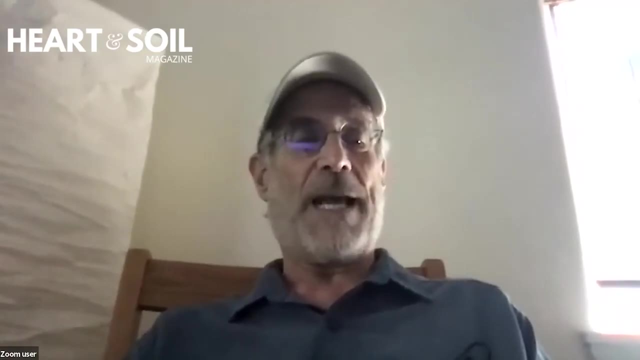 and that's what happens and we've got a serious, serious problem because we have been brainwashed into thinking you need to be a chemical and that you need to fertilize like crazy, and all of these things turn out not to be true, Rototilling being. 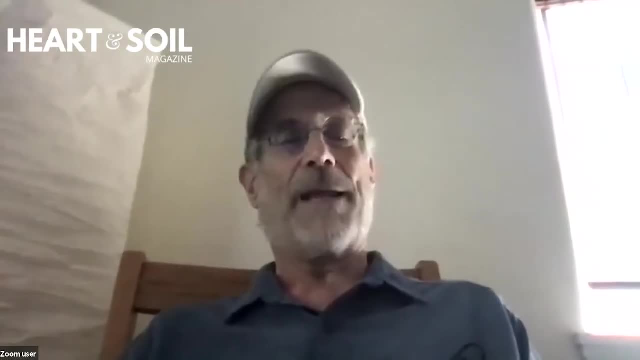 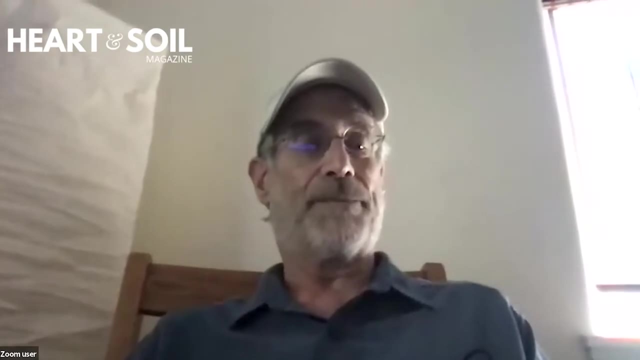 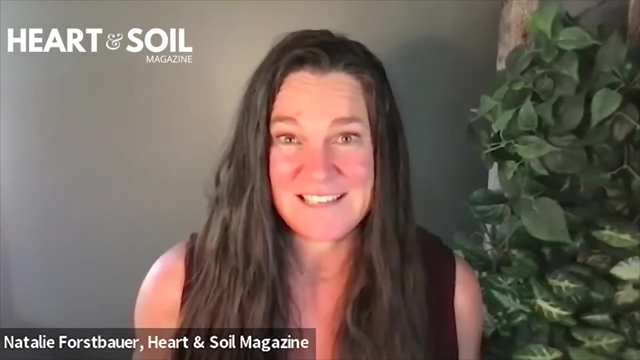 one of them, and so we need to go back to the system that respects and protects the soil food web and protects and respects the microbes that are the basis of that soil food web. What do you say to the gardener who's used to tilling their garden and even maybe using like 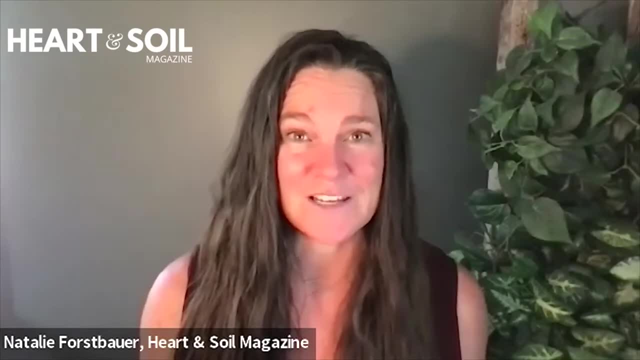 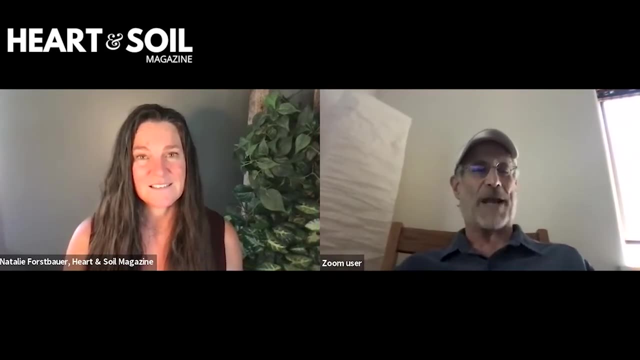 chemicals on it before they plant it, or maybe even while they're- while they're gardening. what do you say to them? Well, I tell them how the soil food web works. I tell them: the plant is producing exudates. The exudates are attracting the bacteria and the fungi. The fungi and the bacteria are attracting the nematodes and the protozoa. We eat the fungi and the bacteria and poop it out, and that's how plants feed themselves. and then I say to them: who do you think feeds the redwoods or a local forest? wherever I happen to be, and it takes about. 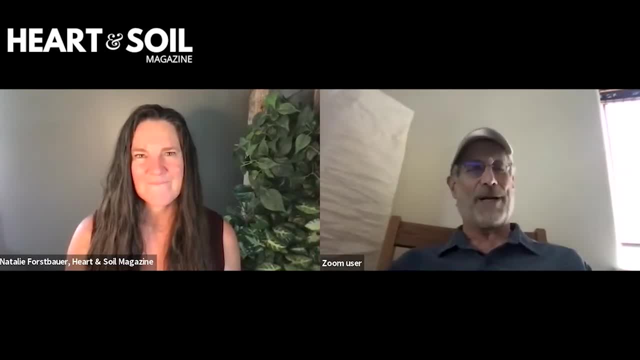 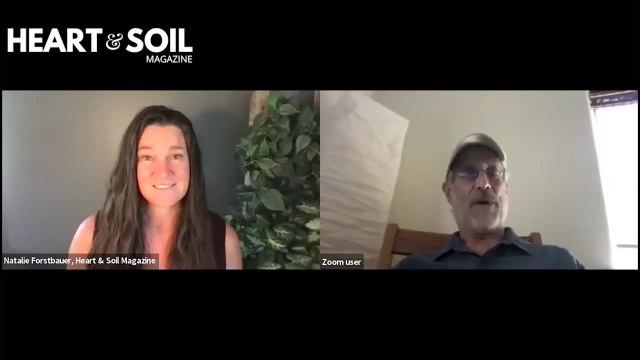 20 seconds for them to say, gee, I guess I don't need to be doing all of this stuff. Okay, they stop. Okay, okay, so they stop. but then where do they start? Well, it's pretty easy to add organic matter to gardens. People can use mulches. People often compost, even though 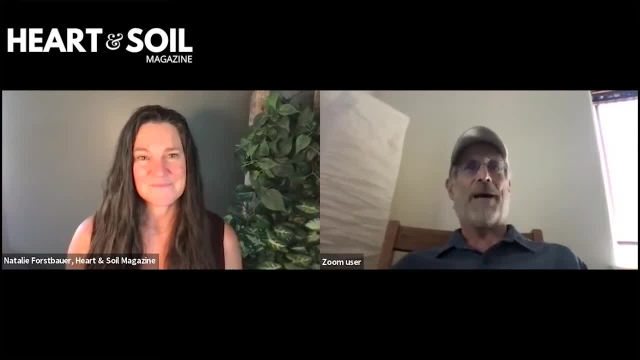 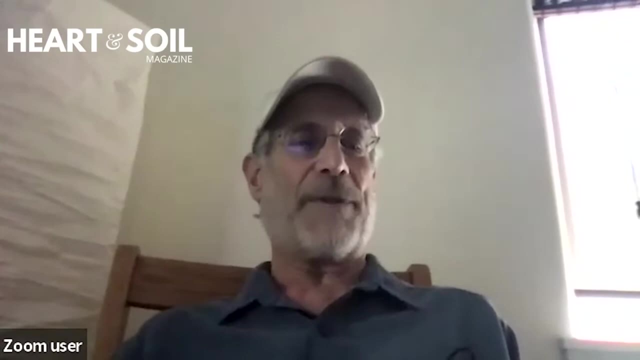 they're chemical so it's easy to use compost. Both of those things return the microbes to the soil and people can use compost teas and some of the sellable products that people are now producing that can return microbes back into the soil. Certainly when they plant they should be in if 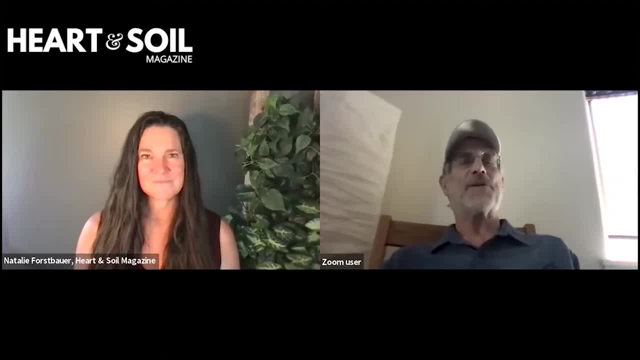 they're going from a chemical to a non-chemical situation. they need to be using ecto and endo mycorrhizal Fungi, depending on what they're planting, and they need to pay particular attention to the biomass of their soil. We, you and I, have a mutual knowledge of an instrument called the. 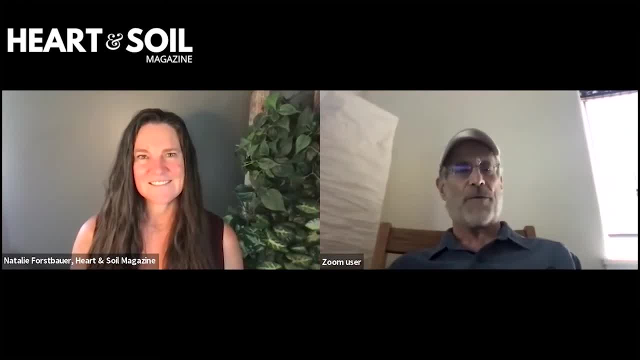 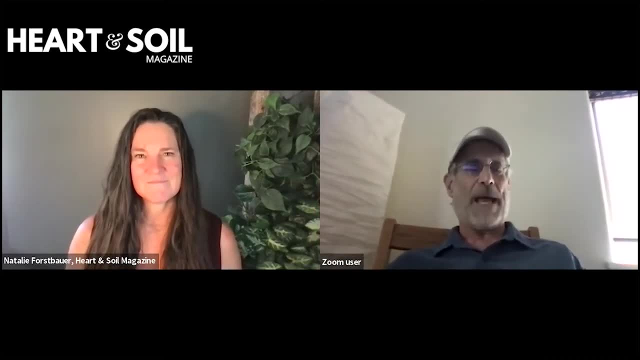 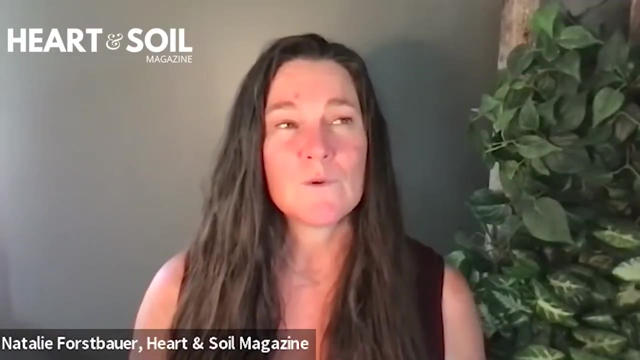 microbiometer. If you're adding to the soil and your biomass of microbes is increasing, then you're doing things right. You are helping the soil food web and you are moving forward. I love how simple you make that, because sometimes people can get really overwhelmed with learning all the, all the things, all the protozoas and the fungi and the. 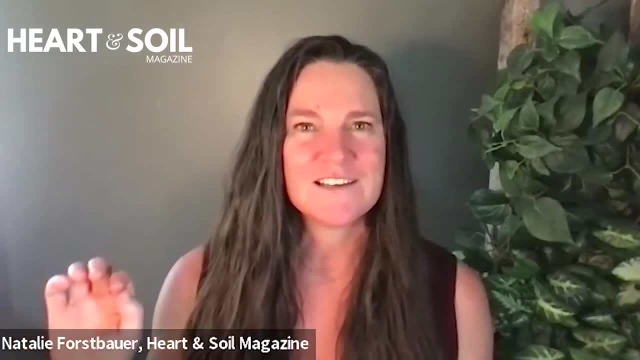 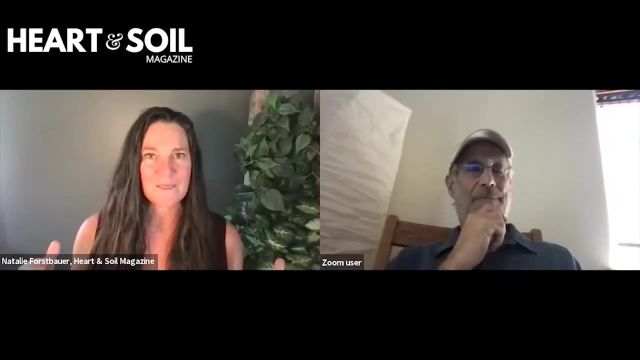 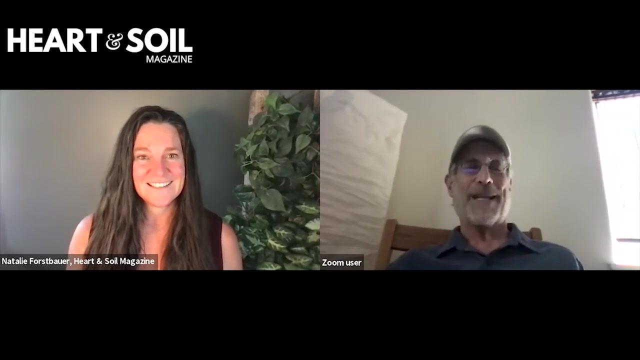 unpronounceable words for a lot of people, and so just know that they can measure the biomass of the soil and get a reading, and to understand that adding organic matter moves the needle Powerful right. Sure, although they shouldn't, shouldn't have any problems remembering their 10th grade. 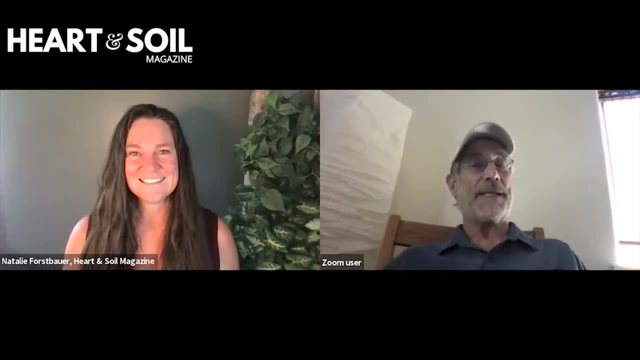 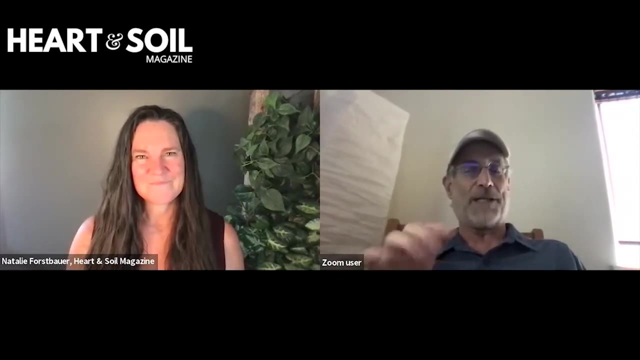 biology class because they studied paramecium and omicron. They didn't study nematodes unless they happened to pick up some pond water and and they, they studied bacteria for about two seconds because they couldn't really see them, other than these little dots moving around. So yeah, you know, when people have some familiarity. 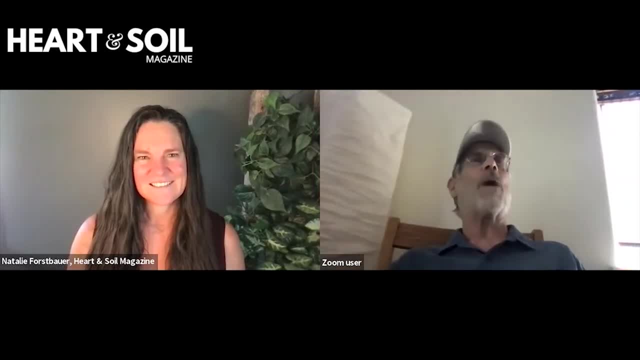 it's just we got to scratch back there and and figure out why were they teaching us this stuff? because they didn't know why they were teaching us this stuff. Now there's a reason, and I and I hope schools change and say to them: you want to study these things because this is how you garden, You know that's, that's important. 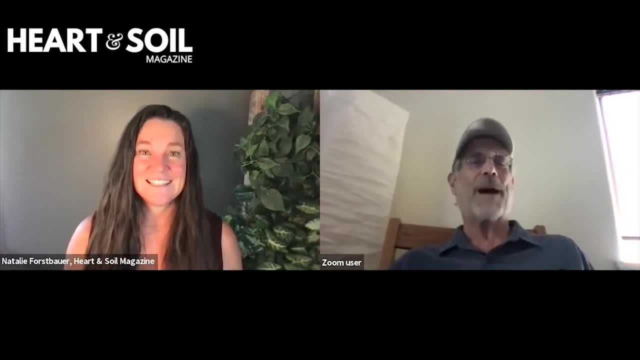 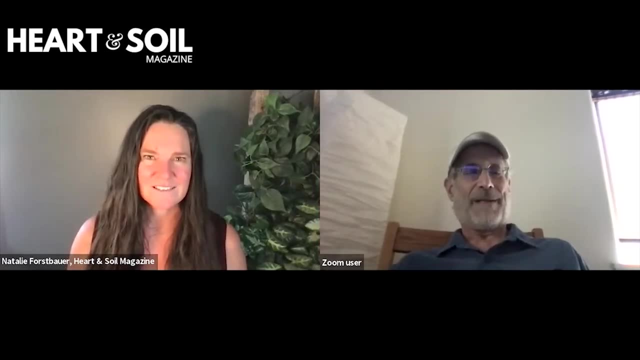 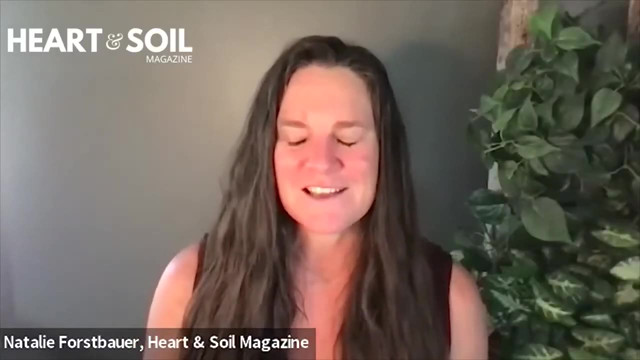 Let's stop studying dinosaurs and start studying microbes. That's yes, yes. could you imagine you could imagine the shift in the world if that's where we started? Yeah, yeah, it would be amazing, It would be amazing. So let's talk teeming bacteria, Jeff, because it kind of blows my mind the way. 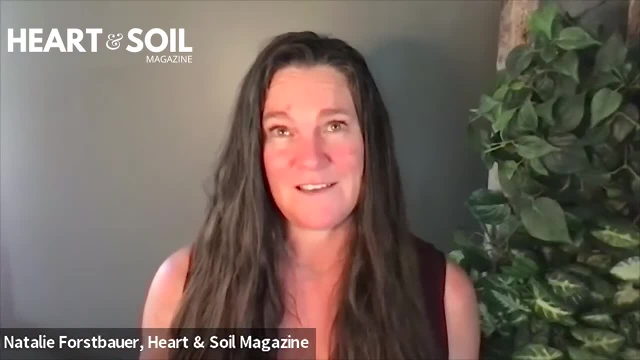 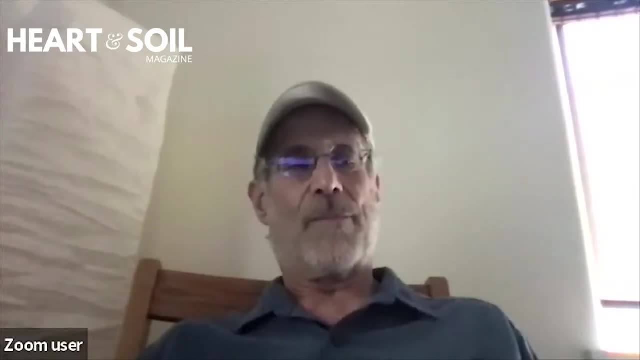 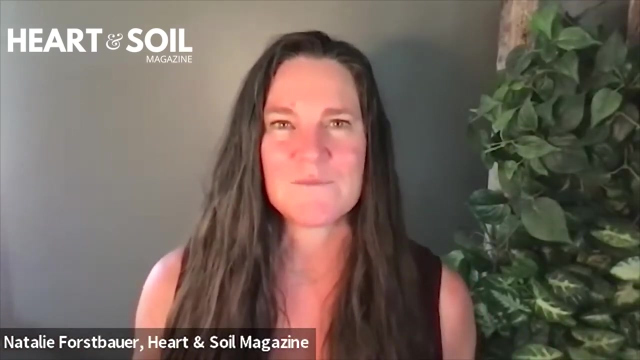 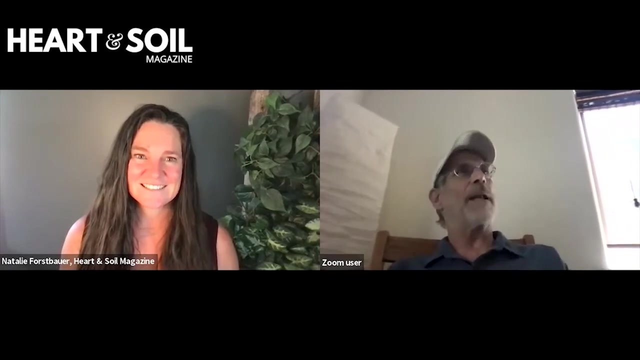 the what we're discovering around bacteria completely rewired And shifts the paradigm of how we experience or what we thought was working, how and how it's working differently. So, before we dive into teeming with bacteria, tell us what bacteria is and why it's important. Okay, well, and let me see if I can also tie it into the soil a little bit. I mean, 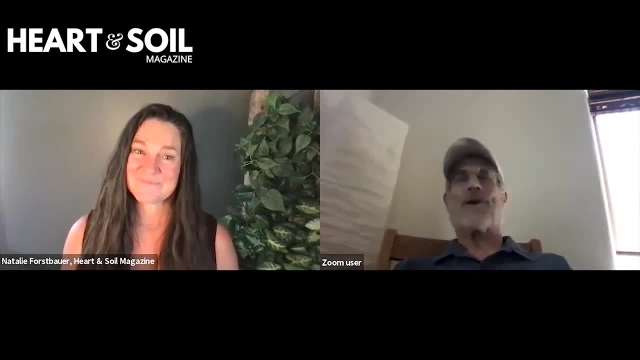 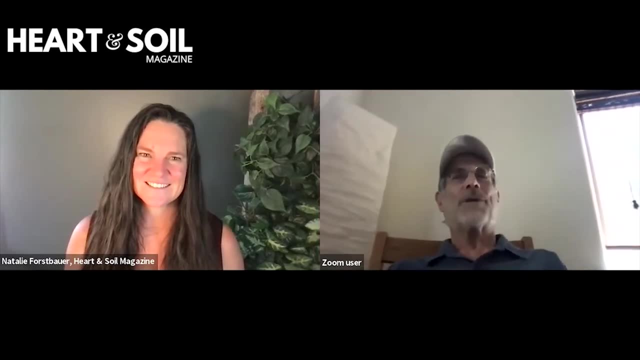 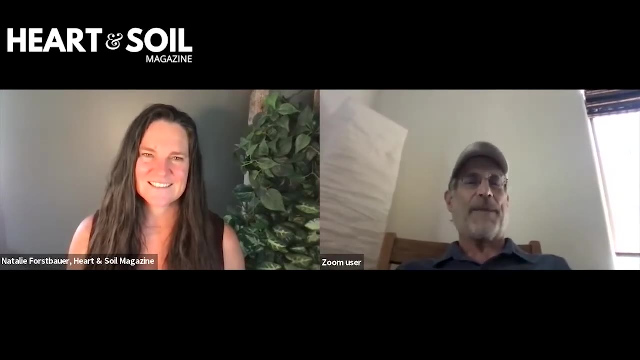 bacteria are everywhere. Of all the organisms you can write about that, this is the most plentiful one. All you have to do is use an internet search engine- google, whatever duck duck, go and put in the words bacteria, head of a pin and go to go to the images and up will pop an image that I didn't use in the 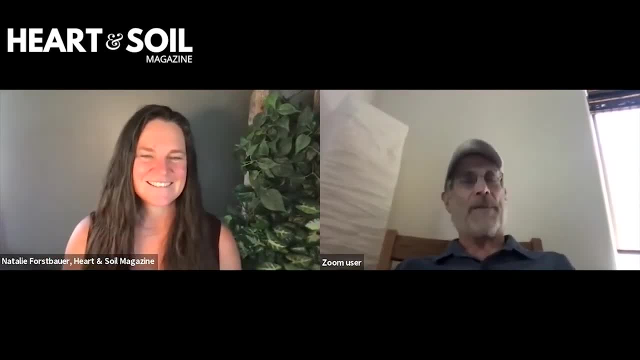 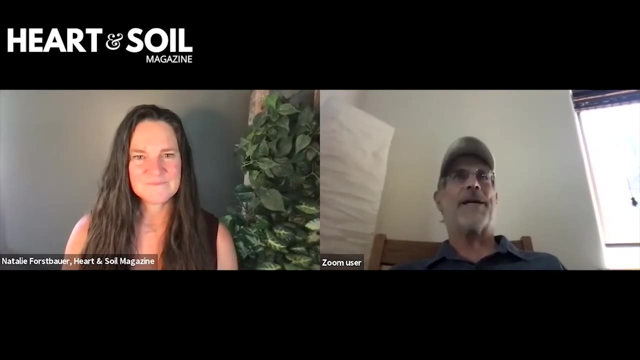 book, because they wanted 400 for it- of a pin. tip the pin covered with bacteria. So when we say bacteria, you know people, their eyes, they don't. you don't think numbers, you think bacteria, you know, you think, oh yeah, bacteria, it's the plural bacterium, bacteria. you know, you might think. 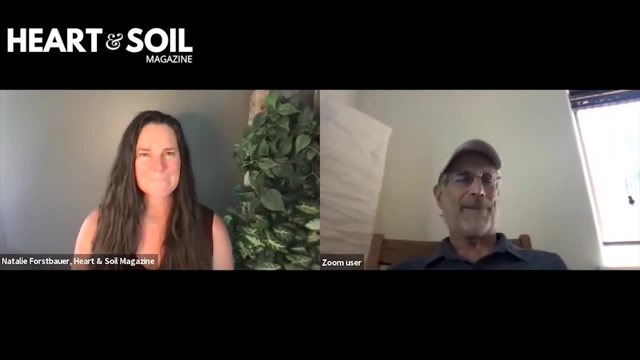 of the cars in a family parking lot driveway. what you really should be thinking about are the cars at the Hartsfield Atlantic airport parking lot. they are everywhere, they are ubiquitous, they breed like crazy, they multiply every 20 minutes, uh, and the numbers are too staggering to even 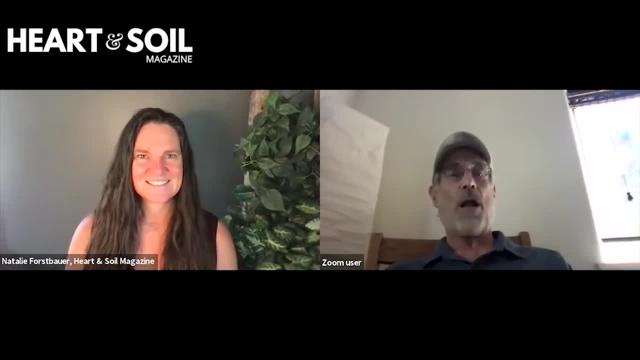 even think about it. So we're going to talk a little bit more about the bacteria. and bacteria Think about, and their size is so small that to consider that they've got all sorts of organelles inside. you know they carry chromosomes that they can talk to each other, that they can have sex with. 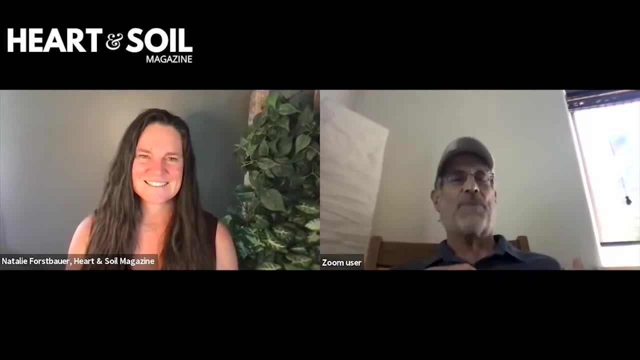 each other. it's just and and that they produce all of these beautiful metabolites that go out into the world that do things like create antibiotics, etc. etc. and now we discover feed the plants. it's really quite something. and so the bacteria themselves, which I spend a little bit of time discussing in the book. that's amazing and the most amazing thing about. 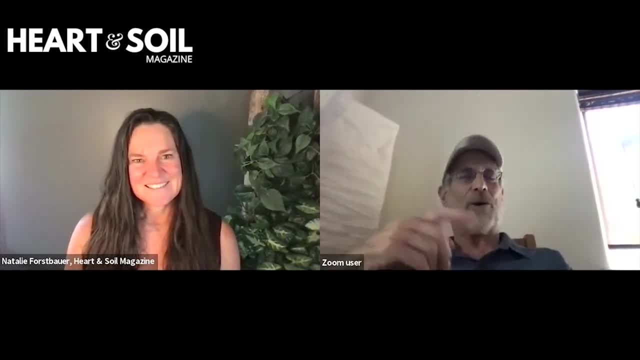 them are the flagellums, the little propellers that cause them to move around, because apparently they're so small that swimming doesn't make any sense. you know, when you and I jump into water, we glide through that water. eventually we sink. when a bacteria jumps into a water, it's stuck. 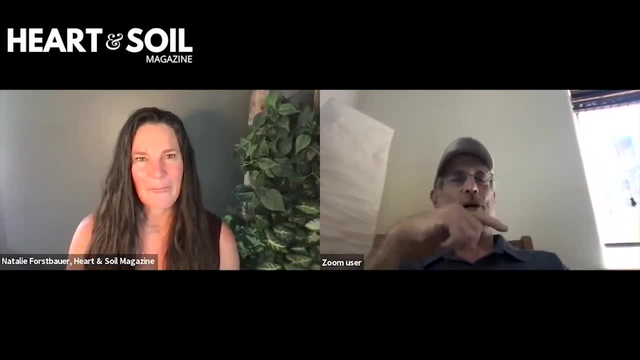 and it can't really move. so some bacteria have a corkscrew shape. that's how they get around in this viscous liquid, and most of them have developed these unbelievably complicated engines- literally engines that have moving parts that look just like a jet propeller- I mean an airplane propeller called flagellum- and that's how they move around and 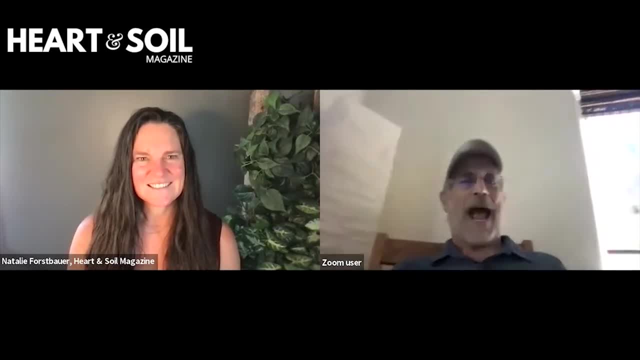 they are. they are simply amazing. But I thought what you were going to ask was: how has the soil food web changed as a result of this new knowledge that we'll talk about in a minute of this web, and so let me, let me see if I can give you a little bit more detail on that. 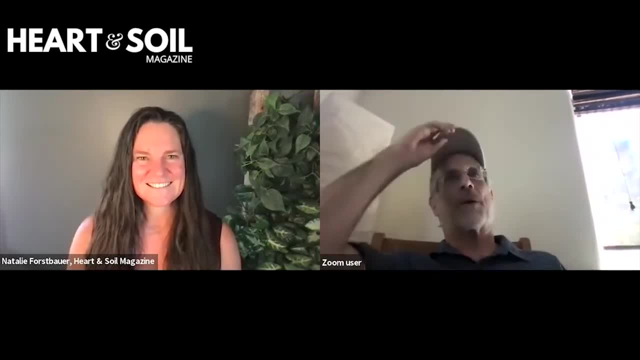 So let me let me see if I can give you a little bit more detail on that. So let me let me see if I can give you a little bit more detail on that. So let me let me see if I can sort of give it a sort of a description. when I learned about the 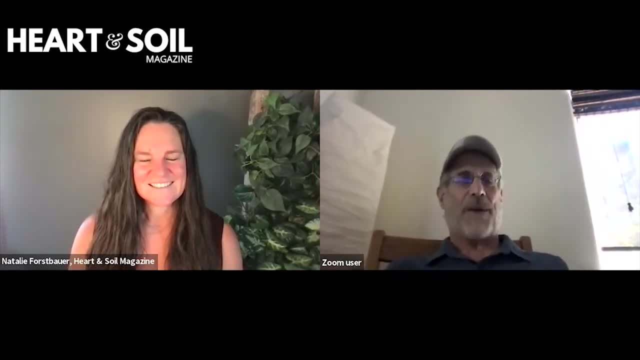 soil food web from Dr Elaine Ingham and when. when all of us learned about the soil food web, it was Dr Elaine Ingham's research and her description of the soil food web, and what we discovered was the plant was a farmer and all the plant needed to do was take that photosynthetic energy, create some. 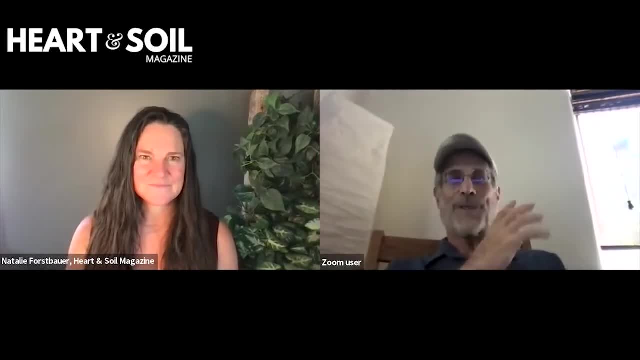 exudates inside the plant, teeming with nutrients. we'll describe how that works, if anybody wants to read that book. and then drips them out of the out of the roots, right out of the root, tips these exudates, and Elaine calls them candies and cookies. they're carbons, they're amino acids. some of them are. 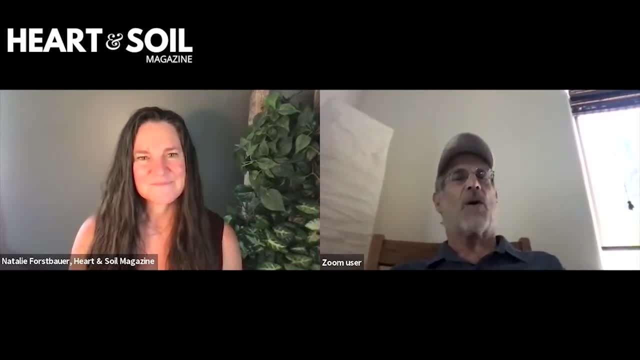 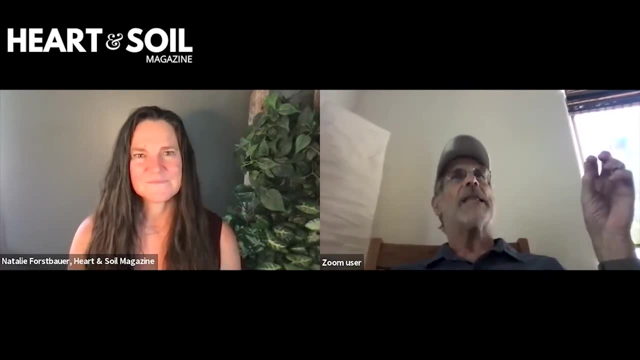 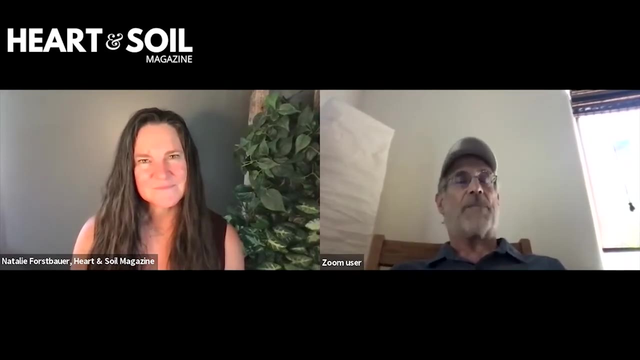 enzymes. they're little molecular delights that go out into the soil, into the rhizosphere, that area right around the roots and that exudate, is designed by the plant to attract bacteria and fungi that the plant continues to feed because the plant is farming those bacteria and fungi. 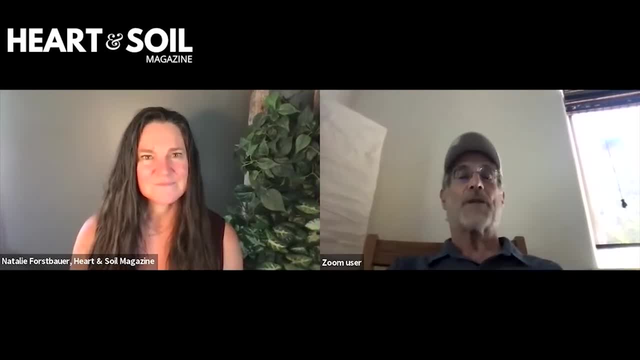 and their populations grow, and they grow big enough so that they in turn attract the nematodes and the protozoa that eat them. and the nematodes and protozoa eat them. they poop out the excess, and this excess material then moves towards the plant. either either is. 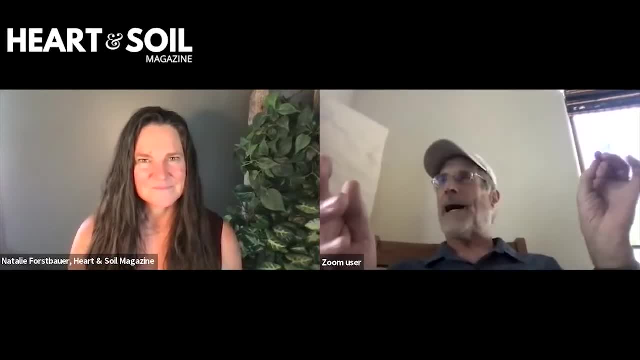 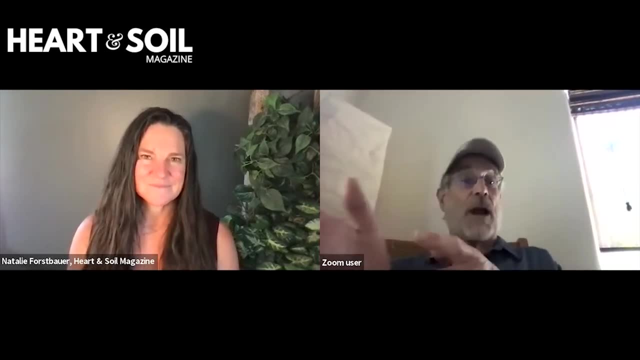 a result of, of flow, uh, osmosis- not really osmosis, because it's the reverse direction- they move towards the plant, they hit the plant and then, as described in teaming with microbes- uh, i mean in teaming with the nutrients- they move into the plant as a result of the plant putting. 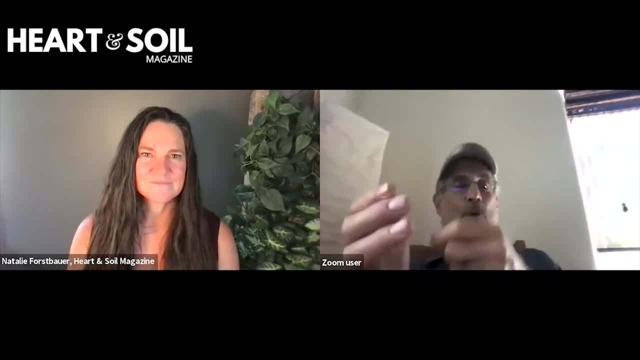 out some hydrogen ions and attaching to them and moving them through these special membranes, uh, that are in in the cell. so the the plant is literally farming these bacteria and these fungi. they're getting eaten, and then the plant is harvesting the goodies that are. result: the manure is then being, you know, collected. that's the soft food web that you and i 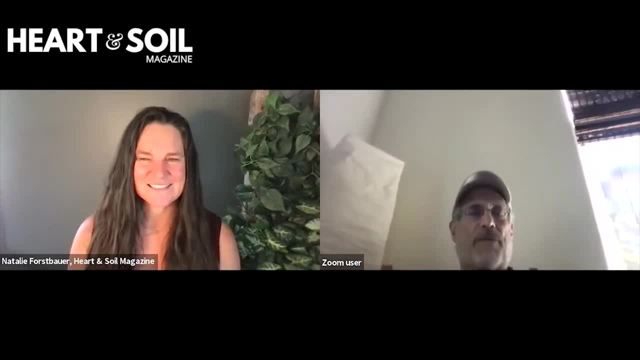 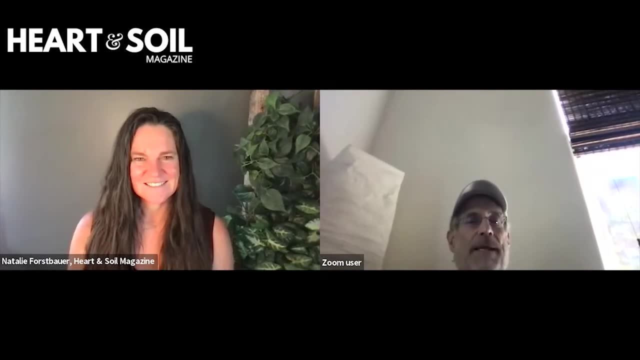 learn and we love it. and that's how, how you know the first, the first three books talk about that. now the variations on that soil food web are a fungi, basically mycorrhizal fungi, because mycorrhizal fungi, attracted by the plant, it's always the plant that does the attraction- move in between the cells of the root and bring 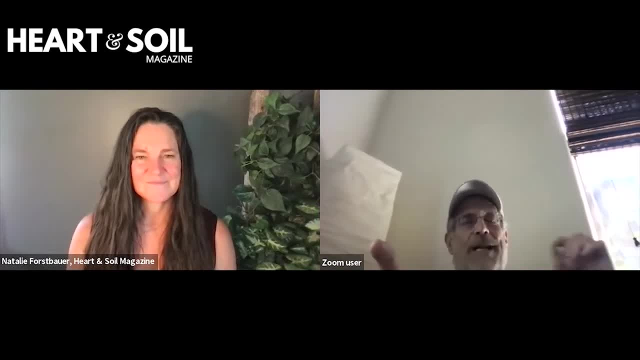 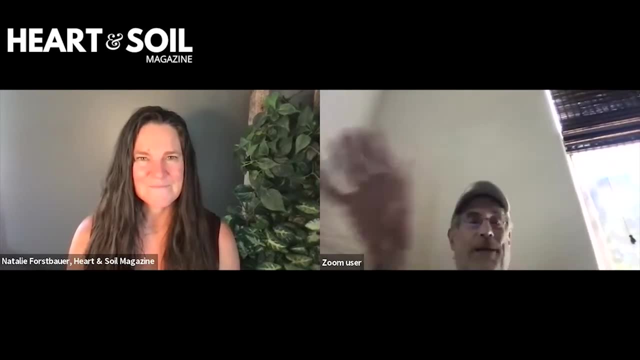 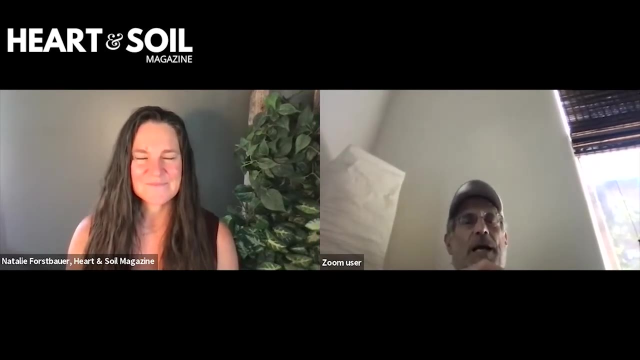 food to the plant. so you've got fungi bringing food, uh, internally, so to speak. and then you've got this fungi that are, you know, outside getting eaten up and being pooped out, that are moving nutrients in, and then we have some bacteria that fix nitrogen in certain plants, legumes, and so so. 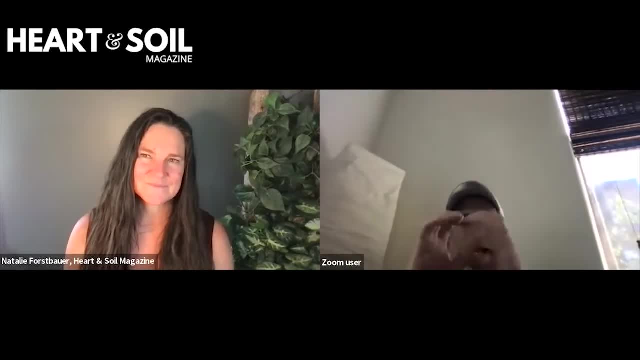 we've got, we've got, you know they. they've got some bacteria that fix nitrogen in certain plants, legumes, and so. so we've got, we've got. you know they they're also attracted to the plant they they go to a root hair. the root hair curls around it. they turn into. bacterioids. they produce nitrogen. some of that nitrogen leaks out into the soil and goes back into the plant, and when the plant dies, those little nodules break up and that soil goes back into the plant. so pretty exciting stuff. and now, as a result of a discovery that was made in australia, 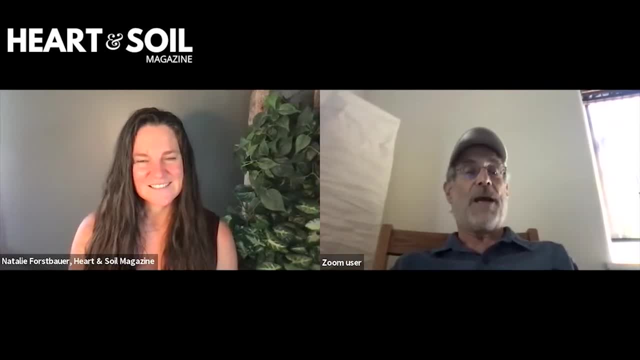 uh, and has been really perfected, uh, in in new jersey, uh, by dr james white. we now know that there is sort of a another way that nutrients get into a plant, and that the plant acts not just as a farmer, but the plant acts as a rancher. and here's how it works. 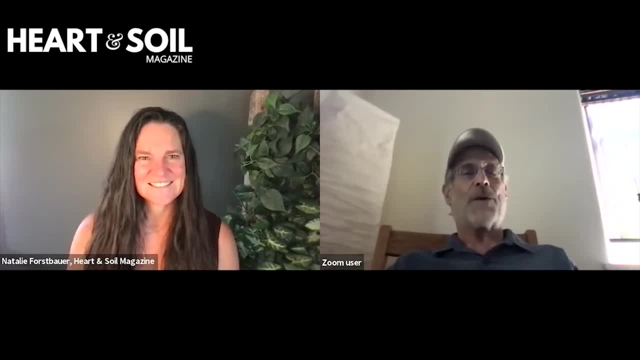 so those exudates have attracted bacteria. some of those bacteria are tricked by the plant, which creates a particular set of smells in a situation that makes these bacteria think that there's an empty soil, and a lot of bacteria get attracted to the plant. that's what we call the miscellaneous bacteria. 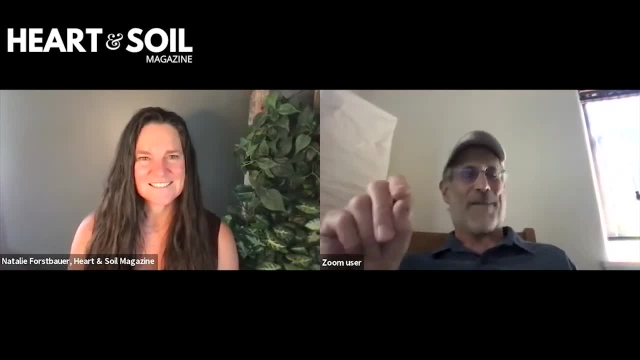 slime hole right at the tip of the meristem cells and they move into that little empty space and they they end up backing into the meristem cell itself. so you have bacteria entering the cell. now they've been attracted by the plant. okay. so far everything sounds the same. 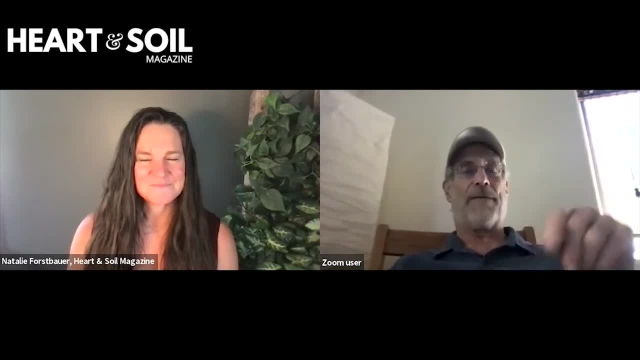 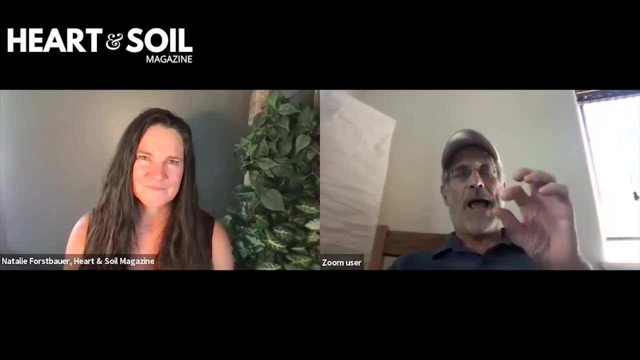 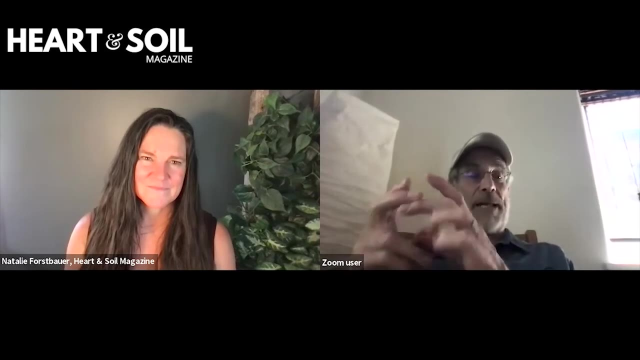 there's some of the same bacteria that are in that little pile of bacteria that keep getting eaten and pooped out, but these are inside the plant, so they go through the cell wall and then they enter a space between the cell wall and that area that has that membrane that. 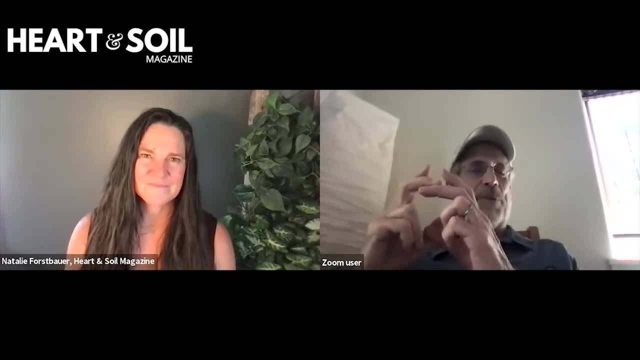 contains all of the organs inside the organelles of a plant: the chloroplasts, the nucleus, you know, the ribo, all the good stuff that's in there, uh, but there's this empty space. so if you think of a tofu container that you buy at a supermarket, 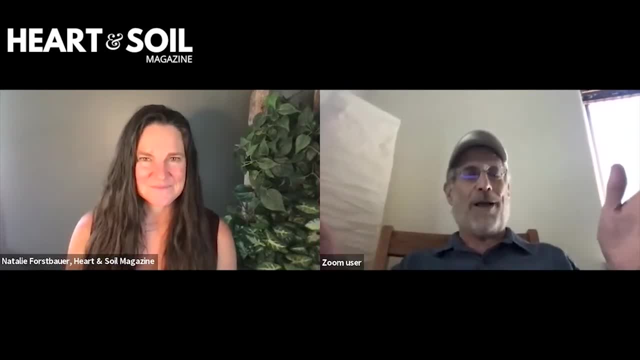 it's got the white cell wall, it's got this liquid which is the paraplasmic space. that's where the bacteria are. and then it's got the chunk of tofu, that's, you know, sort of the inside of the cell. so you've got these bacteria in that liquid at the outside of the tofu container. 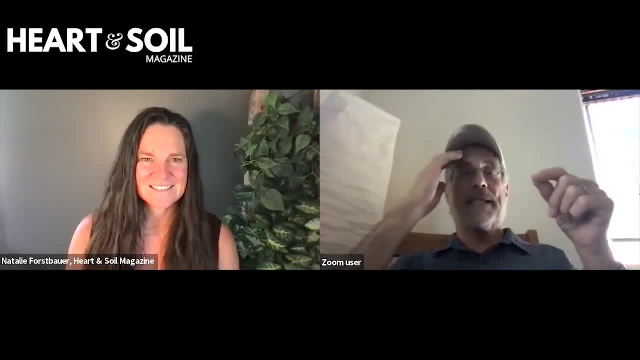 and they're in there and once they get inside, the plant goes: oh, bacteria. and it sprays the bacteria from a little enzyme that sits in that membrane and it sprays it with something called ro. it's basically, uh, you know, a super oxygen and that strips the cell wall off, the bacteria. that cell wall contains a lot of little teeny micronutrients and they're absorbed by the plant. now remember i said bacteria, think hartsfield, you know airport, don't think you're back driveway, you're talking thousands and thousands of bacteria that are moving into the cell and once they move in that cell they have to protect themselves also. they don't want to lose more than their cell wall, and so they produce nitric acid that tends to reduce the power of this oxygen, that gets put on this ro and and that ends up mixing with this ro stuff and producing nitrates, nitrogen. you have fixation of nitrogen in that little space and you begin to get. circulation of these bacteria as they are multiplied. every 20 minutes they double. they don't have a cell wall, so it's probably less than 20 minutes and it's much easier to get double because there's no cell wall on them and they're circulating in that little space that. 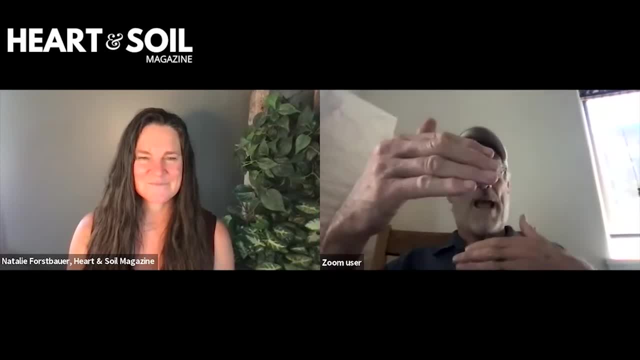 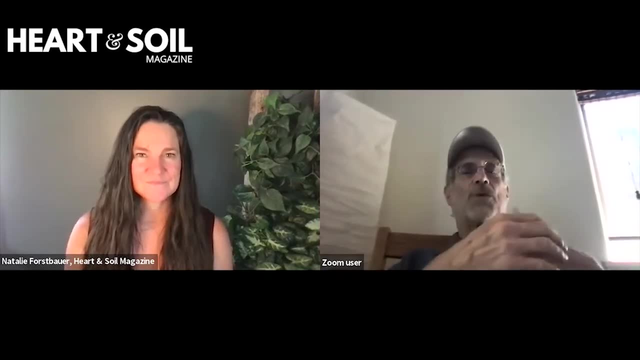 little liquid space between the tofu and the container and they're bombarded with this ro. they're continuing to produce nitrogen. it's absorbed by the plant. the plant throws out a little bit of its exudate into that area and that exudate allows these bacteria to produce. ethylene. so it's producing nitric acid, which turns the nitrates, and it's producing ethylene. ethylene causes young cells to stretch and to grow, and so it causes the plant cell, this little root cell, to grow a little bit and as they circulate around and get multiplied, they end up with numbers that 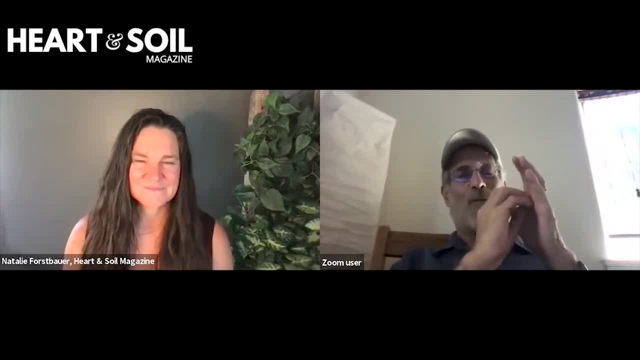 that get caught somewhere in that container wall. you know how that. that container is made out of plastic and it's a container wall and it's a container wall and it's a container wall and it's a little rough edges, you know little well it gets the bacteria get caught there and they begin to. 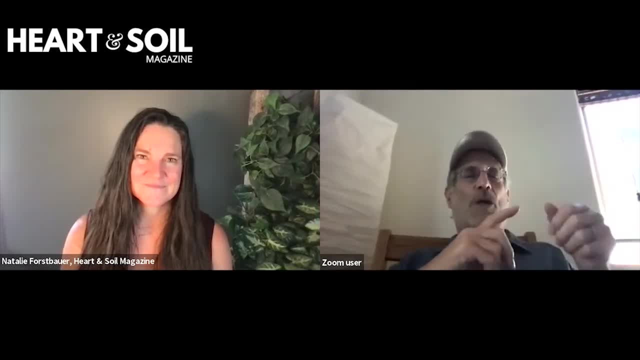 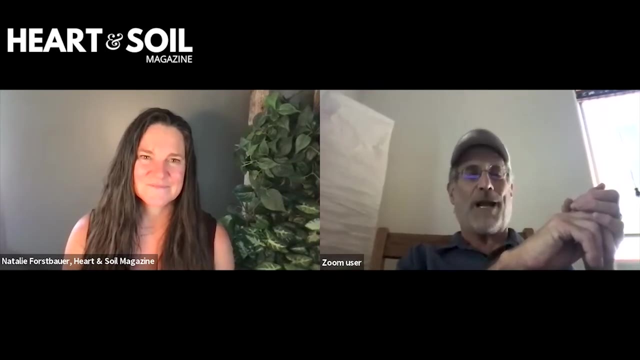 accumulate and they're continuing to produce this ethylene which pushes or causes a tube to form in the cell and that tube moves out into the soil. you and i know that tube to be a root hair. these bacteria cause root hairs to form. the plant doesn't get caught in the soil. doesn't form those root hairs to get nutrients. the bacteria's ethylene causes that root hair to grow. it's part of the meristem cell and as it grows the bacteria then find a way to move into it. there's a small little wave of of periplasmic liquid that pushes the bacteria in more further. 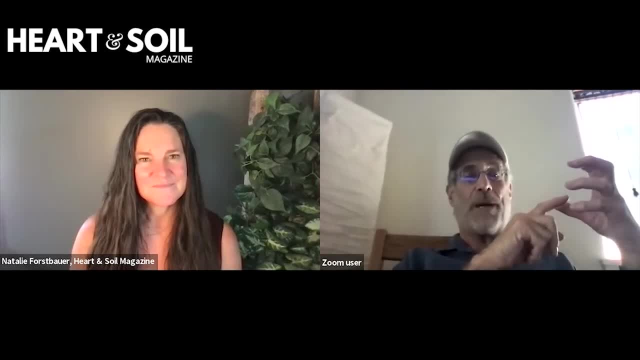 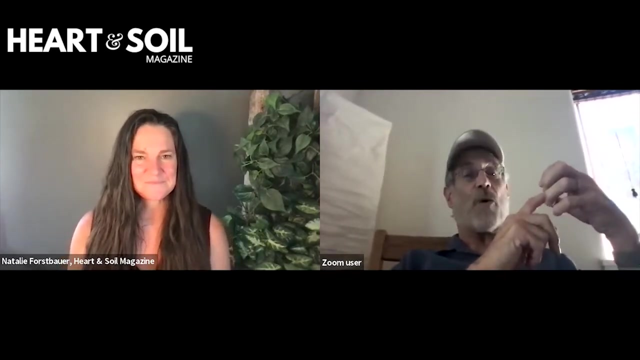 and boom, the root hair pops open, the bacteria are blasted out into the soil and they're going to grow back into the soil, where they grow back their cell walls, and then, two or three days later, make the trip again through a new meristem and end up making a new root hair. now this root hair blows. 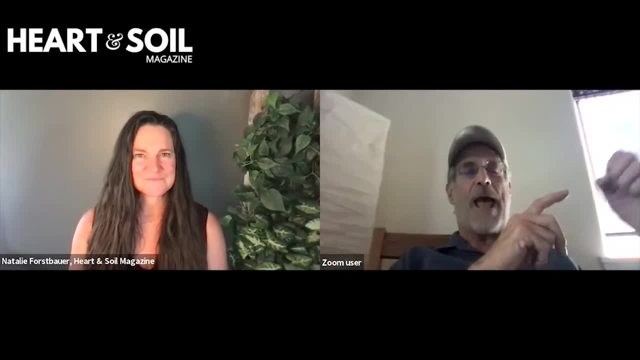 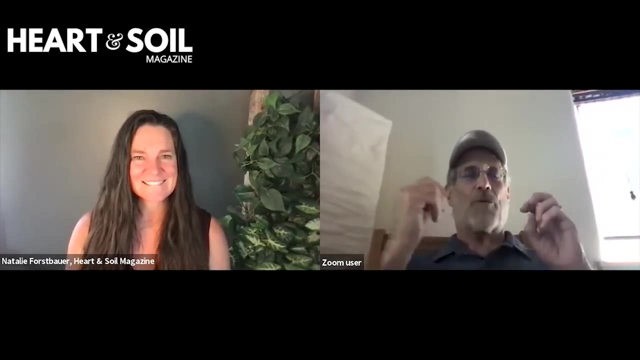 up four or five times. so you get four or five of these explosions all the way up and what's happening is the plant is ranching these bacteria, shearing off their wool, taking some of this, the pork chops, yeah, and then the rest of the stuff back out into the corral. where they grow back their wool, get their pork chops back again and go back into the plant to feed it. up to 30 of nitrogen comes from nitrogen that's fixed this way inside the plant. what a discovery this is. so you've got. you've got the farming and the ranching going on at the same time. 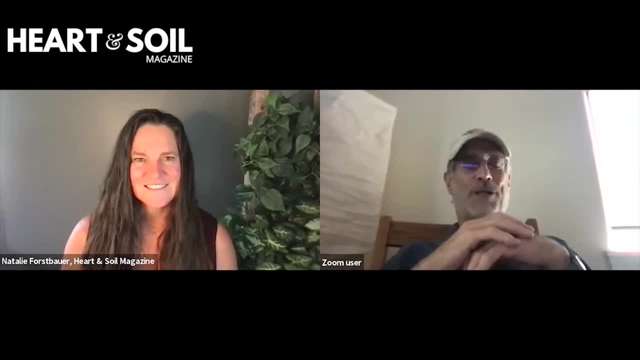 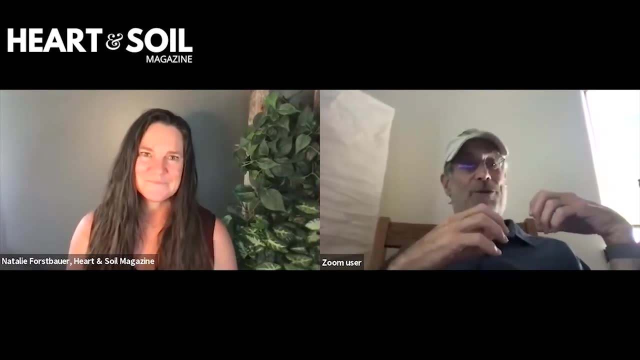 and and to really open up questions now: the research that dr elaine did to end up with a farming portion- fabulous. the research that dr james white and his, his, his students and others around the world, of course, but really it's james white and his students at rutgers university. 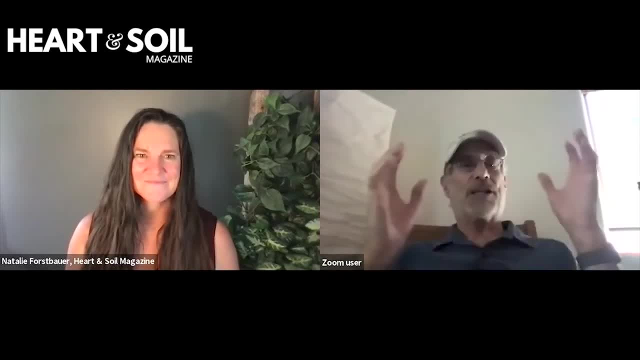 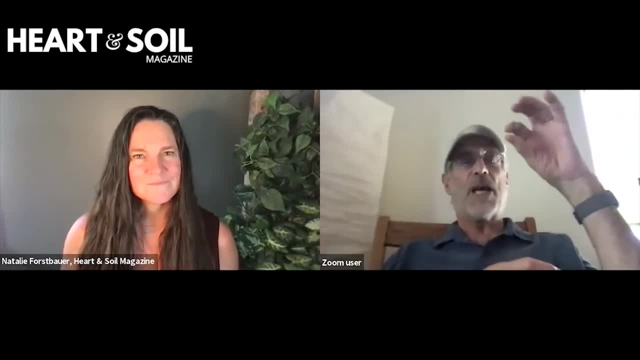 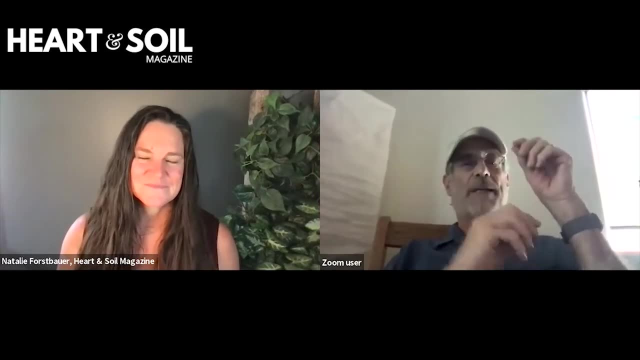 hormones that cause the plant to have different capabilities. gibberellic acid, which makes the plant grow, uh sets fruit, auxin. all of these things are produced by bacteria in different parts of the plant, and then we discovered that the trichomes in the cannabis plant, for example, or tomato plant, 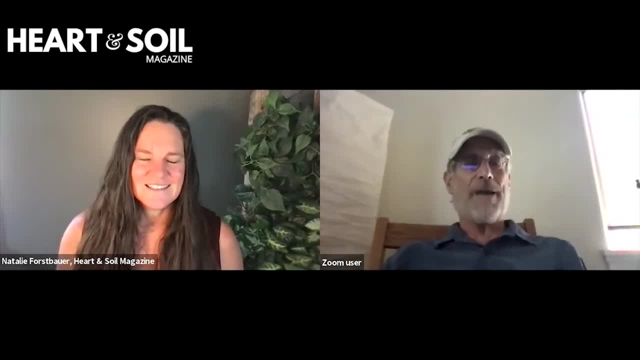 those trichomes act very much like the bacteria that are moving in the paraplasmic space in the meristem- not quite exactly the same, but there's a lot of connections between them. they're fixing nitrogen in those trichomes. now we know what those trichomes really do. they're a way for the plant to be able. we used to think. 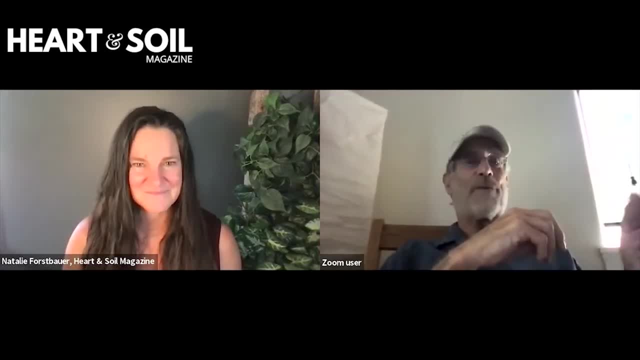 they're keeping insects away from the plant, keeping slugs off of blah, blah, blah. no, they're producing nitrogen. they're nitrogen fixation stations and some of that nitrogen bacteria. these bacteria spill out into the phyllosphere, that area around the plant, and create more of 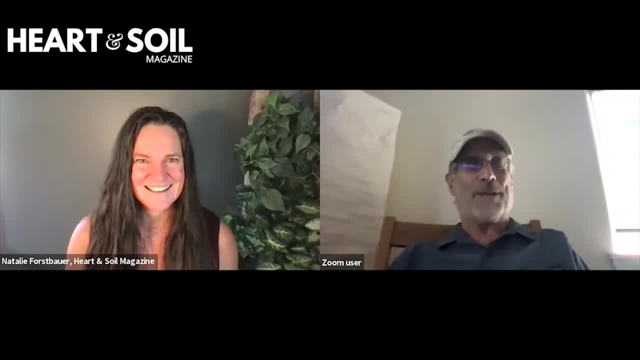 these. ah, it's just a spectacular situation. it's unbelievable and the pictures are phenomenal. the microscopy is every bit as good as it can be and it's just a spectacular situation and it's, it was during the original soil, food, lip stuff and, and so you know, we're just seeing stuff. we. 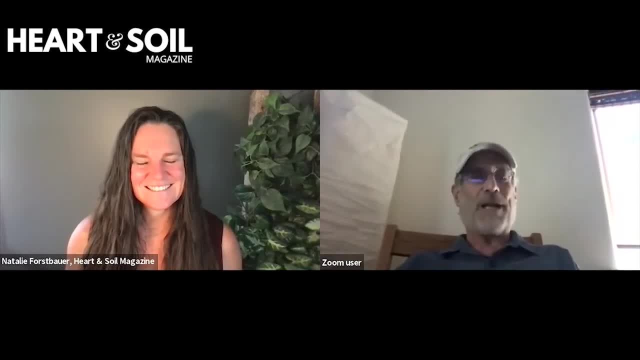 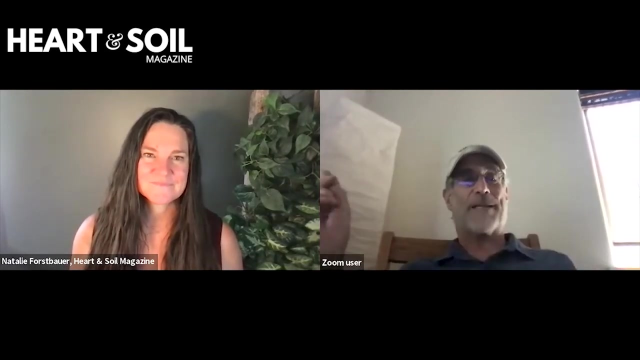 can't believe. and the take-homes are pretty clear, because these bacteria get trapped in the flower. the flower forms seeds, they get trapped in the seed coat and they're carried on to the next generation. so corn that's 400 years old has the same bacteria. 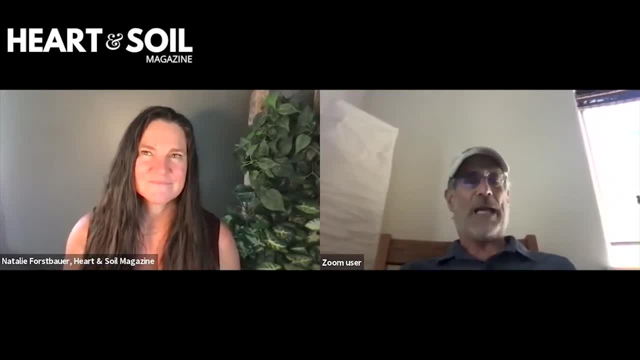 today that it had 400 years ago, unless somebody was stupid enough to sterilize the seeds or maybe to put too much nitrogen on the in the soil, etc. etc. etc. so it's really a spectacular discovery and and the implications are incredible and the fact that we now know that bacteria can fix 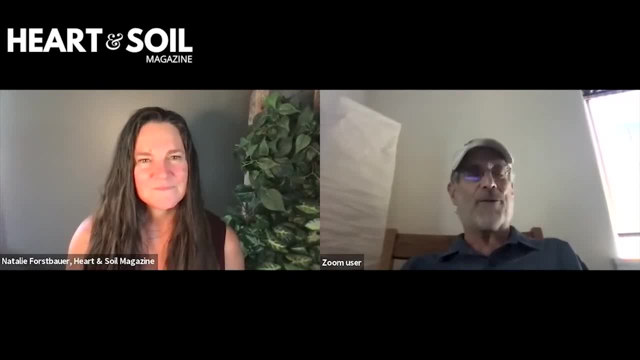 nitrogen in a different way than rhizobia bacteria that people put on legumes or that are in legumes, and that bacteria can fix nitrogen in a different way than rhizobia bacteria that people put on legumes, opens up the whole door of nitrogen fixation inside crop plants. 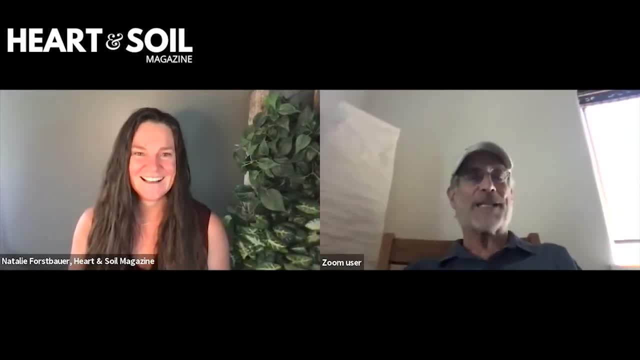 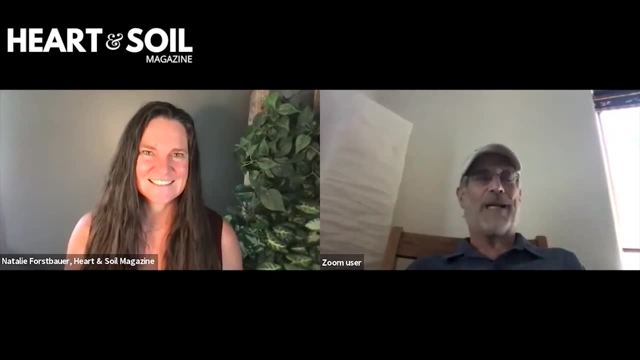 that was a big mouthful. the process, incidentally, that this wonderful woman whose name i can't pronounce because i just can't, and that dr james white has worked on at rutgers is called. i call it rhizophagy. there's lots of different ways to pronounce it: rhizo meaning root phagy meaning. 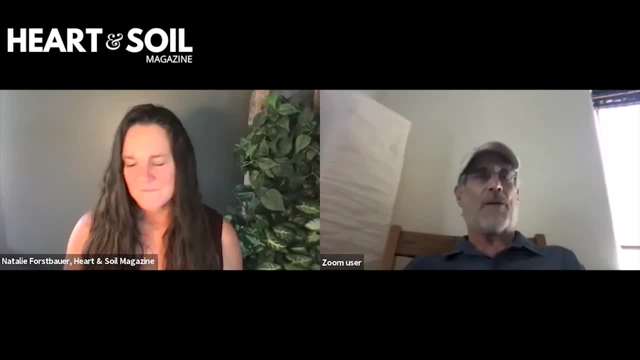 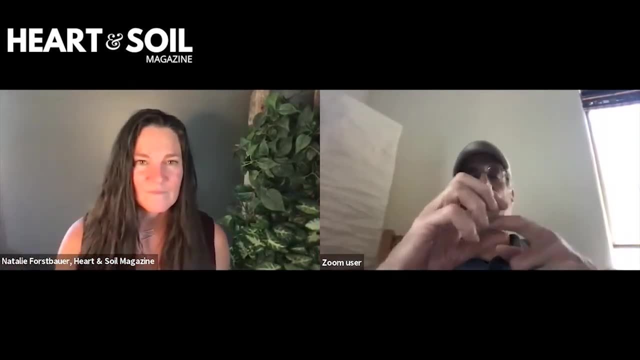 root eating because when, when the original discovery was made, the thought was that the roots were literally the meristem cells were opening up and engulfing these bacteria and bringing them in. now we know the bacteria are literally moving through the cell wall- uh, you know, on an individual basis as a result of being 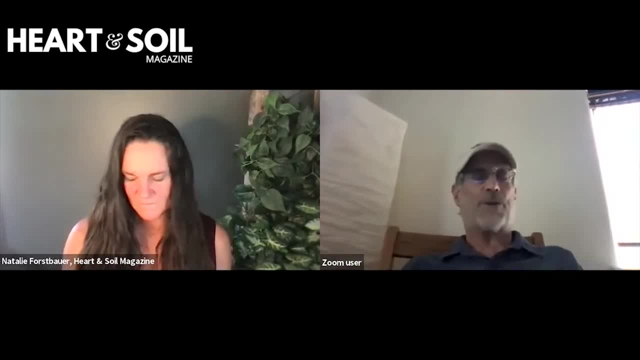 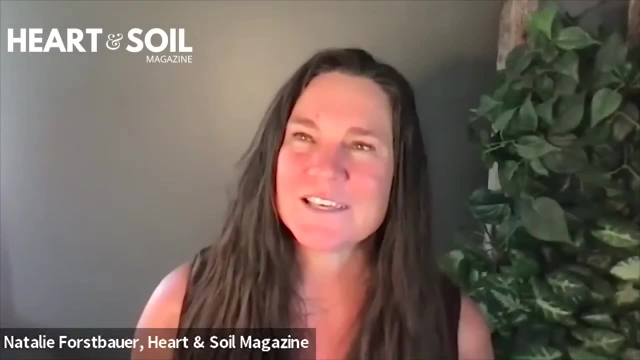 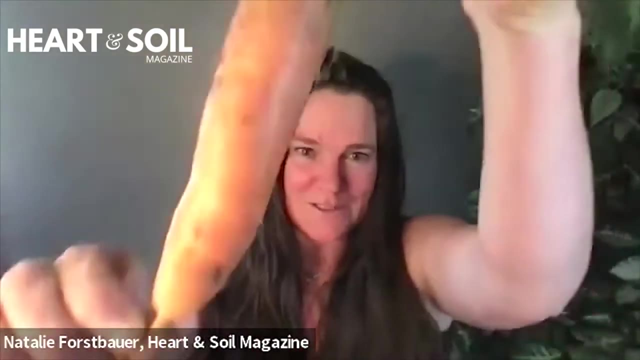 tricked by the plant. so really fascinating stuff and the pictures are just yowzer. yeah, that's, that's really incredible. there's nothing like looking at biology under a microscope. it's quite magical and i'm wondering if we can just simplify it with the carrot root. can we simplify? 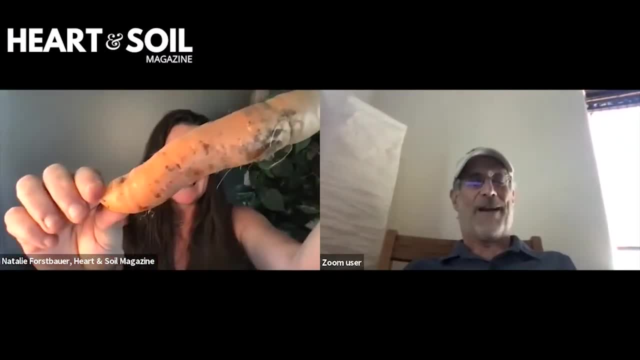 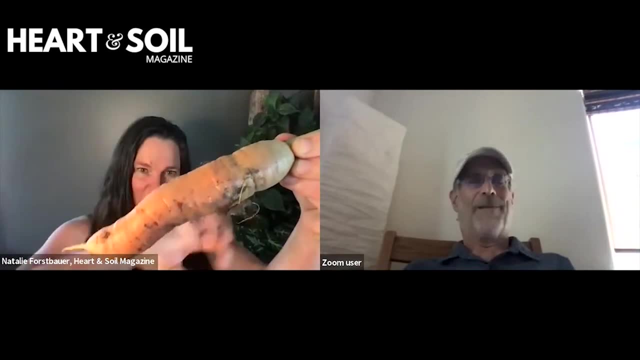 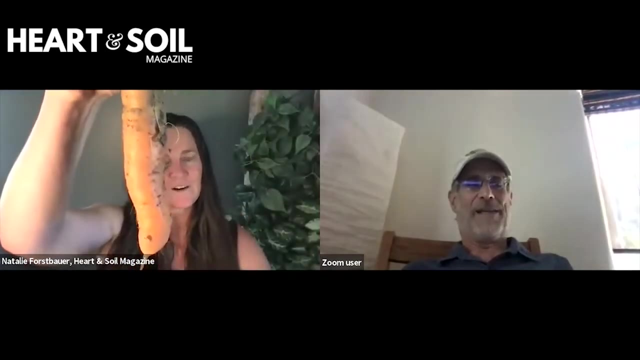 yeah, see those here. so what you're talking about here? yeah, so what you're talking about is the. the bacteria are taken in, so there's all these healthy microbes happening around in the dirt and the soil around the. this carrot and micro the, the carrot roots, will take the bacteria up in into here and 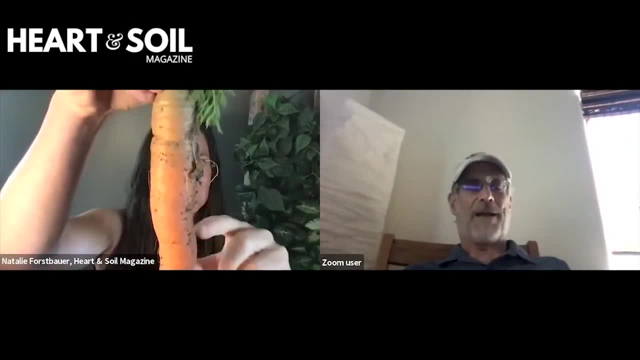 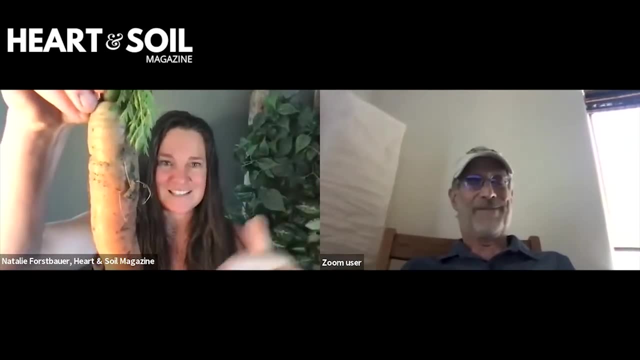 it'll do its magic, because we used to think that the plant would grow itself. right, that's what we thought, and we thought it would grow itself through the nitrogen and phosphorus and all the things. and then we learned about the soil food web and we learned that everything is being farmed. this, this is. 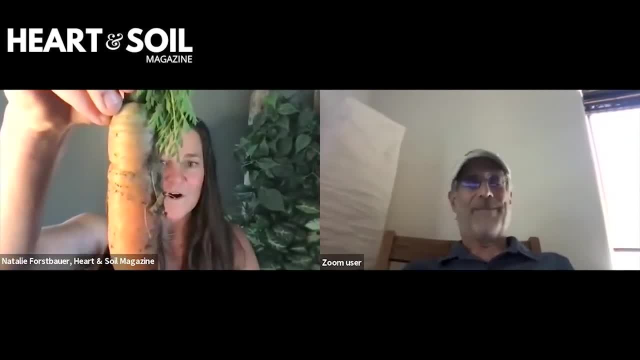 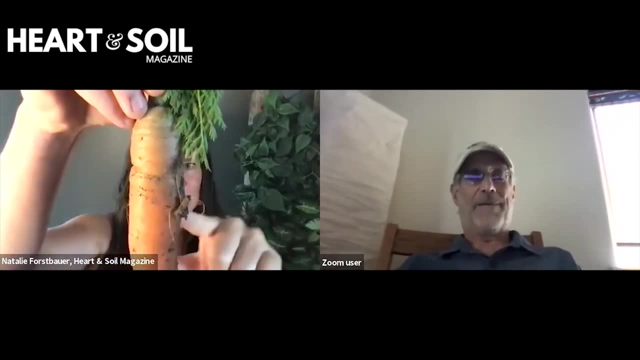 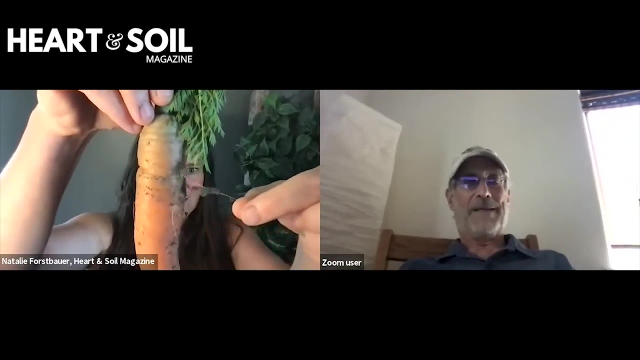 actually a farm like we're talking about, and so now we're learning that the bacteria actually enter into the main root system and then, after it's used, it goes. it's a, it's like, oh, i'm done now and i'm going to go back out, and that's when these little hairs are produced. and then 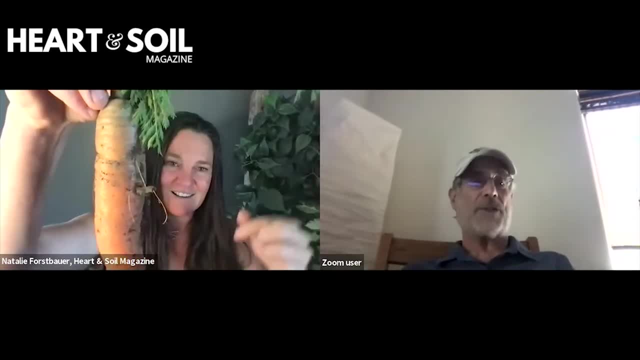 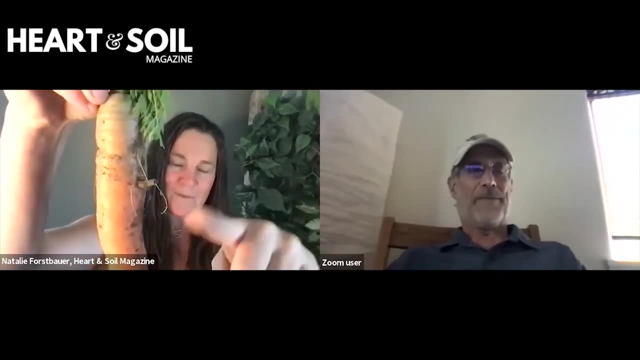 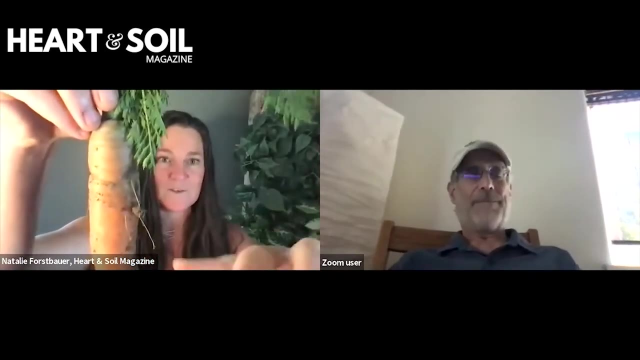 produced right, right and of course the hair stay. so as the plant grows, you know they're still functioning, but they're not functioning with bacteria in them. and then the bacteria come out back into the soil around the root and they replenish and rebuild themselves, and then they 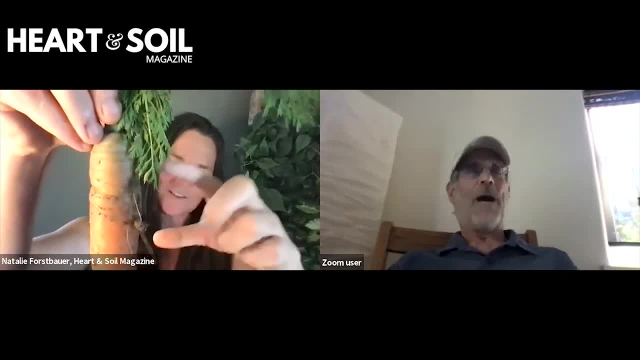 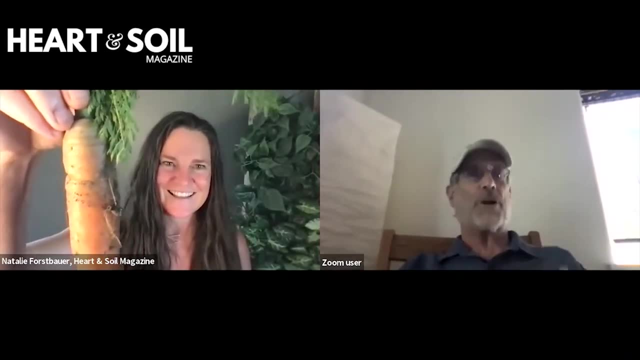 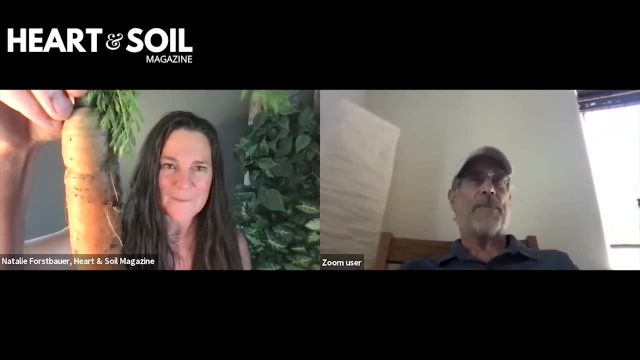 come back in and they're like: here you go, here's some more, some more good stuff. actually it's more. it's the plant goes. here you go. this is a terrific ride. you come in, come. you know the plant is in charge, not the bacteria. so it's not the bacteria seeking food, although you know why would a bacteria move inside? well, 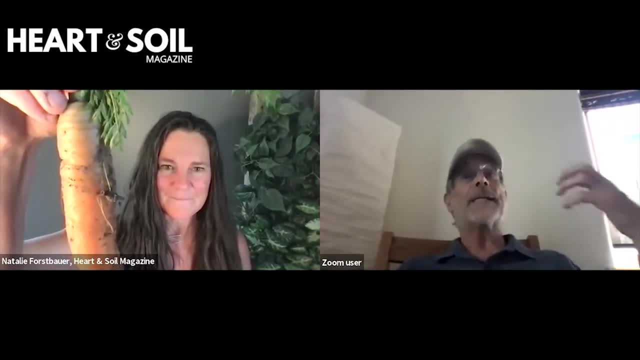 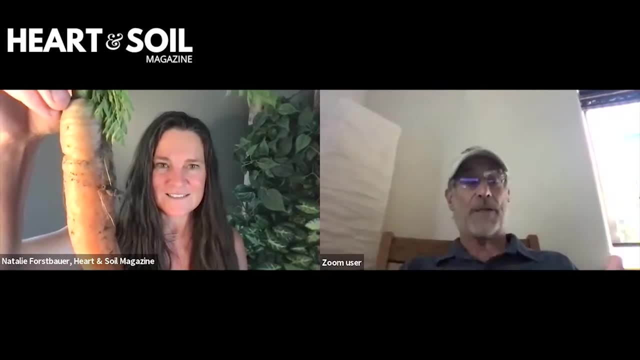 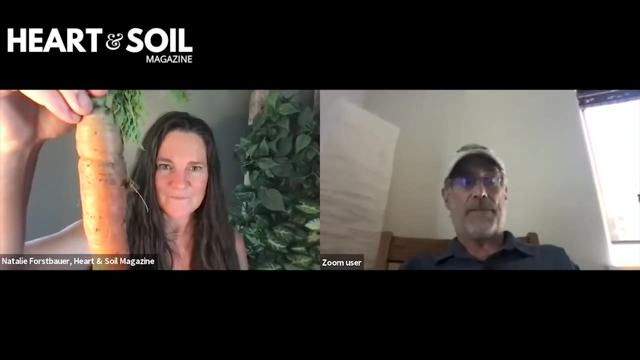 it's. it's got less competition, there's being fed, but it's the plant signal that makes the thing work. it's the plant that control, as it is with mycorrhizal fungi, as it is with rhizobia bacteria. it's the plant that calls them and sets out the signal right. so it's like: right, come here and 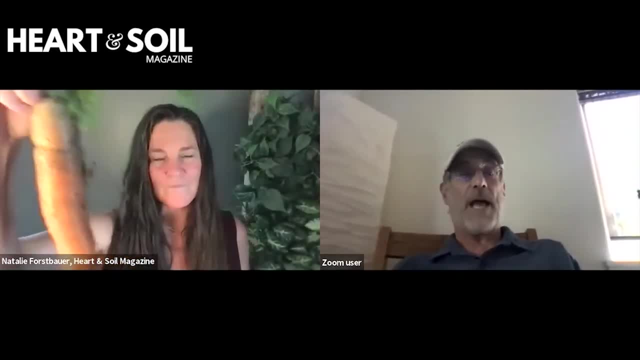 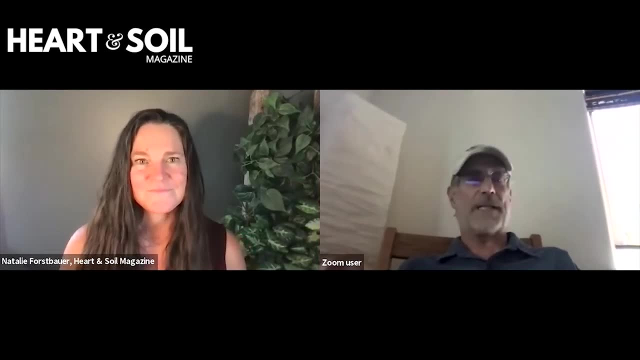 some of the bacteria. some of the bacteria are the same bacteria that are being farmed. some of them may be special bacteria that may be being taken in so that they can do various things, like sitaphores, that that that are able to throw out chemicals that tie up things that you don't want inside the plant, so they tie them up in the soil. 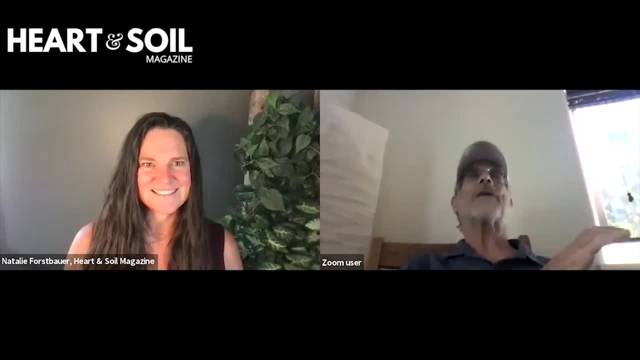 so it can't get in the plant. uh, you know, there are all sorts of these incredible things that are going on. and then these, the endophytic bacteria that are inside the plant, causing the plant to be able to grow, and they're able to grow, and they're able to grow, and they're able to. 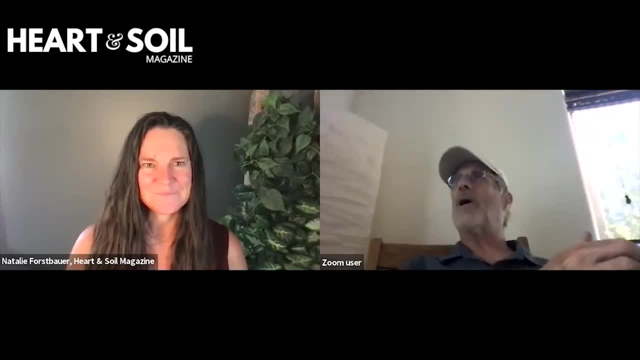 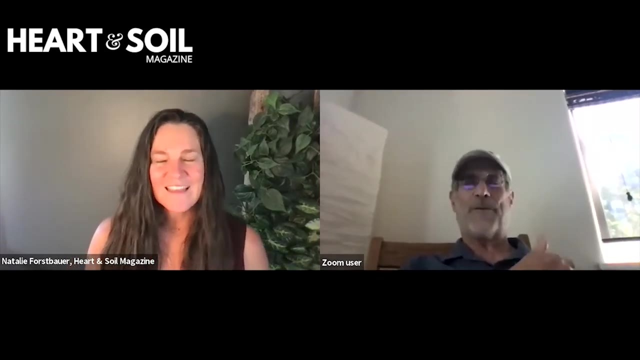 be able to withstand a lower temperature, for example, causing the plant to have a thicker or cell walls, a tree to have thicker trunk as a result of having these bacteria in there so that they can withstand wind better. it's unbelievable, the symbiosis between these bacteria and plants. 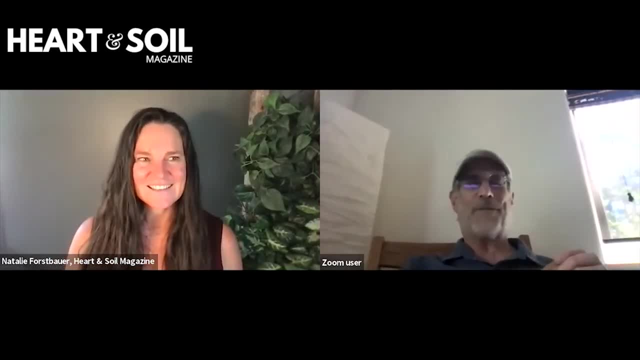 and not just little ones, big ones. it's fabulous, just fabulous, and so if you're a farmer, you got to figure out how to use this, how what. you know how to use all of the soil food web, obviously, but we have a new, little new piece of information here. it turns out that some bacteria benefit some plants and don't benefit other plants. so we need to be studying these things and figuring out what what works and what doesn't work. there is a different bacterial mix in vermicompost than there is in regular thermocompost. well, those bacterial mixes work. 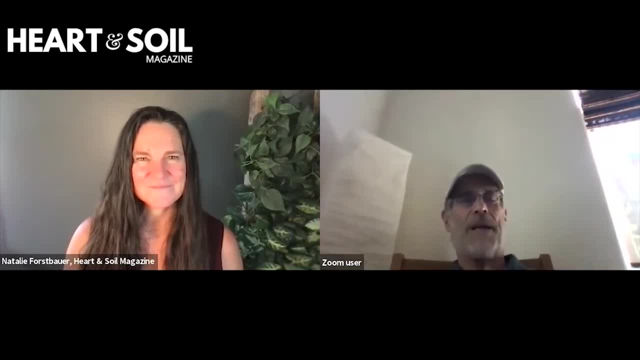 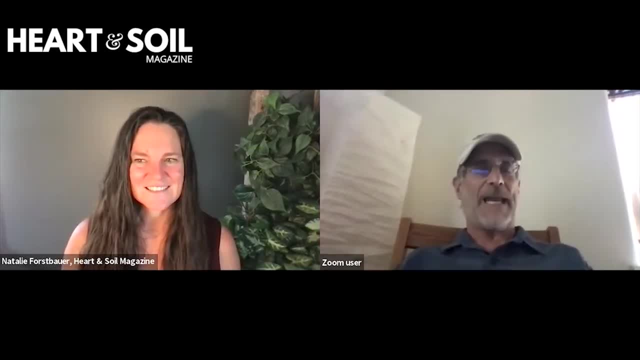 mean we already we're capable of sending in a sample and getting a dna. you can send in the sample saliva and get your dna uh. no reason you can't be doing that with. with the soil going to be cheaper and cheaper and cheaper. and once you get the right rna dna uh, you can determine what. 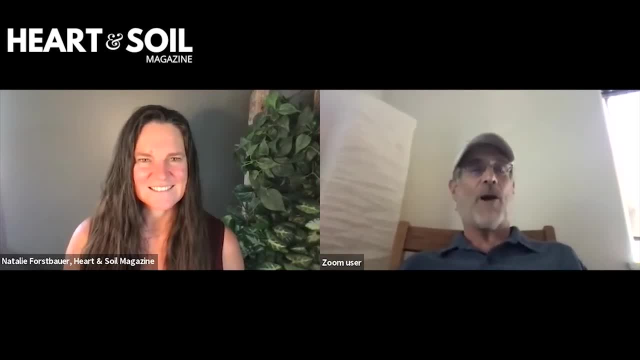 kind of back. you can already determine what kind of bacteria you're going to be using and you can determine what kind of bacteria are in your mix. it's just a little bit expensive. the databases are already there and it won't be long that somebody like dr judith you know, will come along and figure. 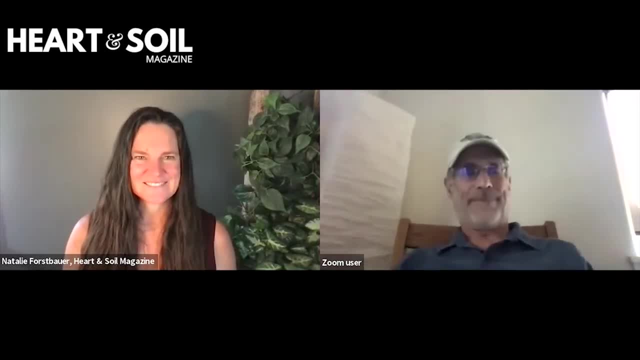 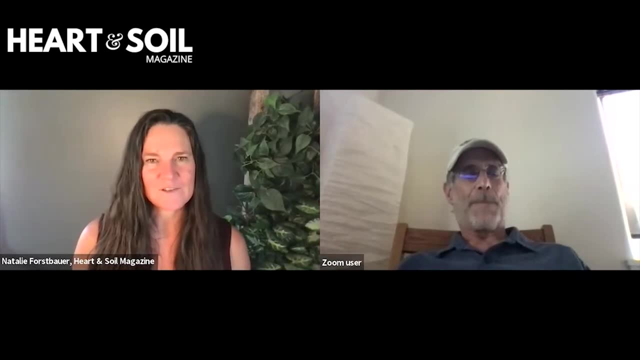 out a way you can point your cell phone at this stuff, and there you go. yeah, jeff, what helps feed the rhizophagy process? well, uh, you know, a couple of things are seem to be pretty clear. one is: when you use nitrogen- chemical nitrogen- the number of bacteria in the plant is lower, so you have a lower. 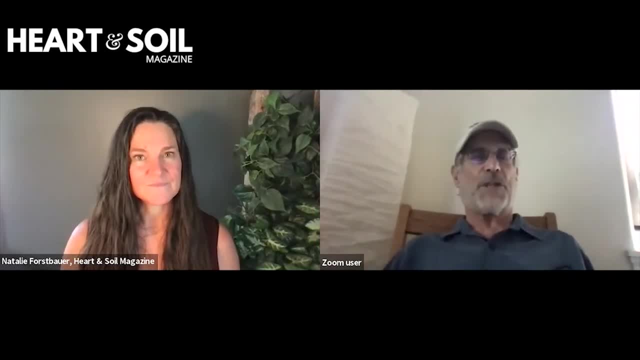 ratio, you know a nitrogen efficiency and you have fewer bacteria. so adding chemicals? we got another reason why using chemicals does not help the system, becoming pretty clear that when you add the chemical that doesn't mean the plant won't grow. you're adding the chemical, but when you add the chemical the night, the nitrogen fixation by bacteria goes way down and you're just spending extra money. well, that's not what we need to be doing and, as we said at the beginning, you're not creating soil structure that all bacteria that are in the soil help create soil structure. so it's very important that we keep these populations. we build these populations. we've discovered certain bacterium that definitely work with certain plants. you can begin to buy some of these now at nurseries, as a spirulium, for example. a lot of cannabis growers are beginning to use it. wheat growers use it. there's several different strains from brazil and russia. 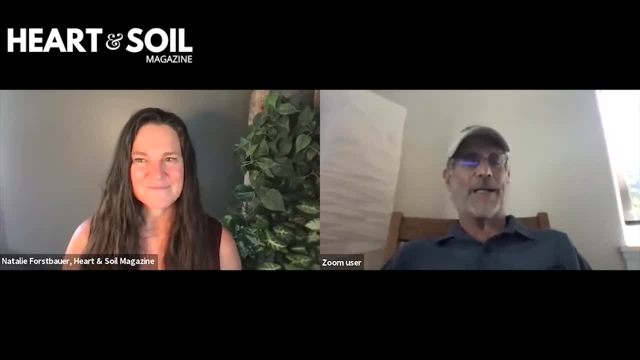 and all sorts of different kinds. so people are very cognizant of this. the big chem companies- you know the buyer and etc. etc. they're into it big time because this is a way that they can get away from the chemical stuff. that's not why they're doing it, because they're going to make. 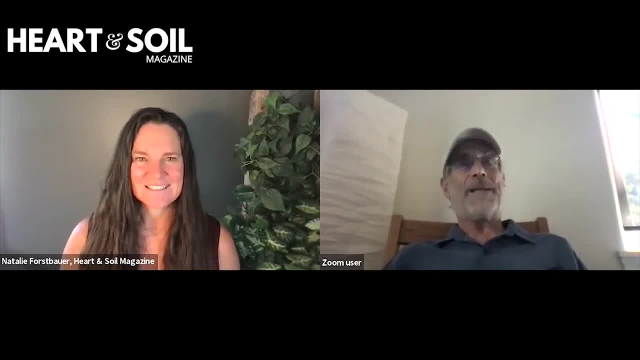 money, but the positive result may be: maybe they'll discover that glyphosate's not so good for bacteria and we'll stop using it. so, yeah, there's only good stuff that's going to be coming from all of this and how far we've come from the 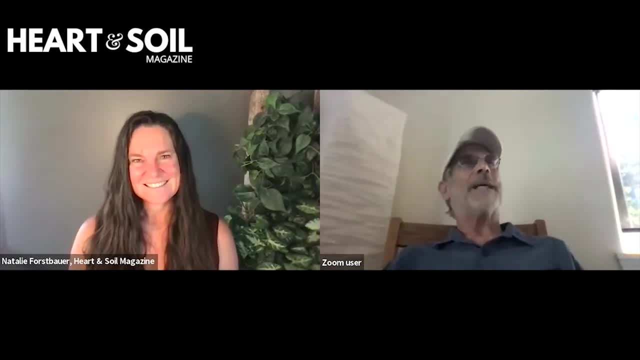 day i remember standing up with dr elaine ingham, probably 1996 or so, in front of 800 garden writers and communicators in washington state. we had our national convention and i said: how many people know what a mycorrhizal fungi is? and not one, not the new york times. 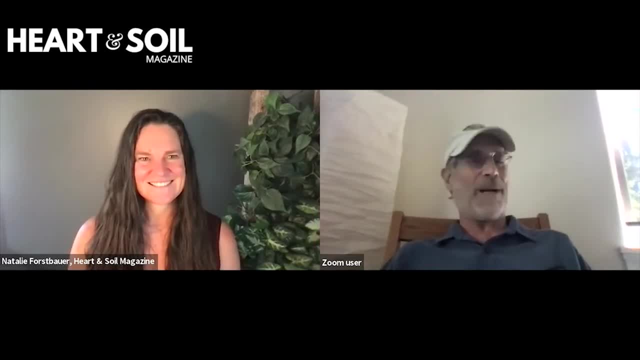 garden columnist. nobody raised their hand, nobody knew what they were. look at us today: unbelievable. so it's all going to be coming, and you know people like like dr elaine and judith and uh, and and james white and uh, as i say, all i do is report the stuff. i don't, i don't make these discoveries, but 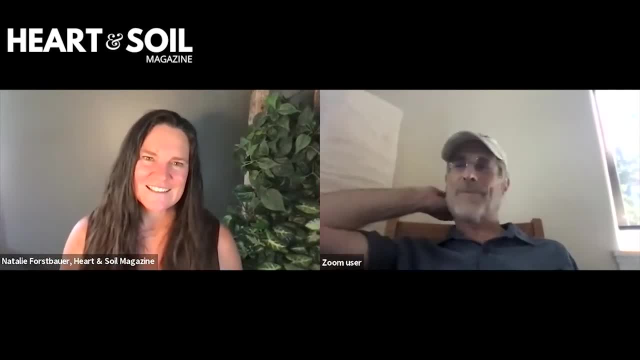 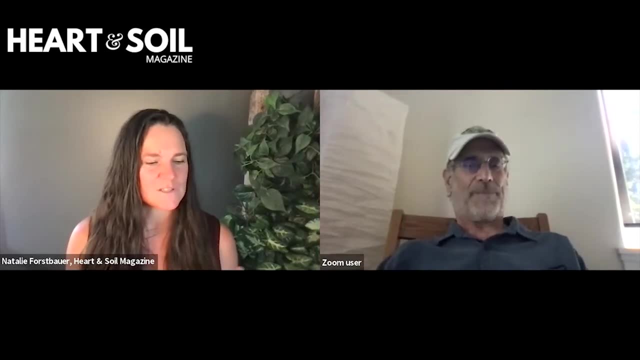 i'll tell you, there's a lot out there and people, really, you know we all need to go back to school. you know how? do you think the discoveries around bacteria and rise of hygiene are going to change the way we farm and the way we garden and change the world? yeah well, there's no question, we'll be. adding. i mean, if there's anything that's easy to grow, it's bacteria, and so we'll be doing specific research. what bacteria work best with strawberries? uh, and, and, and we'll be producing them because they're easy to produce. the problem is marketing them and and shelf space. some of them are. you know that you can produce them, but 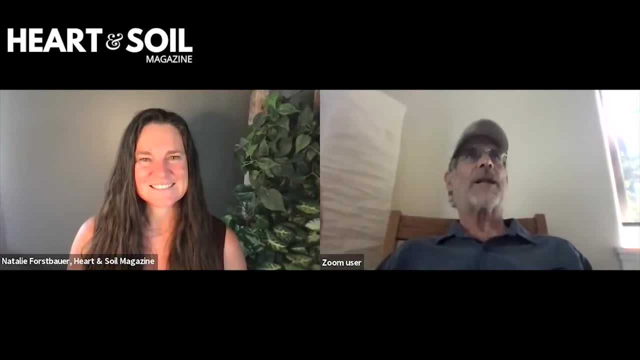 you can't sell them two years later, that's right. uh, we're gonna have to learn how to do these things ourselves and learn different vehicles for the carrying them and what. what turned into, you know, spores, instead of existing as live active bacteria, and all this stuff's going to be. 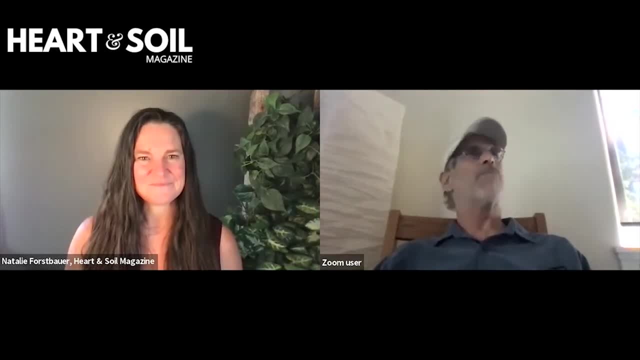 you know, i suspect there is a brand new area here. you know that we can, we can't, we can't even name of science, of how people are going to be treating this stuff, because it really is the answer, jazz, as were chemicals for a while. i mean they, you know, artificial. 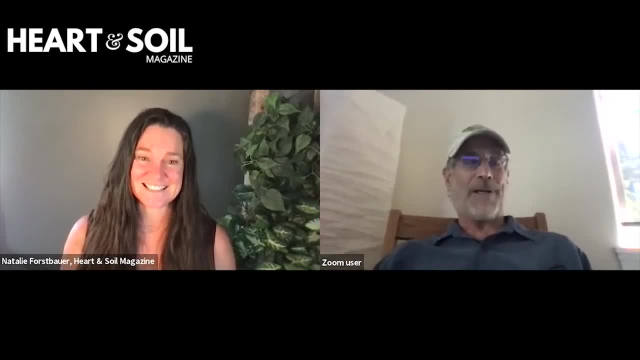 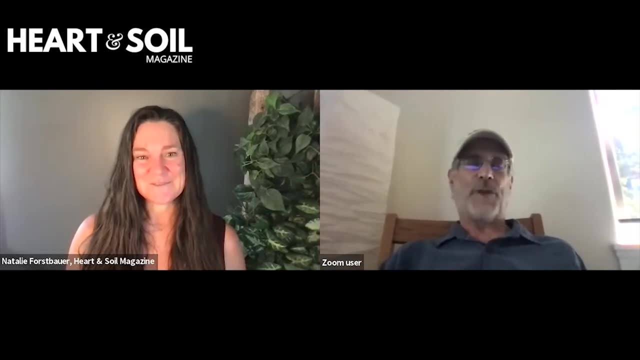 maneuvers is what they were called, and they worked, they were, they did. yeah, they realized. we didn't realize what they were destroying at the same time, and now we do. so there's no excuse for using them now. we'll go back and if it's the same companies, okay, you know. 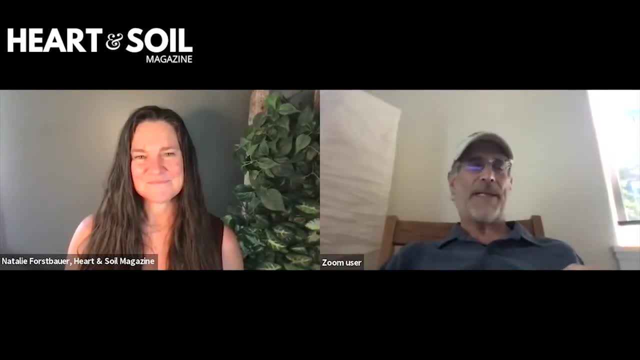 uh, they go back, figure it out. stop using the bandsaw stuff. let's do it the right way. so, jeff, how do we like? why? let me let me back up for a second. so when we think about bacteria- and i'm saying we, the general population, think about bacteria. 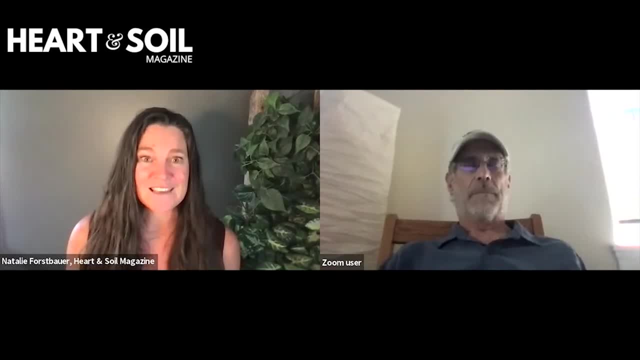 we're thinking anti antibacterial soap, we're thinking washing your hands as many times as we can and as often as we can, so we're not getting sick, so we're keeping ourselves clean, so our children are healthy, so our parents are healthy, so our grandparents are healthy. and so i'm wondering: 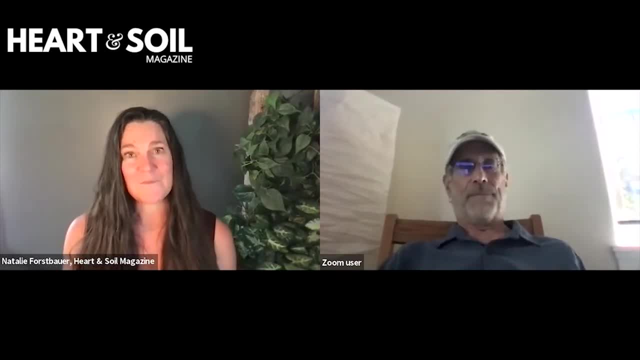 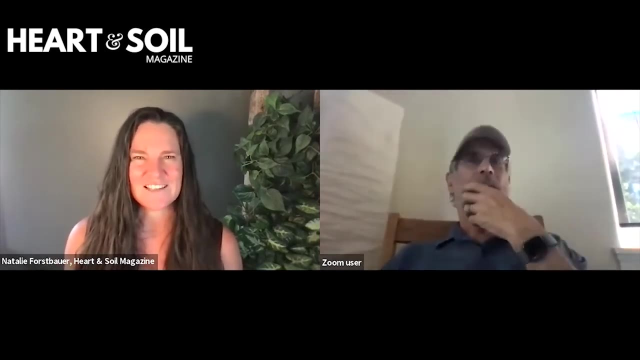 how do we shift from protecting ourselves from bacteria to understanding that bacteria have a really, really important place, because when we're killing the bad bacteria, we're killing the good bacteria, and so that, whether that's with antimicrobial soap or with that's chemicals in the field, how do we use that perspective? again, i mean, i was half kidding, but not really- we got. 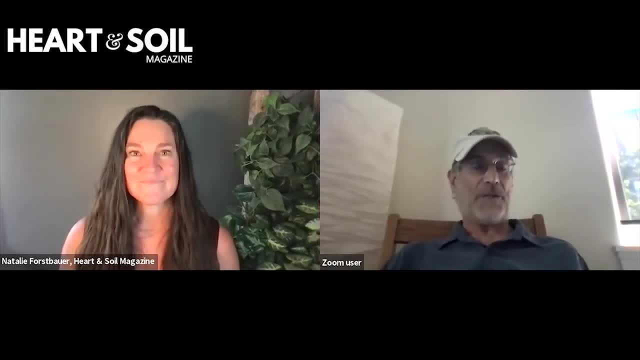 to stop studying dinosaurs at age six months, with plush toys moving them into books. their first books are dinosaur books by the time they're six years old. they can stay. they can name these complicated dinosaur names. there's no reason we can't be doing it with microbes that help us so that they understand. 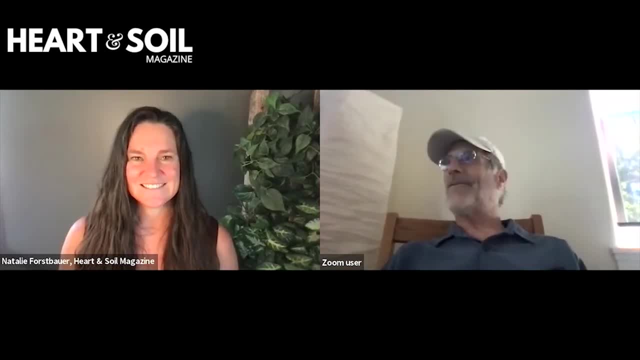 from age up. you know that it's fine. you know we're going to be getting things like fecal bacterial transplants. i think that'll change people's minds a little bit. um, and i think we just need to educate, educate, educate. i mean, you know, i always say half, you know you've got more bacteria. 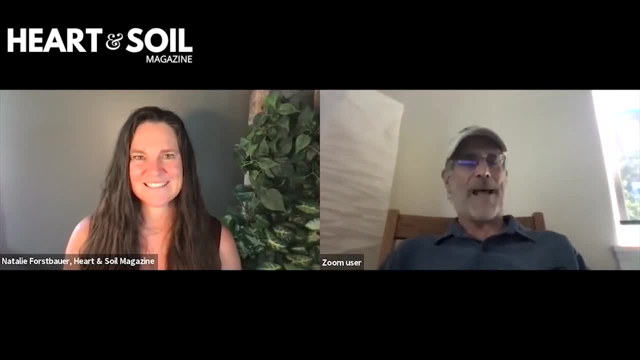 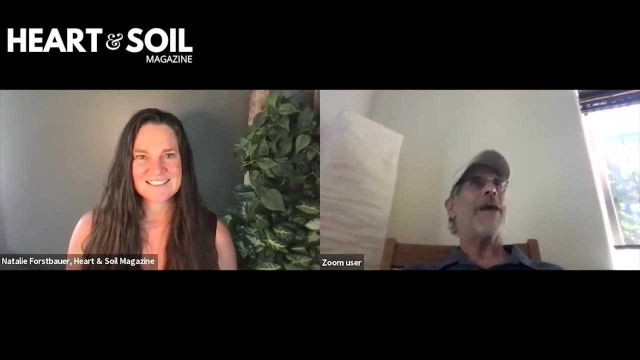 in your body than you do. human cells, blah, blah, blah. you know we're, we're getting it, and now that we've got a bacterial situation, you know where we've got to really pay attention that we don't overuse them, etc. i think people, people are going to start to learn about them. plus, now that we can. 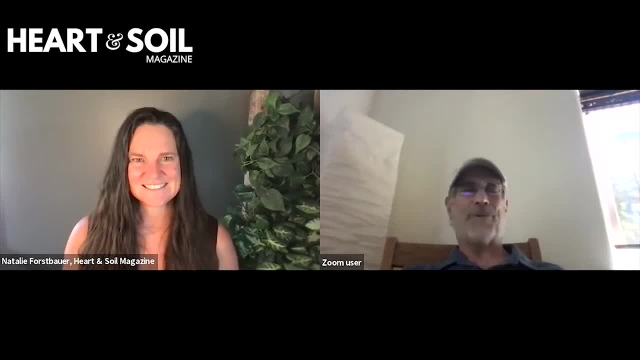 see them better with microscopes. it's going to be a completely different world, completely different world. well, you and i study. we're going to be able to see them better with microscopes. it's going to certainly what i studied in high school. i'm 73 years old. i studied in high school with these. 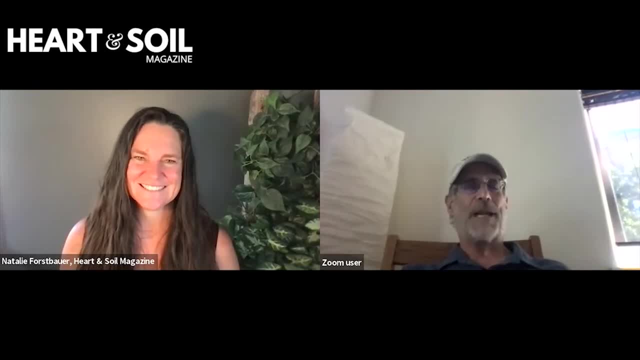 crappy microscopes. i mean, my goodness gracious, big difference today in hopefully more and more more places. so we just have to make sure people understand and when you go organic, people need to understand why they're going organic and it's the only way to do it. now i'm getting that group. 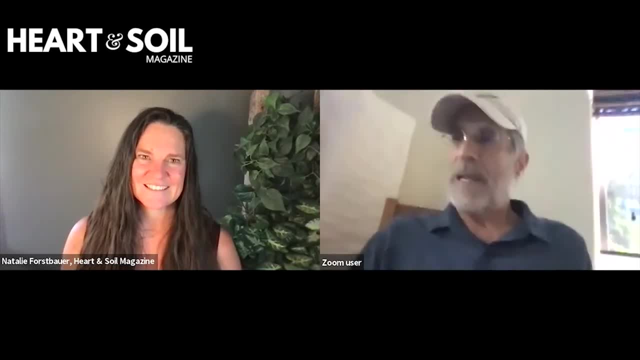 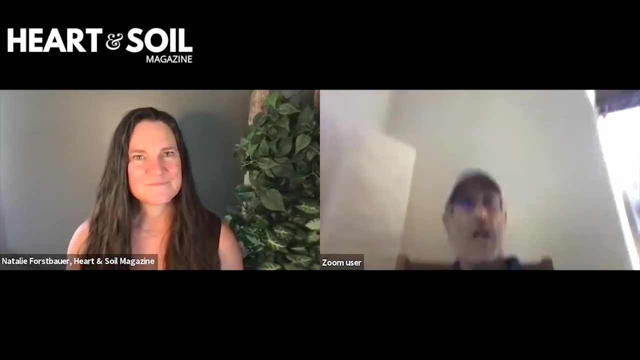 that we spoke to that lane and i spoke to out of those people today, garden writers- i don't know any, not one garden writer, not one that isn't fully organic, so fully eating organic themselves. they're eating and they're writing. wow, who i don't know? who you know? when was the last time? 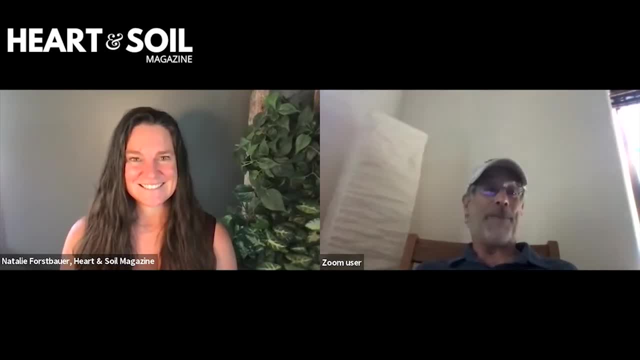 you read an article that said other than one that might have been a press release. gee, why don't you go spray, you know, glyphosate, uh, in your vegetable garden and kill all the weeds around your plants? no, nobody does that. you're not going to be able to do that. you're not going to be able to do that. 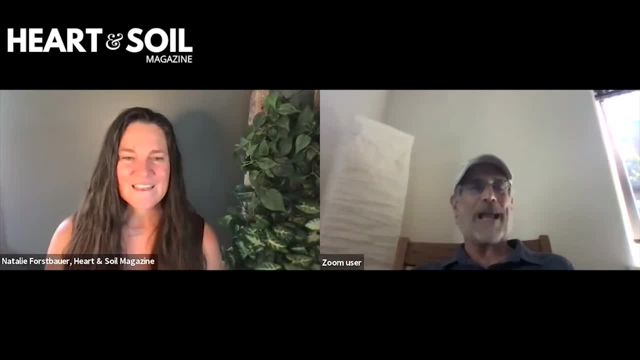 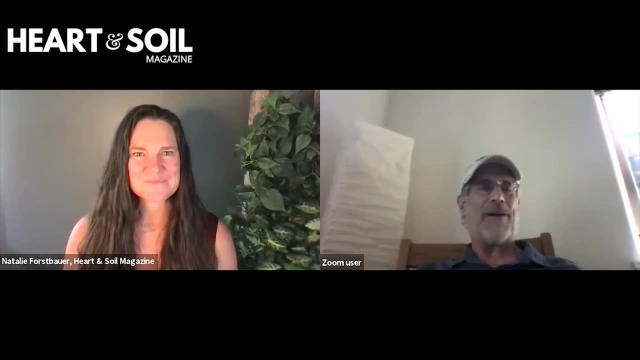 because nobody writes that way, because we're all organic. people do understand. once you're exposed to science- and that's what i try to do- it's the science. it's too complicated. often, because scientists are complicated, they have their own shorthand and, uh, you know, speak to each other. 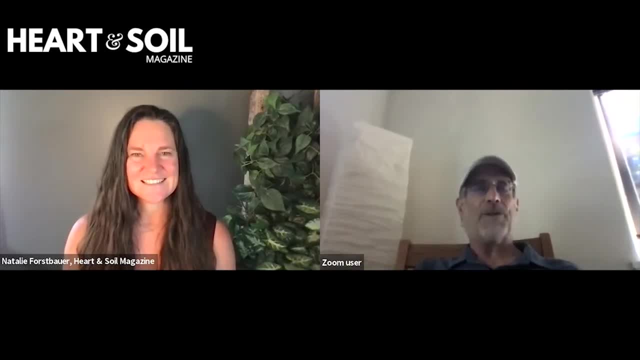 in a way that they can fully understand, and that's important that they be able to do so. but you and i, we need, we need it, we need spoon fit. that's yeah, yeah. so what do you say to a neighbor who is, um, you know, who is using something like glyphosate to kill the weeds? 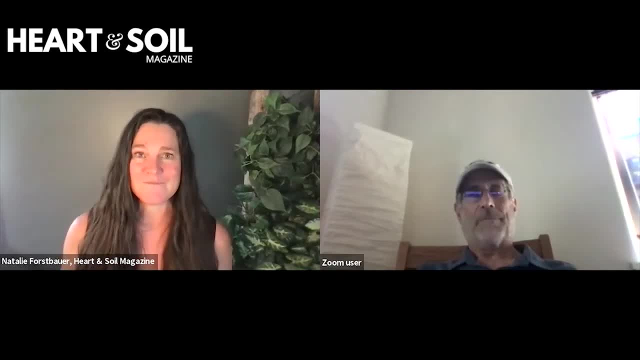 along the fence line and you have the conversation with them, how valuable you think organic is and you know they even are struggling with health problems and you can make the connection and they still are like i don't care, i want these weeds gone and this is what i know. where do you? 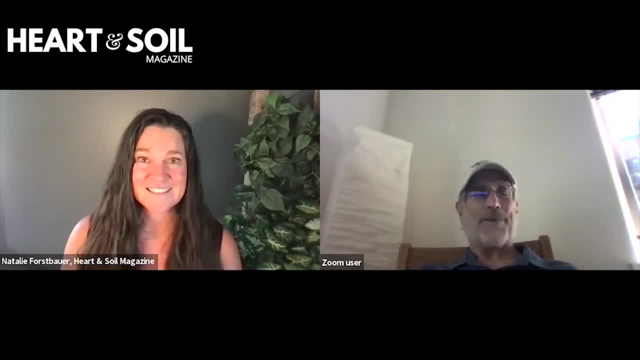 start with the conversation with them. well, you try to start nicely, trying to point out that anytime you spray it, you're not going to be able to do it. you're not going to be able to do it. you're not going to be able to do anything. it drifts, you know two miles, my goodness. you try to show them. 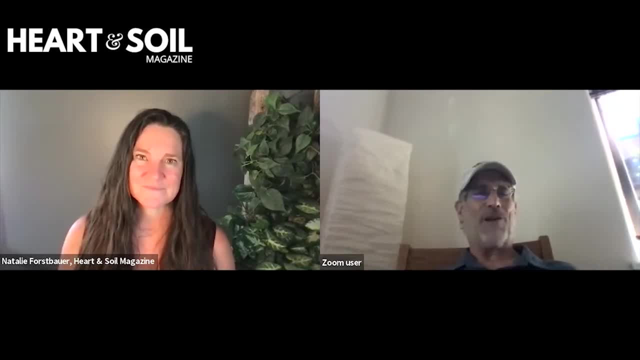 the internet articles about what the stuff does to dogs in long island, who you're living on the lawns of long island and you hopefully convince them. i've got i've got an ongoing debate with a friend of mine over glyphosate because we have a serious invasive choke cherry situation up in. 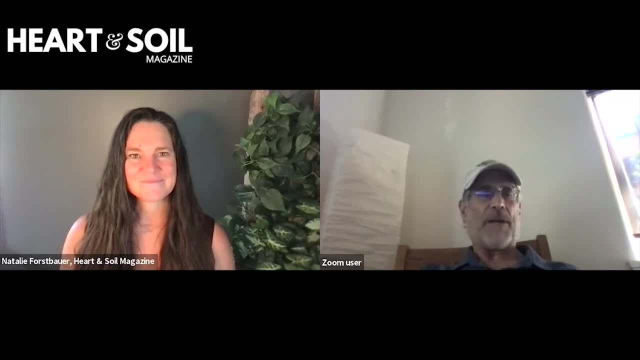 alaska. the birds spread on my crazy and they're taking over the riparian areas and we, you know fishing and salmon, etc. etc. and the he claims the only thing that kills the trunks into the is glyphosate. and i keep thinking, no, if you keep using glyphosate you won't figure out something. 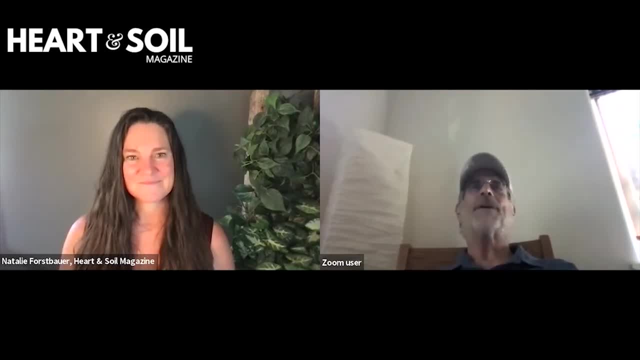 new, but it's. this has been a debate he and i have had very civilly for probably 10 years now, so you gotta try to be civil. it's not that easy. and if it's your neighbor, oh yeah, hard right, yeah, all right. curious: do you have any ideas about those choke cherries? i hear the same thing about mulberry. bushes? yeah, no, they're terrible and we shouldn't plant them. i mean, what we did in acreage? you know, i live in acreage. we plant them as ornamentals because they're beautiful. you know, when they're in flower and then the birds just go nuts and they seed everywhere, and so now we're pulling. them out. it's against the law to plant them, and there are lots of things that this happens. bayberry, you know also, barberry, lots of stuff. so yeah, uh, and, and hopefully, what we're going to discover is that if you change the bacterial mix, you can kill them, that you don't need to use glyphosate, and that's what's coming, i mean. 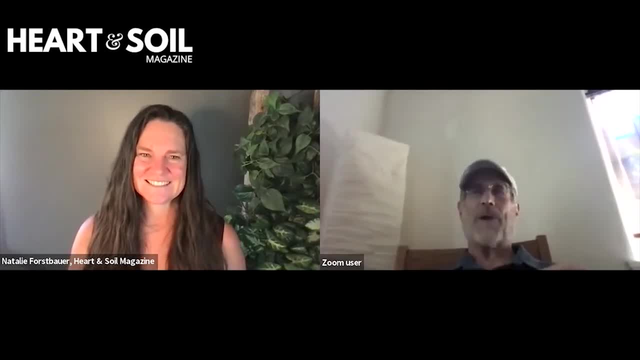 they're really the uh. you know i we talked about rhizophagy, but these endophytic bacteria, they're amazing, i mean they're. dr james told me about one that you put it on the plant. you plant the plant next to the weeds, they jump off the the plant you want and they kill the weeds. wow. 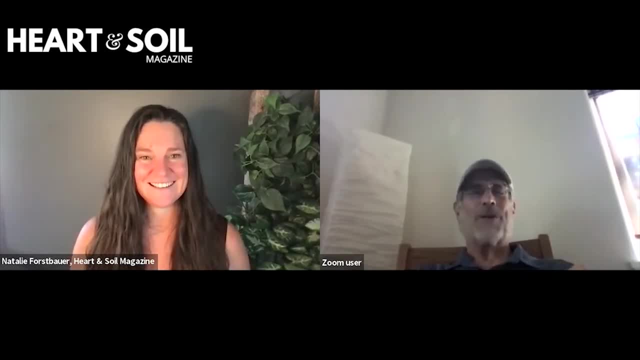 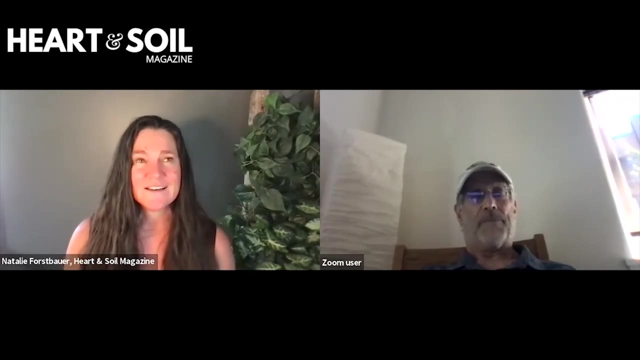 that's my, that's my kind of bacteria and so you know stories like that. people start to wake up and go: bacteria, not bad, that's so bad. yeah, it's really really powerful. because i, my parents, are organic farmers and, um, my brothers farm the farm now full time with my dad and and my dad was saying they 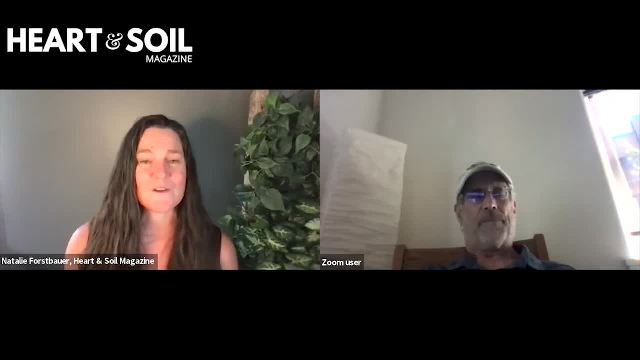 have such good, they've gotten such a good rhythm with their, with their fields, and they just they hardly have any weeds anymore compared to what they had, you know, even five or six years ago, and that's why they're so good at building the soil food web and uh. they become very good at composting and uh. 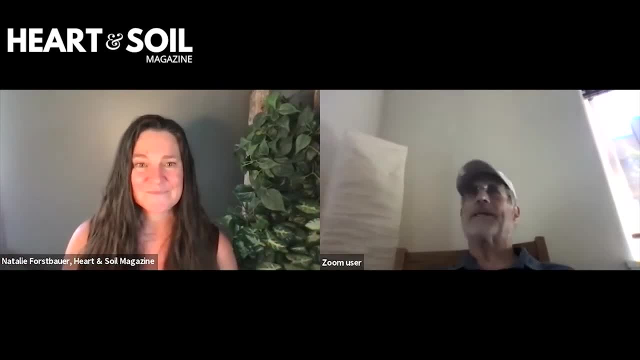 the weed pressure is way lower. yeah, i mean it. it is amazing, people. we've created this situation where we have to be those bacteria and those fungi at the bottom of the soil food web, and we're not good at it, so weeds develop, et cetera, et cetera. yeah, i, i, you know it's interesting. 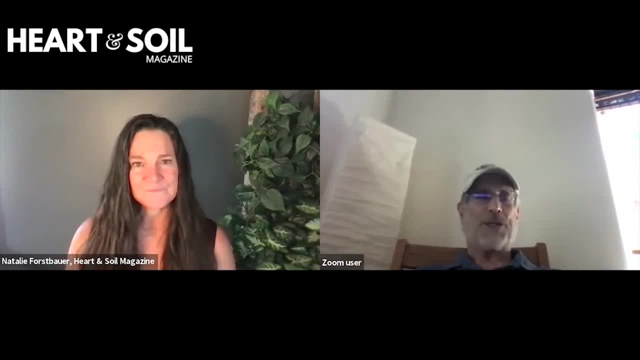 because the publisher- and we've talked about the quadrilogy, that's what four books- is known as a quadrilogy, also a tetra, tetralogy, yeah, tetralogy, i don't know um, anyway, the quadrilogy, and they keep them. you know? what else is there? and 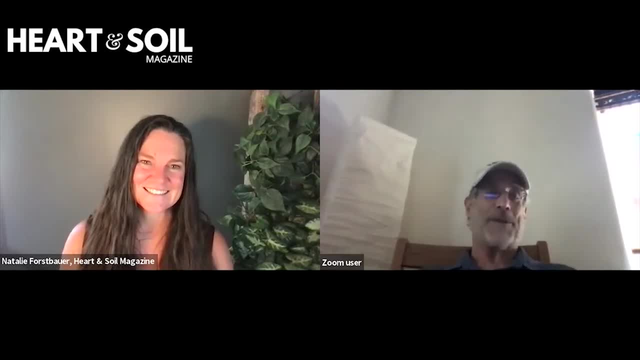 i can. i'm not so sure there is anything else. i mean, you know, i guess we could write about nematodes and and protozoa, but aren't we supposed to learn that in high school? it's these things that people just don't think about and they're so important. everybody gardens, everybody eats, and once they. 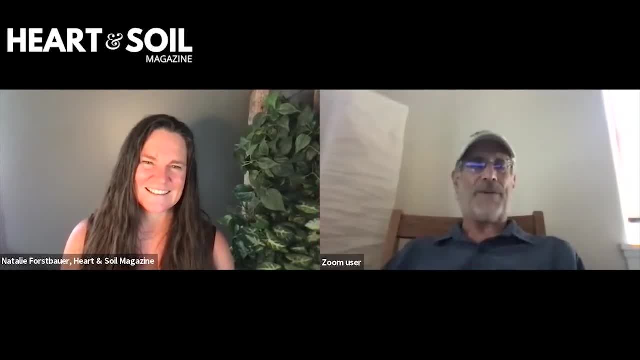 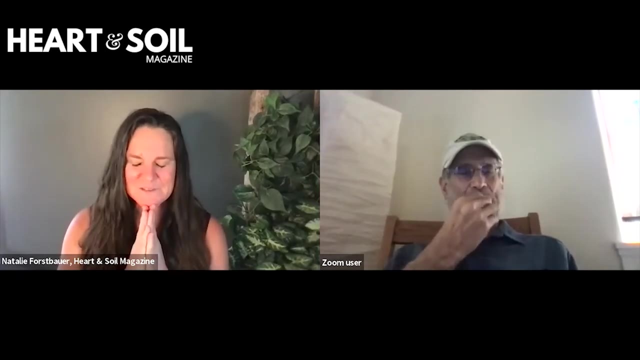 know, this stuff sure changes, sure changes the attitude. i can, i can tell you that there won't be. i think there won't be a cannabis grower in the world that sterilizes the seeds anymore. oh yeah, yeah, can i ask you about that? so that was one piece of teaming back with bacteria. that was uh. 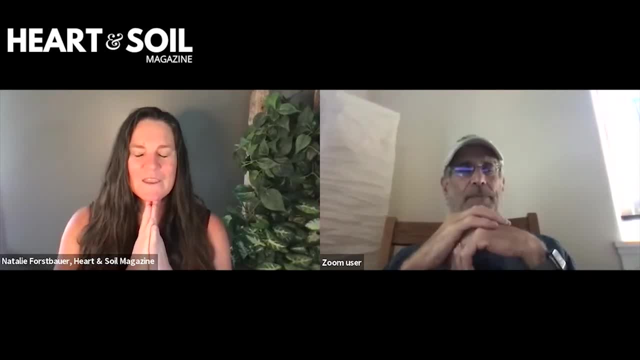 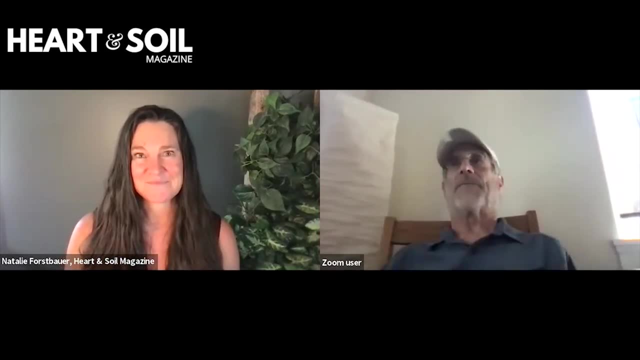 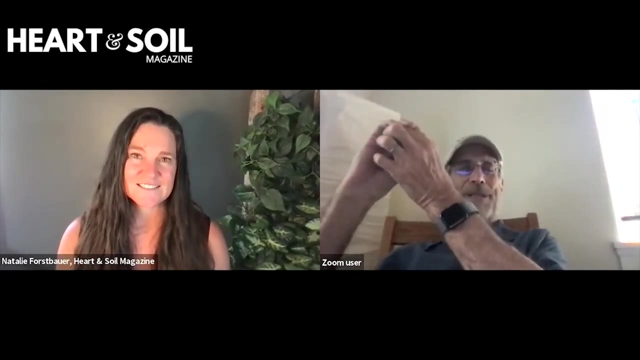 very curious and inspiring because, knowing what we're learning about bacteria, how will that change the way we save and harvest seeds? it's very important because, first of all, that these seeds, you know, contain everything that was inside that flower, you know, and they and they contain these specialized bacteria that keeps 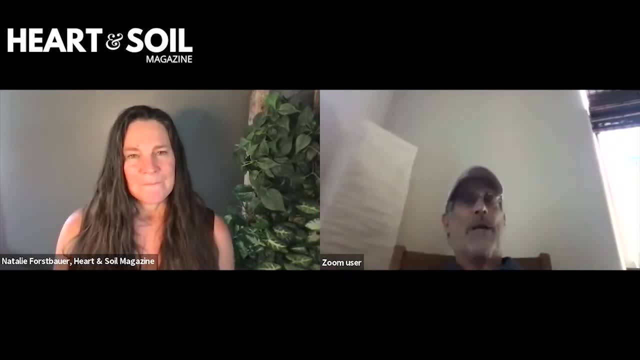 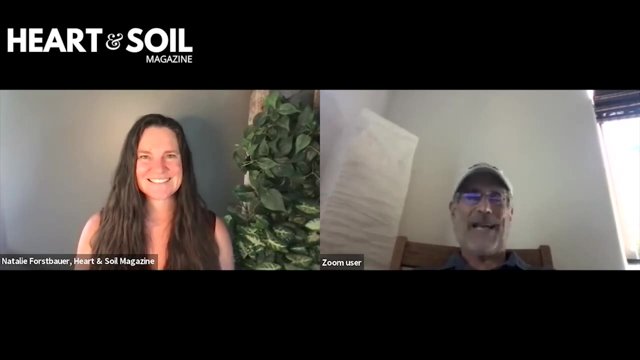 a plant strong, and will we now know that they're different for different plants? you know, for years and years in the cannabis world people were trying to develop terroir like we have in the grape world. well, it's probably not the soil. i hate to tell people. it's probably the bacteria that are in the grape seeds that are now in the 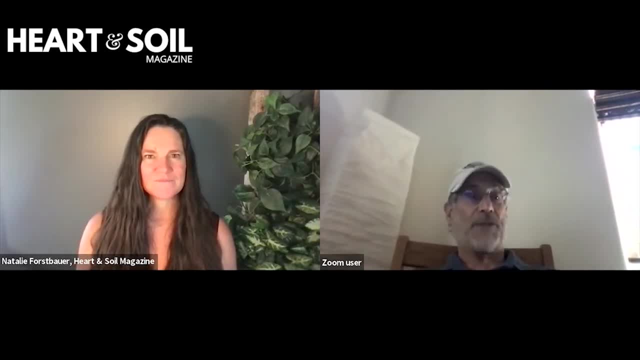 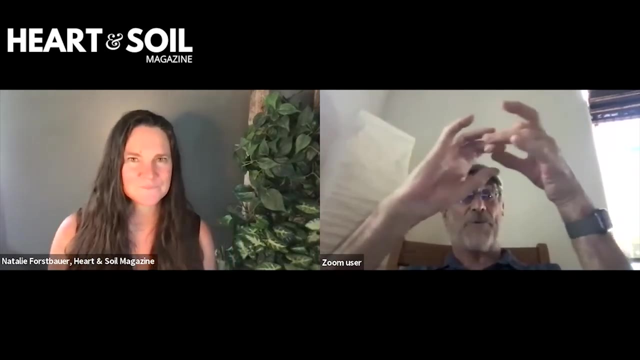 grape plants, because it certainly is so with regard to cannabis strains, the bacteria is what gives them their flavor, not the soil. it's very interesting: they speak in tric, they in the trichome, you know they're doing their little thing, fixing nitrogen, but they're speaking to each other in 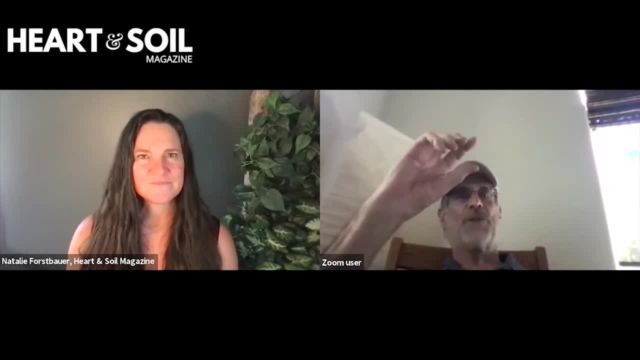 terpenes, and the trichome cell is producing cannabinoid in order to scavenge oxygen from around the bacteria so that they can fix nitrogen. you can't fix nitrogen if you have too much oxygen, and that's why those, those little bacterioids, form. 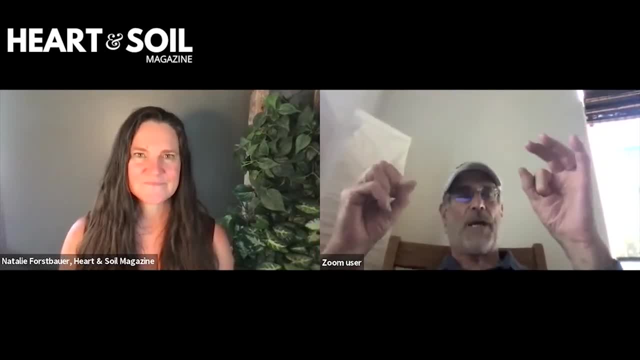 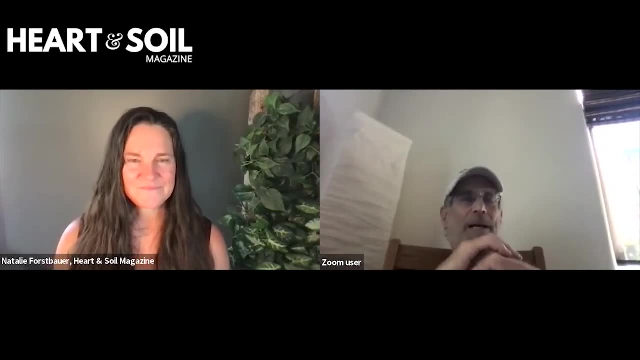 that little nodule that you see when you pull up a legume. that's, you know, to keep oxygen out, one of the reasons so you get different flavor based upon the stuff that's being produced by these bacteria. it's pretty amazing and, as i indicated, i mean a 400 year old corn has the same bacteria today that it had 400 years ago. that bacteria jumps off the seed and gets into the soil. so think about it if you- if you sterilize it you probably take- it's pretty hard to really fully sterilize a seed- got to use scientific chemical stuff as opposed to hydrogen peroxide, which is what most gardeners use: sterile soil. 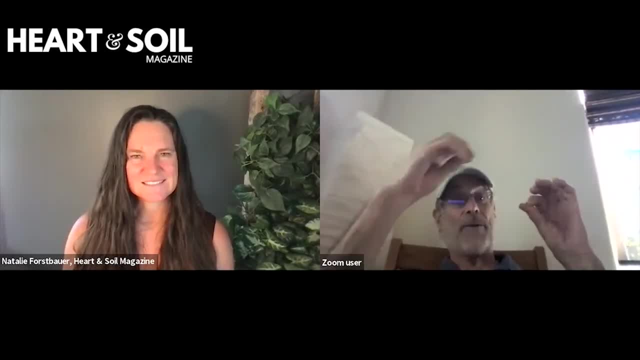 not as bad as sterilizing the seed, because the bacteria can get into the sterilized soil as long there's no sterilizing stuff there. a lot of people plant lots of stuff. they take a grapefruit seed and they'll put it into the napkin and wet the napkin and then wait for it to sprout and then 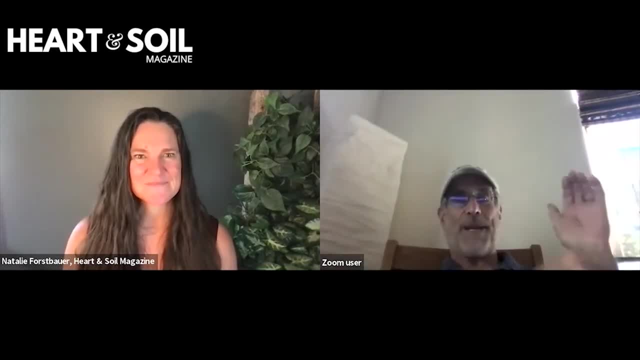 take the grapefruit seedling out and put it into the soil. wait a minute. the napkin's got all the bacteria that jumped off the plant. the napkin to use soil over again because it's already got the bacteria in the soil that that the plant needed and attracted and brought with it and it grew. 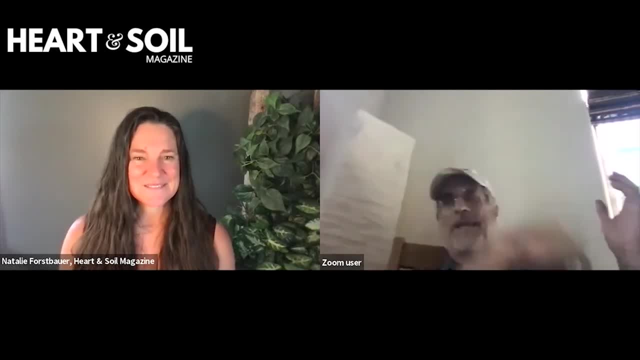 populations. and then you're throwing that soil out. oh, plant the same thing again in other than the potatoes which have a ph situation about them. yeah, it's, it's, you know. and then rototilling, you know, under the old soil food web system i used to say rototilling. you know, what's up here gets. 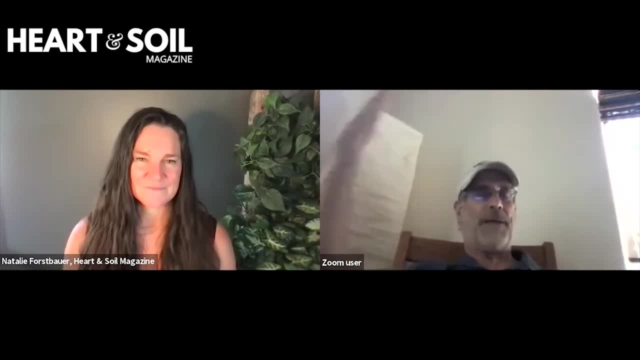 down there. what's down there gets up here. you mess up the system. well, these bacteria, you like to be in that little rhizosphere. so, yeah, all of this is just such key stuff that people just sit down and think about a little bit. and then, as i say, the the experimentation between vermicompost. 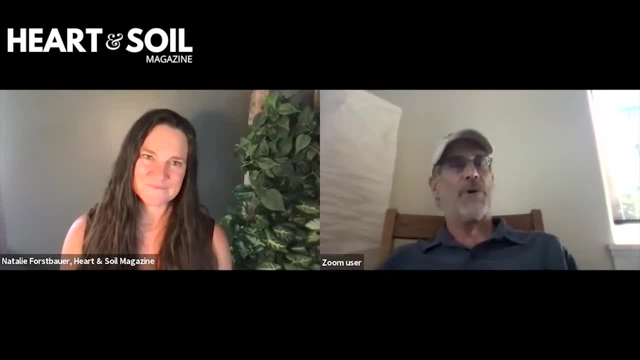 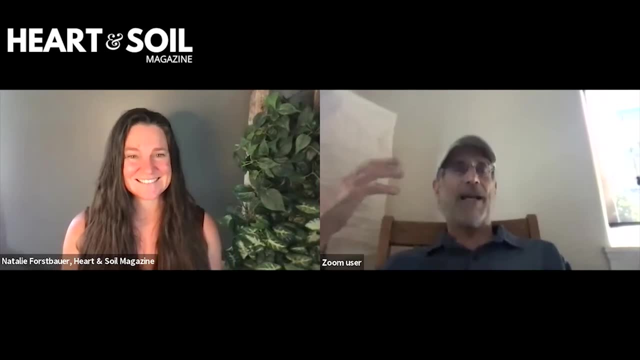 and regular compost and grass clippings, compost versus manure compost, and these experiments are not hard to do. i didn't have time to do it, but they will get done and we'll revise the addition and you know it's going to be important stuff. yeah, that's cool, but what are some of the other? 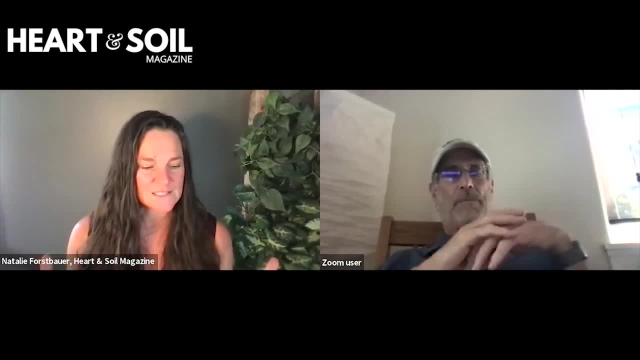 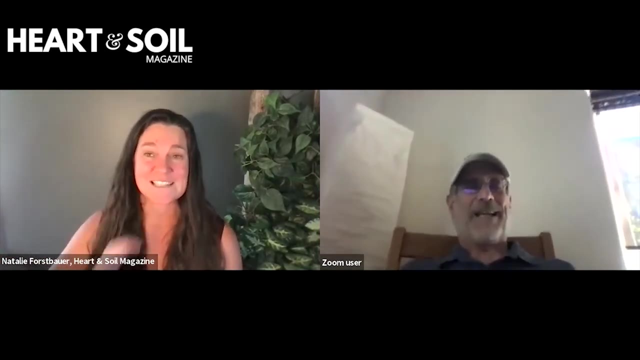 pieces of the changes. the way we might want to save seeds is: a lot of people think they need to keep their seeds dry, right, i never knew that people sterilize their seeds before planting. that is something i've been sort of sheltered from growing up in the organic space, so yeah, and i had no idea that it was a big. 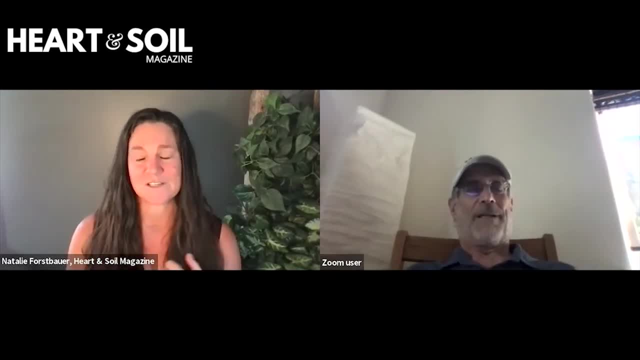 thing until i learned it was a big thing. so so, knowing to not sterilize their seeds, knowing to not like take all the moisture out of how they're stored right, they have to have oxygen. they have that moisture, and so what we've been told all our lives is: no, no, you don't have to have oxygen. you. 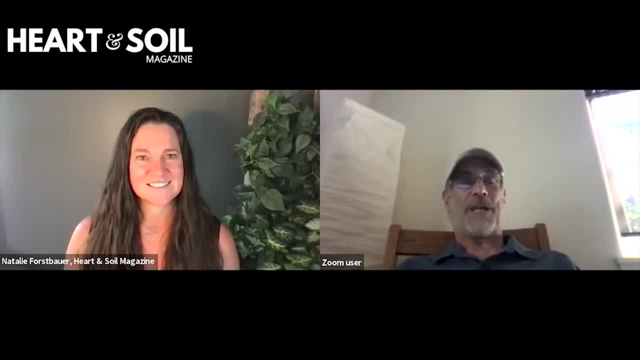 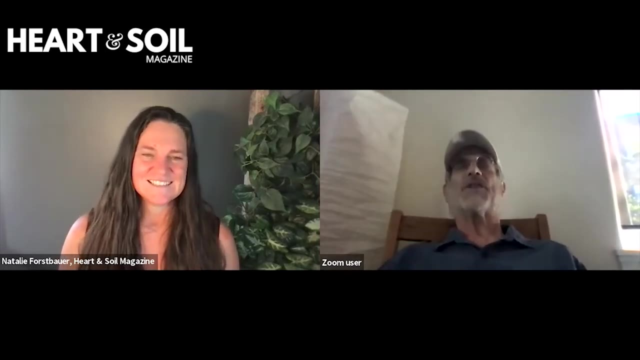 dry the seeds out, you know. you put them into a, you know, try to get as much air out of them. just keep them nice, you know, yeah, it is interesting, it's very different. um, yeah, it's fascinating stuff. and the pictures again. as they say, because of the way the staining works, you can stain for the. 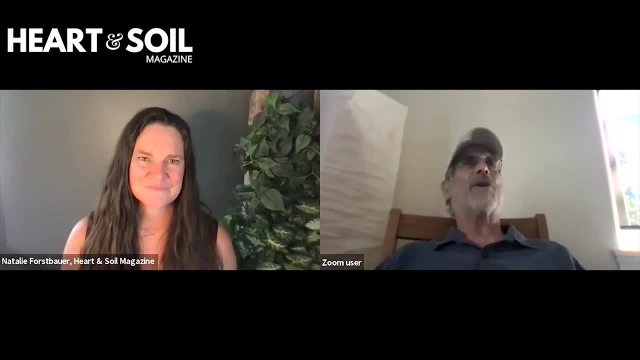 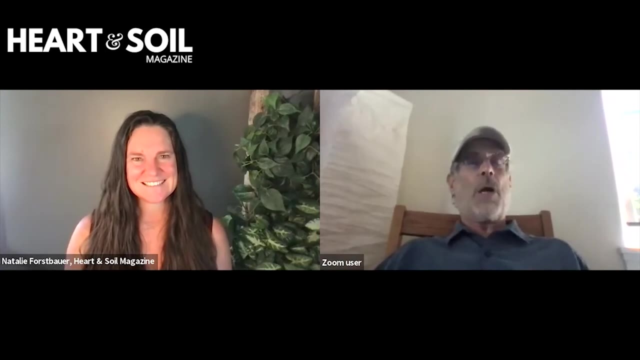 nitrates. you can stain for the carbon, you can. you can stain for the arginine, the exudate that's put out, and so the pictures that these students are getting are unbelievable and the advancements that are being made. i mean, when i wrote the book, the, the information about about trichomes was conjecture, probably about oh, 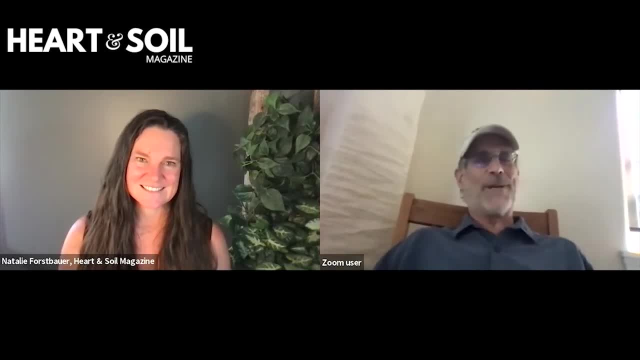 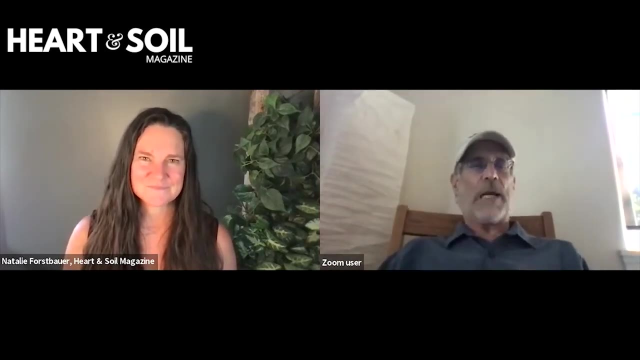 i don't know. i would say april of this year. no, it's not conjecture anymore. they have a proposed model. they understand how it's working. spectacular, just spectacular. so we're learning so much and- and as we started the, the talk about soil structures is being destroyed left and right by chemical farming, by mechanical farming. 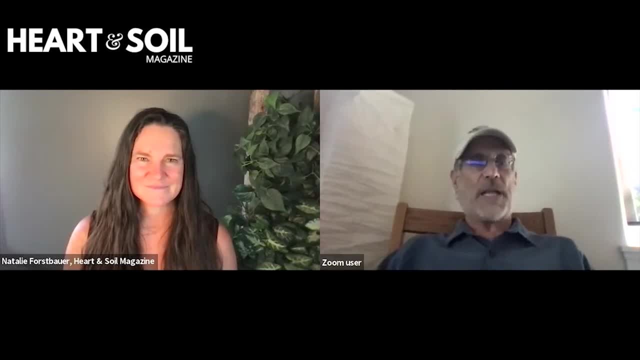 uh, where did i just read? in arizona, they just had a dust cloud. well, these things just don't appear out of nowhere. uh, you've had, you know, and during the depression, the dust bowl. that that's we. we. we have literally, they say, 60 seasons of soil left because it disappears, it blows off. we lost. 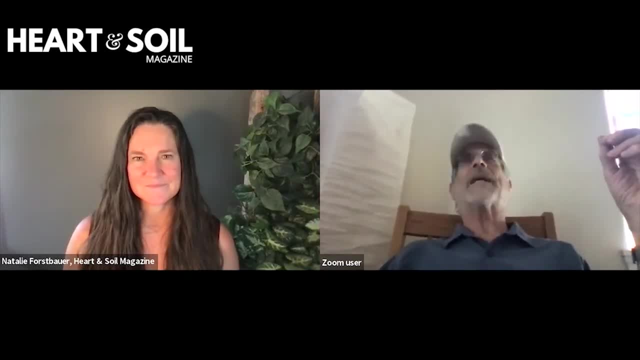 structure. so we've got to go this way, we've got to go this way. we've got to go this way. we've got to be regenerative in terms of respecting the soil food web and feeding it like crazy to make sure that it feeds us, because otherwise we are screwed. simple as that. two more questions. do you have time? 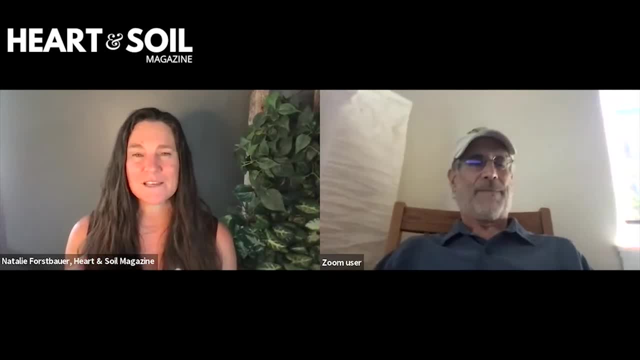 yeah, how do you see bacteria playing a role in cultivating health, personally, for humanity and globally for our planet? well, i think we've discovered that when you use artificial fertilizers, nitrogen in particular, we end up with less dense food. the nutrient density of a salad today is compared to 1945. you know, like drinking gin versus water. i mean, it's got nothing in it and that's because we use these chemicals. we know that that when you stop using them, the bacteria increases. the bacteria feeds the plant. the bacteria operates the plant the way it's been operating for eons and eons. it's. 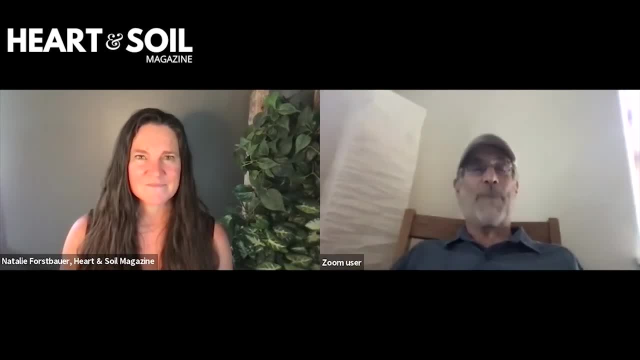 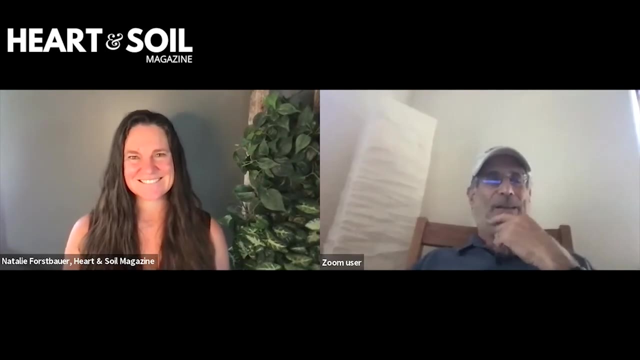 been a system that's provided us with nutrition until we broke the paradigm after world war ii. so it's going to bring us back. no question, it's going to make food much more healthy. plus, you know, we're learning different ways to grow bacteria when you think about it. uh, those um burgers that are not meat. 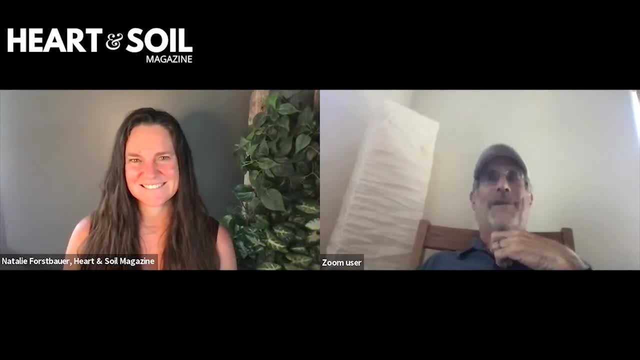 you know, those are all. those are all made out of bacteria and it's going to be terrific. so we're going to. we're going to find some interesting stuff. it's going to be. it's going to be great, but the the density of food, i think, is going to get much better. the bricks is going to. 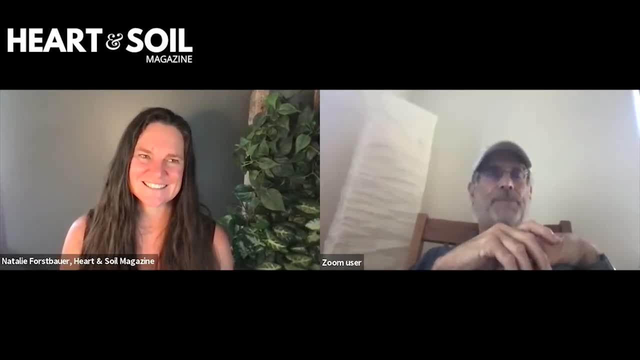 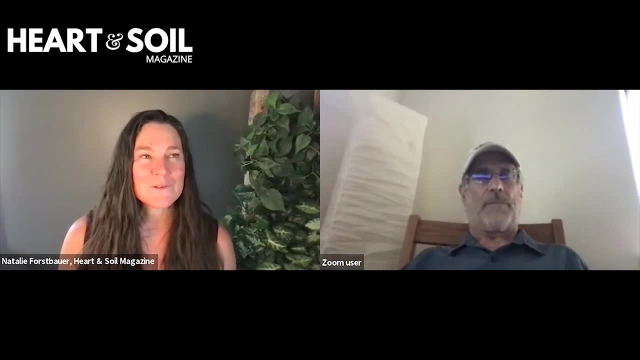 go way up. we're going to have much better food again. that's awesome, that's exciting, that's really exciting. and what about? what's something that people don't ask you about that you really want people to know about? you know, of course, this has sort of been a theme throughout all the books. the 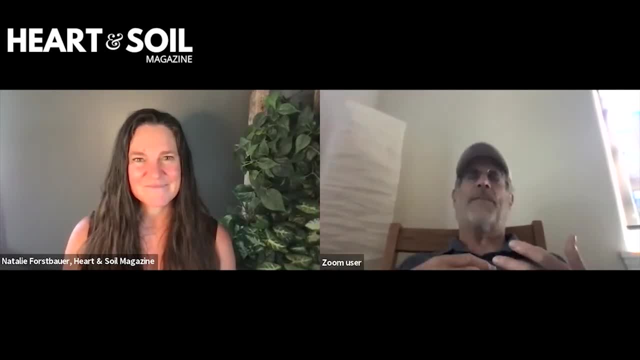 quadrillionaire and really people ought to read them all. and i always tell people it's, it's not me, it's not my writing, it's the subject matter. you have to understand this stuff, otherwise you can't be a good farmer, gardener, grower. you just can't be. and and the time i always tell people you buy. 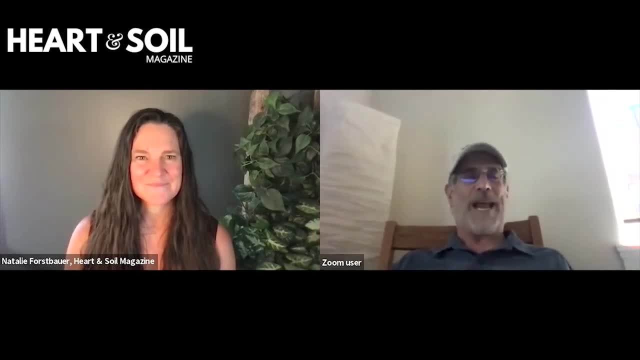 teaming with microbes. if you know nothing about this stuff and read it and don't like it, i'll buy it back at three times the price. no one's ever taken me up. i'm always worried. you know the homeless person's going to walk in 10 000 copies, but uh, it's it. it's just such eye-opening stuff and it's. 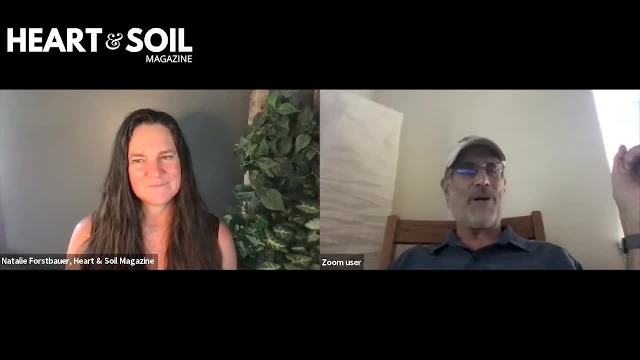 so important. it's just so so important. so i i i always get into the metaphysical side of it and nobody ever asked me about that when, when i wrote teaming with nutrients, for example, it became pretty clear to me that you know, we're just like a plant cell, we're enzymes talking to. 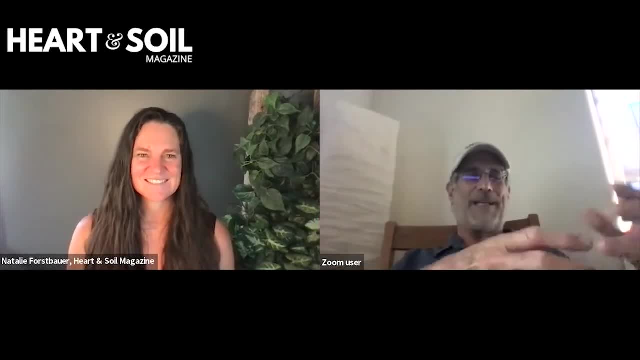 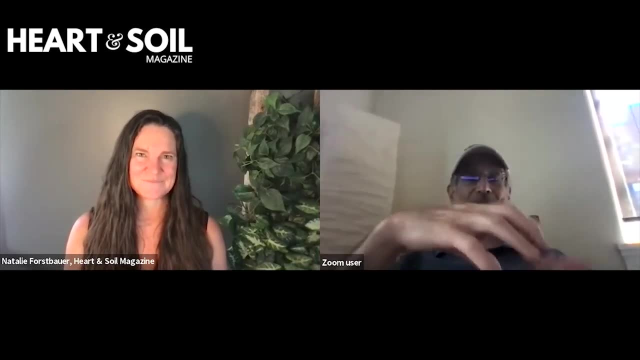 each other, fertilizing the, you know, making something. uh, a new idea is going to come out of this and uh, you know, it's just horton. here's a who kind of stuff. you take that cell, it's just the world. so fedex is just like the endoplasmic reticulum and it distributes stuff all around. 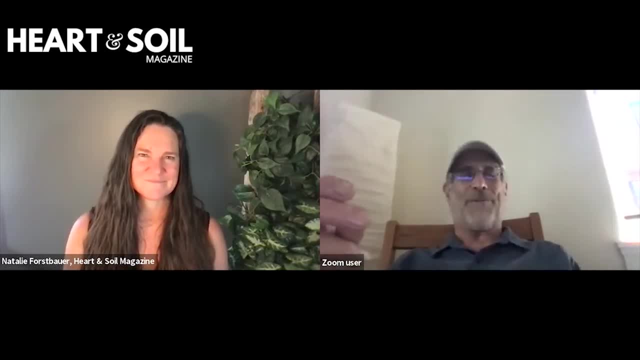 the world and you know it can move it out anywhere it wants to. and it's just mind-boggling the connections between. but when you get down to bacteria, when i see pictures of bacteria versus pictures of space, these new pictures that we're getting from the new satellite- oh god, the similar. 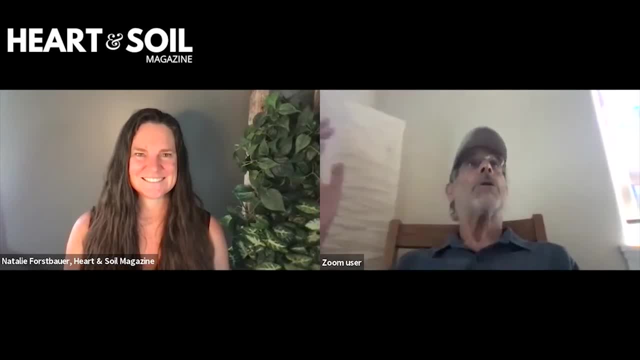 it is freaky. some of these nebulae look like the bacteria that i was writing about in teaming with my with with the bacteria. how can that be? they're identical. in fact, the last page of teaming with nutrients, i think i have a picture of space and a picture of a cell. you can't tell which one is which. 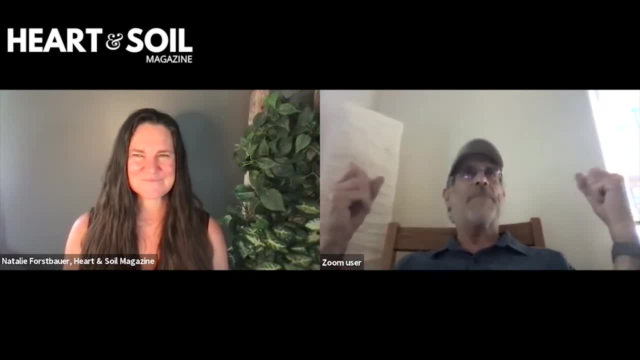 it's unbelievable. it's unbelievable, and so the metaphysical of all of this, i think, is important for people to get into. we think plants are these dumb, inanimate, can't run away, objects that sit there and take it. no, they are sitting, they are smart, they are active, they are doing stuff. 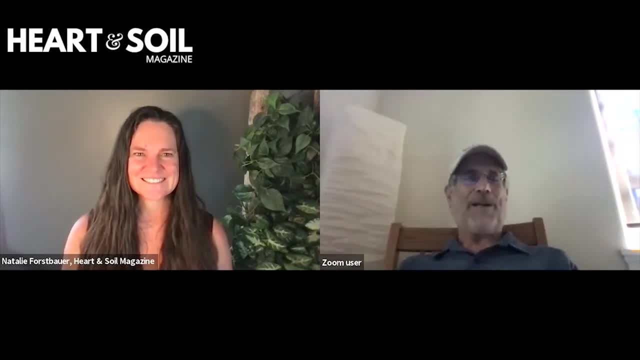 and we need to respect them and learn to work with them. period, that's powerful, and why is that important to you? well, uh, you know it's it. it makes us just part of the system, not in charge of this system. you know, gardeners always think they're. 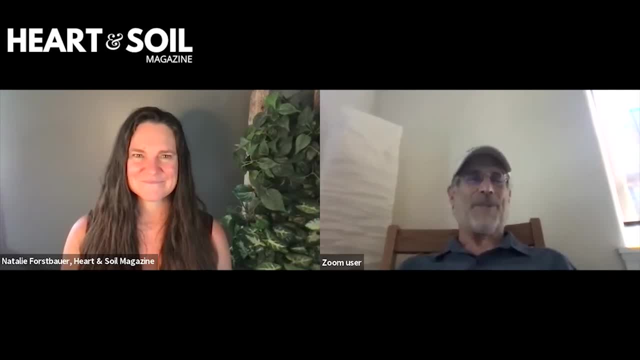 in charge. no, we only mess stuff up. we're just part of the system. we can bring water to the garden, you know. we can put it on the plants, we don't have to do anything else. you know, if there's enough organic material in there, the plant can take care of itself and we can bring water to. 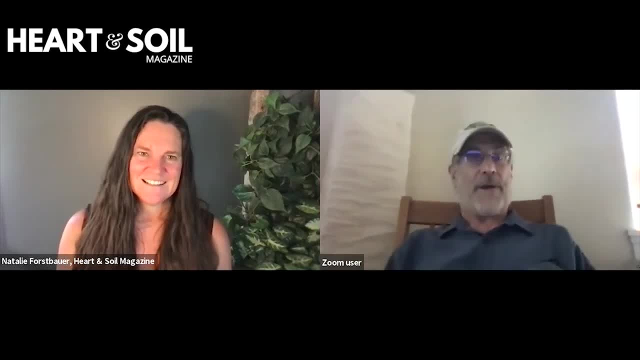 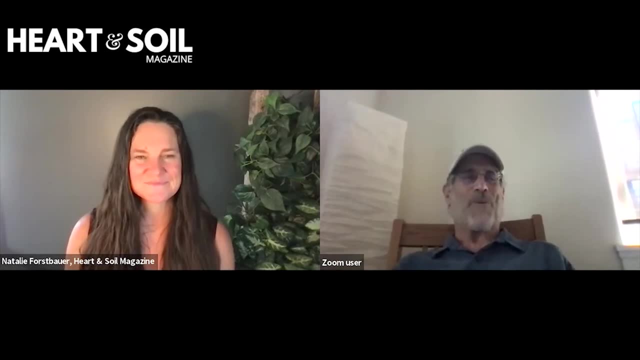 itself. you know, there used to be, there used to be arguments people would have because i think i- and i always hate to do this- well, i won't, i won't even do it- there was, there's, a famous person that people put words in her mouth, uh, and she basically said: you don't need to fertilize, you don't need to. 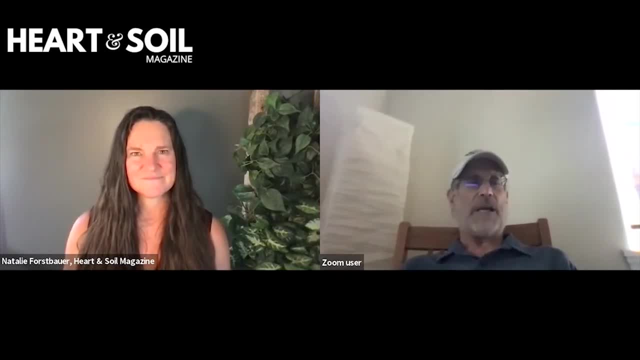 fertilize. if you provide organic material, you never need to fertilize. and she's right. you don't need to fertilize because we've got these microbes doing all this stuff for us and and we're just part of the system- we're just part of the system- we like to get in there and destroy the system by taking it over. 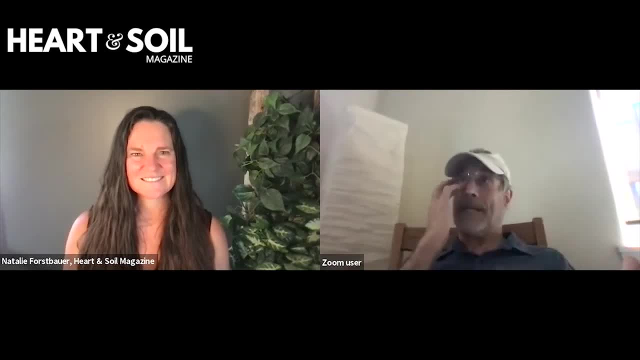 so it's important to to get into the metaphysical side of this stuff and to appreciate, wonder and be part of it, because it's really quite incredible, agreed and aside from expand, like deepening into that and expanding our awareness into that, like you so beautifully named. 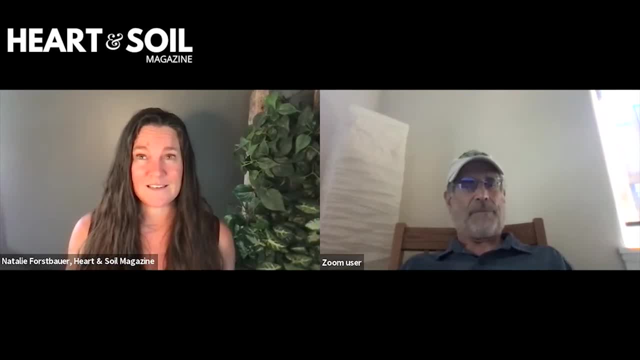 how else can we deepen into that connection and knowing that we're part of the system and not separate from well? i mean, you know, we used to just talk about the soil food web and then people started talking regenerative uh, which which is really still a soil food web. the difference is it includes not. 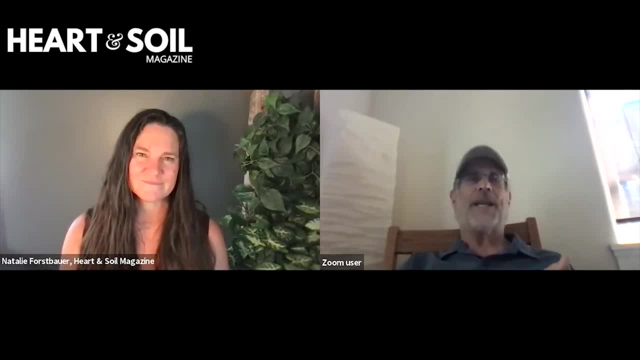 just adding organic matter to the farm. regenerative farming also includes treating the people who work on the farm properly, you know, treating the people who buy from the farm properly. so you know, we've got we've got a lot of people who buy from the farm and we've got a lot of people who buy from the 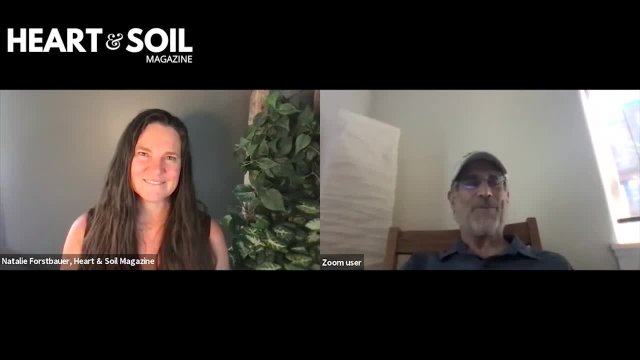 farm and we've got a lot of people who buy from the farm and we've got a lot of work to do to become like sort of a united system where we're all part of it, not just the gardener is the boss, right? so it's actually really deepening into personal self-awareness, oh yeah. 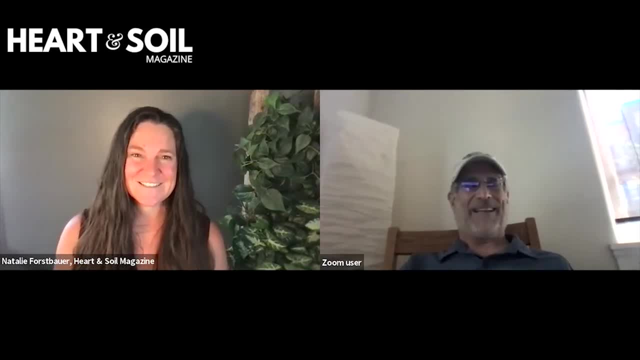 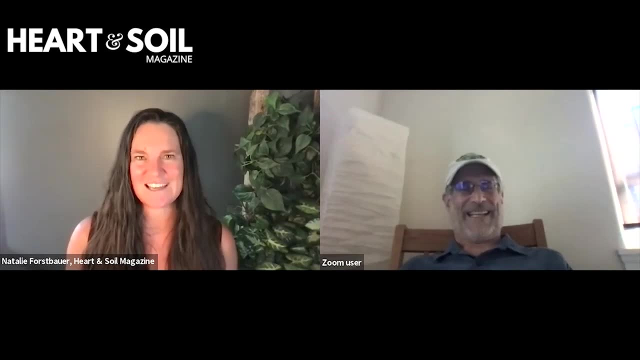 sure, why not? why not? yeah, awesome, powerful jeff. thank you, jeff. tell us where we can find teaming with bacteria and all the teaming books. right, you can find them at amazon, for sure, all good bookstores have them. and if they don't have, 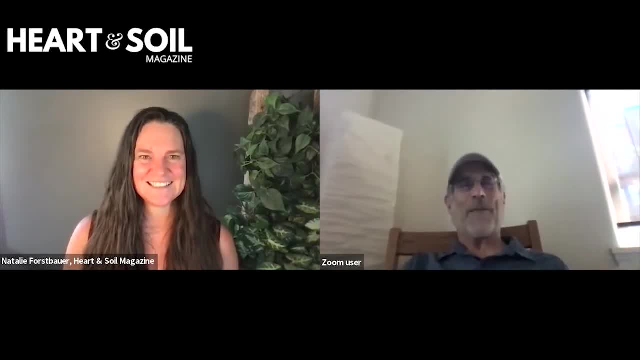 them. you walk in and you just go over that little machine and order five copies of each for the store. yeah, no, you can. you can get them almost everywhere and oddly enough, they're- they're in audible, so you can get them on audio. you can get a kindle version how they're going to do. 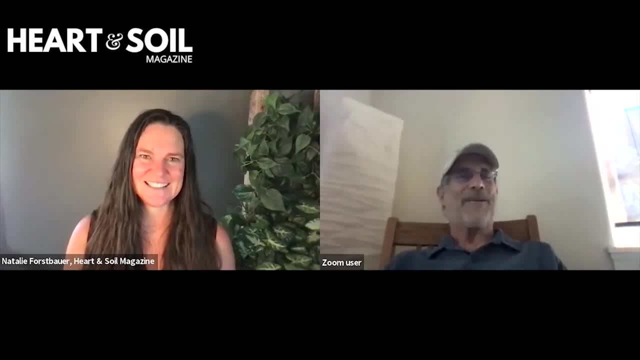 the audio of teaming with bacteria. i do not know, because they are named funnily. there are a lot of different names, a lot of long words. it's going to be very interesting to see how they do it. but the books are available. you can get them at your libraries. 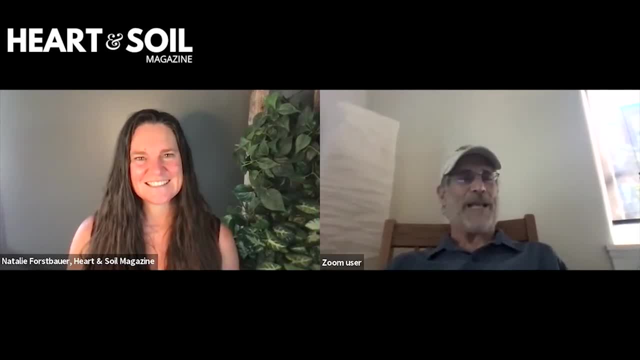 don't i? you know, i only have one rule: never lend your books to anybody. make them go out and buy their own. amen to that. it's such a resource. i- i yeah, i've gifted a few copies myself. it's one of my favorites. just it's one of my favorite places to start people with excellent, excellent, excellent. 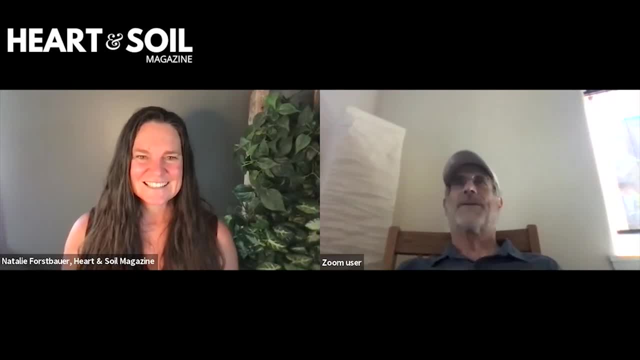 me too. yeah, and they were so much fun to write because i didn't know this stuff. you know, it's just, uh, just a journey of paying this stuff up and if, if i understand, you know, if i understand it, then i know somebody else can understand it. i'm a lawyer. i'm not. this is not my i'm not. i never took a course. 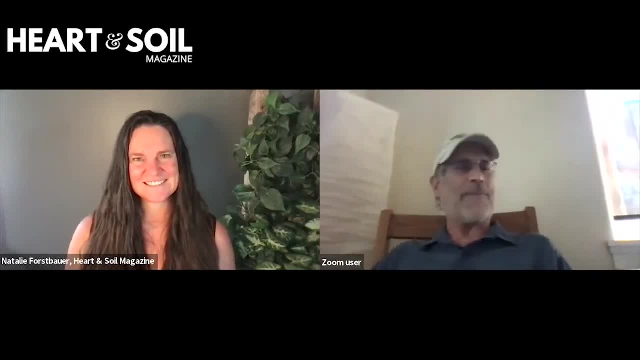 in botany, uh, and i never took a course in micro microscopy i took. i took a couple of internet stuff, but yeah, so it's just fun. it's really a lot of fun and and they're just a beginning point and i think if you read them then hopefully you know you'll hop on the internet and go to the libraries.